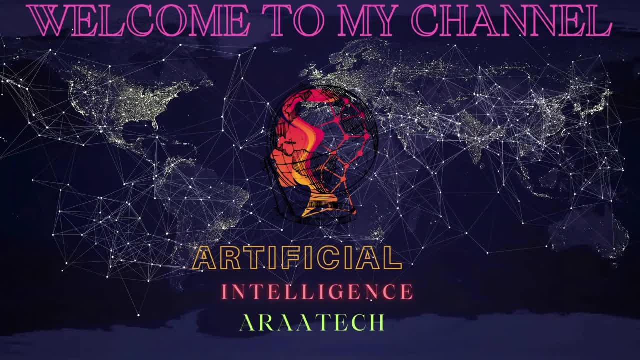 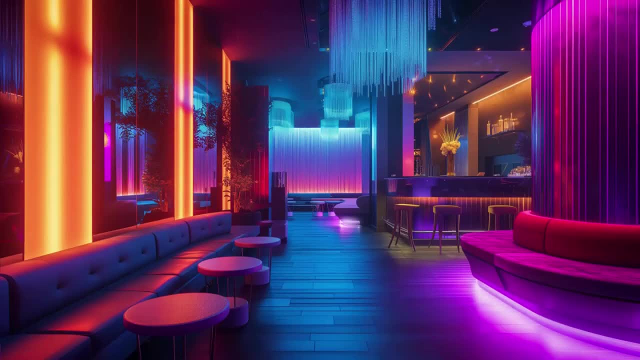 Hello viewers, as usual, presenting a new topic, Let's start. Fuzzy logic, a fascinating branch of mathematics and computer science, offers a way to deal with uncertainty in decision making. Unlike regular logic, which is all about strict true or false statements, fuzzy- 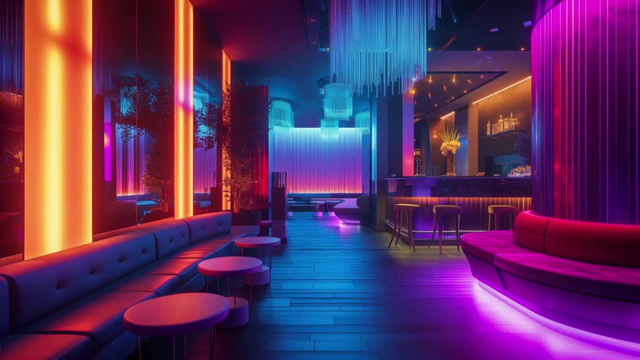 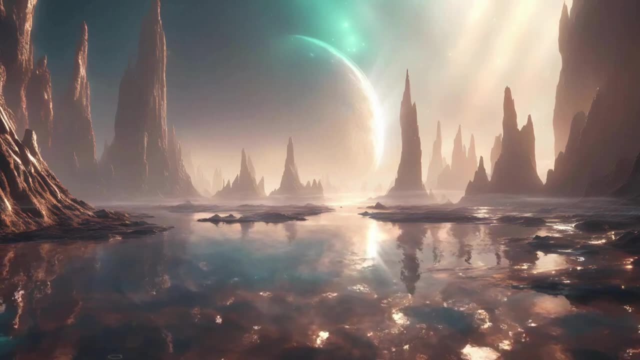 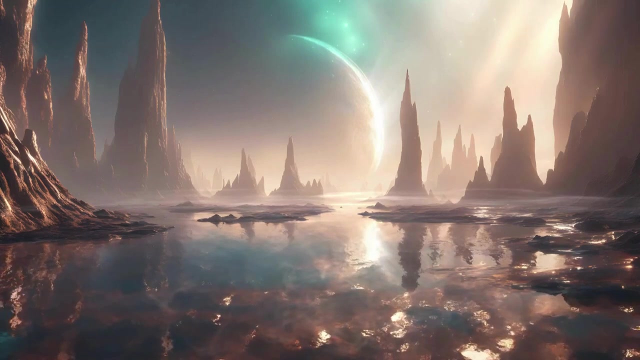 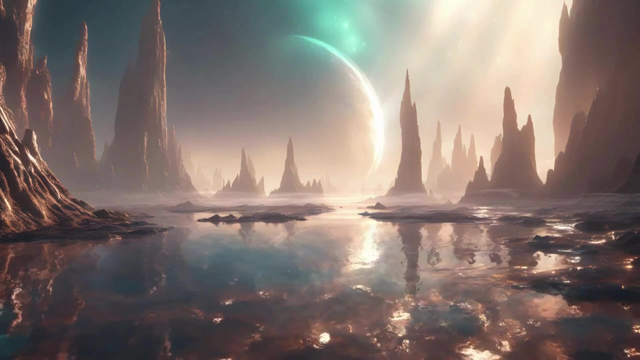 logic embraces the fuzzy in between areas of truth. It's like saying something is kind of true or mostly false, which makes it perfect for handling real world situations where things are not always clear cut. Developed by Lotfi Zadeh in the 1960s, fuzzy logic has found its way into various fields. 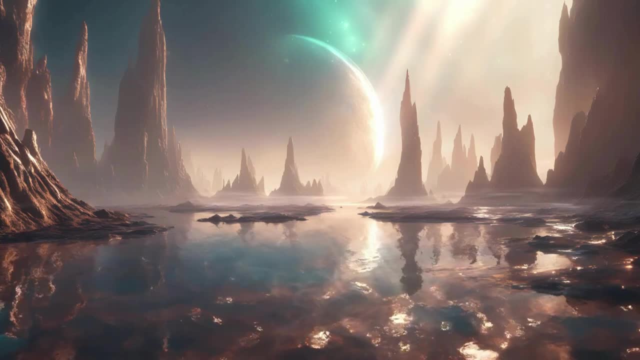 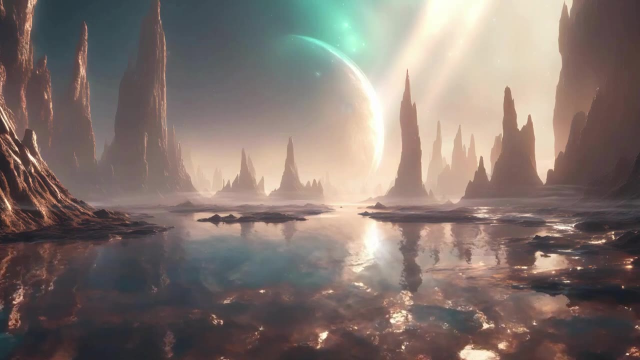 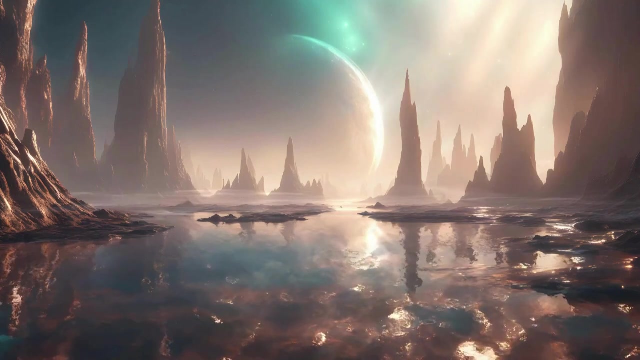 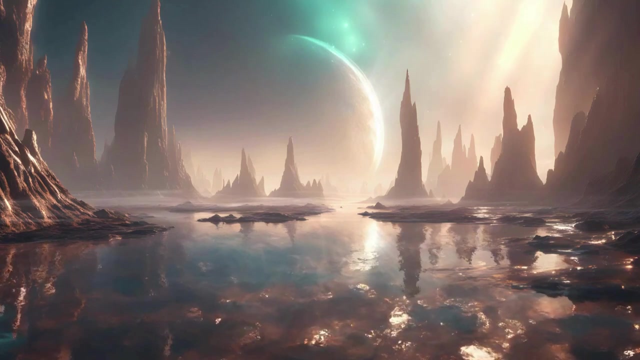 like artificial intelligence and control systems, because it can handle incomplete or ambiguous information really well. At its heart, fuzzy logic uses fuzzy sets and linguistic variables to represent vague ideas through membership functions that measure how much information belongs to a set. In this guide, we will explore fuzzy logic from the ground up, covering 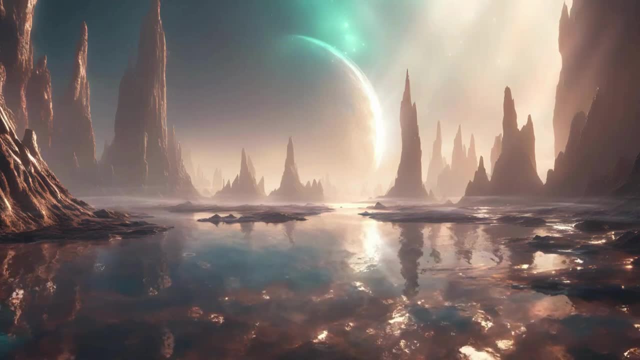 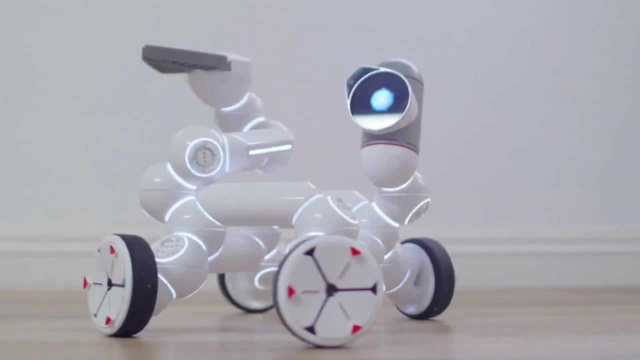 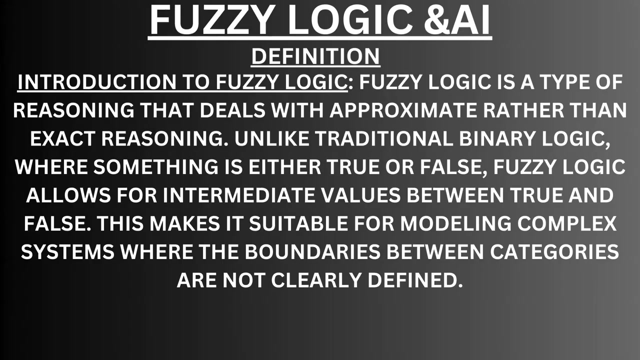 everything from basic concepts to practical applications. So, whether you are a student, engineer or researcher, you can dive into the world of fuzzy logic and discover its power in making sense of the uncertain. Fuzzy Logic and Artificial Intelligence Definition. Introduction to Fuzzy Logic. 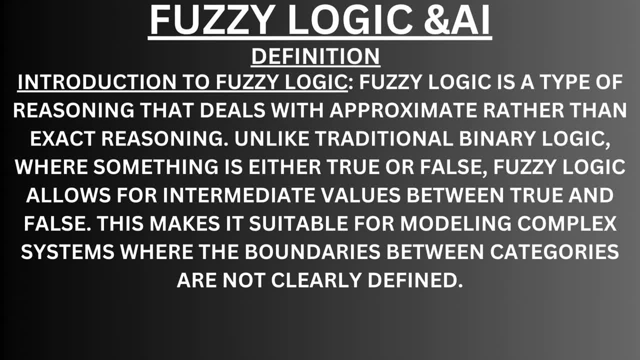 Fuzzy logic is a type of reasoning that deals with approximate rather than exact reasoning. unlike traditional binary logic, where something is either true or false, Fuzzy logic allows for intermediate values between true and false. This makes it suitable for modeling complex systems where the boundaries between categories are not clearly defined. 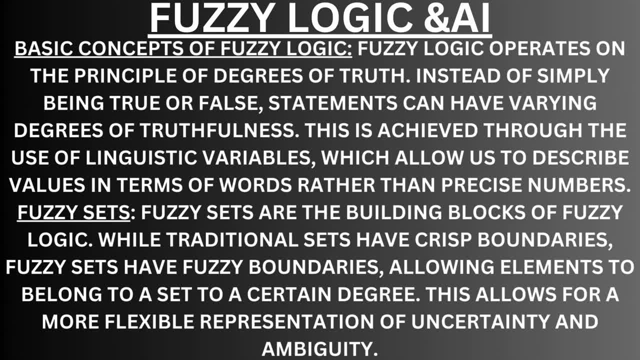 Introduction to Fuzzy Logic. Do you know the basic concepts of Fuzzy Logic? Fuzzy logic operates on the principle of the degrees of truth. Instead of simply being true or false, statements can have varying degrees of truthfulness. This is achieved through the use of linguistic variables, which allow us to describe values in terms of words. 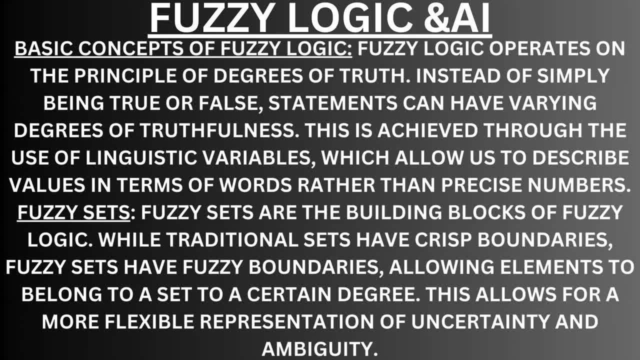 rather than precise numbers. Fuzzy Sets: Fuzzy sets are the building blocks of fuzzy logic. while traditional sets have crisp boundaries, Fuzzy sets have fuzzy boundaries allowing elements to belong to a set to a certain degree. This allows for a more flexible representation of uncertainty and ambiguity. 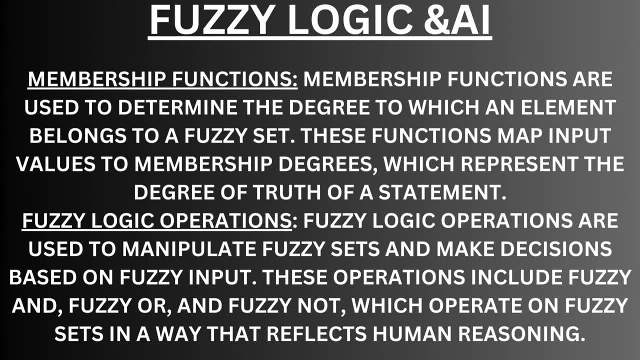 Membership functions: Membership functions are used to determine the degree to which an element belongs to a fuzzy set. These functions map input values to membership degrees, which represent the degree of truth of a statement. Fuzzy logic operations: Fuzzy logic operations are used to manipulate. 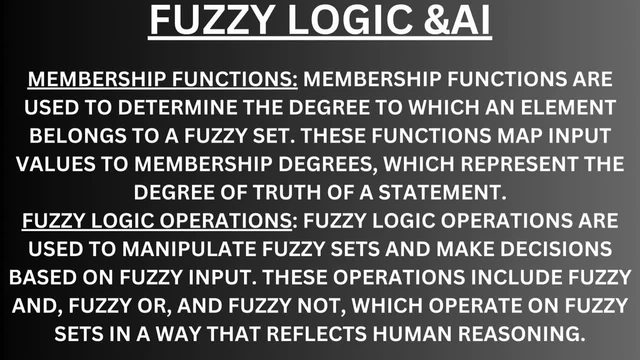 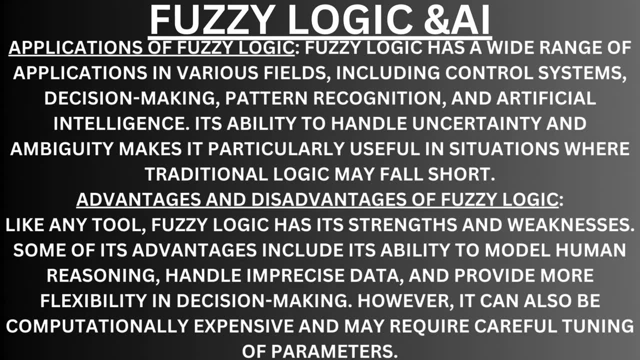 fuzzy sets and make decisions based on fuzzy input. These operations include fuzzy and fuzzyor and fuzzynot, which operate on fuzzy sets in a way that reflects human reasoning. Fuzzy logic has a wide range of applications in various fields, including control systems. 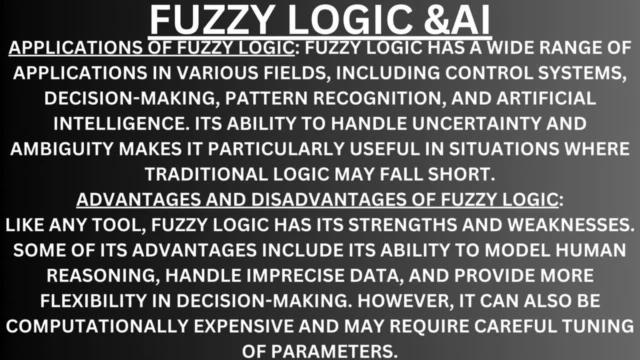 decision-making, pattern recognition and artificial intelligence. Its ability to handle uncertainty and ambiguity makes it particularly useful in situations where traditional logic may fall short. Advantages and Disadvantages of Fuzzy Logic. 1. Fuzzy Logic has its strengths and weaknesses. Some of its advantages include its ability to: 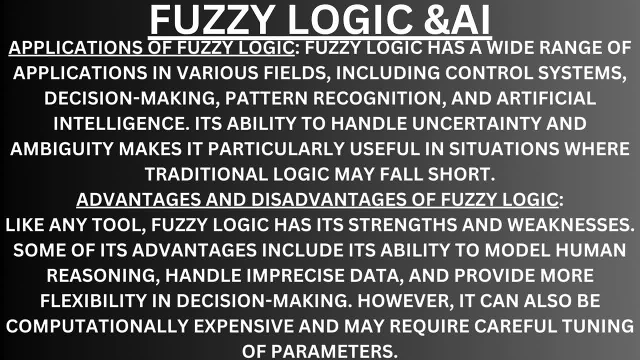 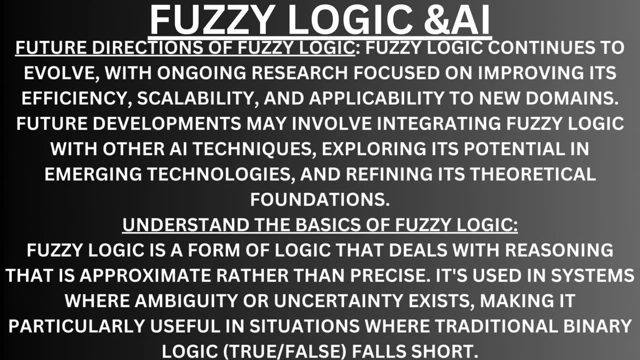 model human reasoning, handle imprecise data and provide more flexibility in decision-making. However, it can also be computationally expensive and may require careful tuning of parameters. Future Directions of Fuzzy Logic. Fuzzy Logic continues to evolve, with ongoing research focused on improving its efficiency, scalability and applicability. 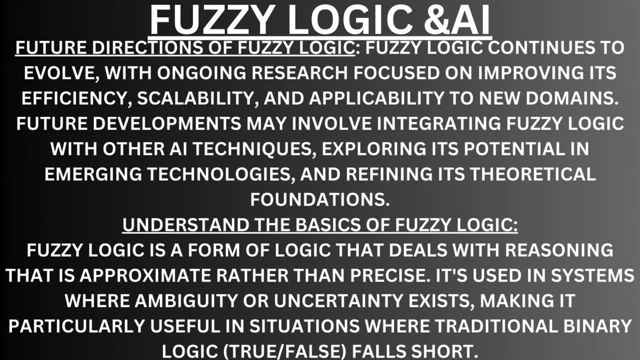 to new domains. Future developments may involve integrating fuzzy logic with other artificial intelligence techniques, exploring its potential in emerging technologies and refining its theoretical foundations. Understand the Basics of Fuzzy Logic. Fuzzy logic is a form of logic that deals with reasoning that is approximate rather than precise. It is used in systems. 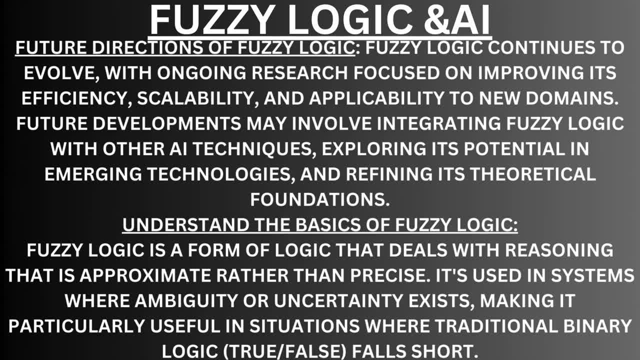 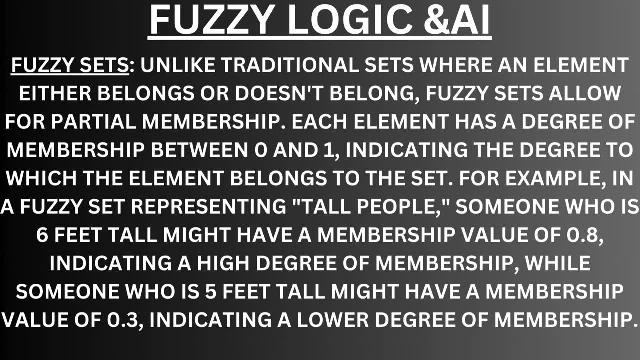 where ambiguity or uncertainty exists, making it particularly useful in situations where traditional binary logic falls short Fuzzy Sets- Unlike traditional sets, where an element either belongs or does not belong, fuzzy sets allow for partial membership. Each element has a degree of membership between 0 and 1, indicating the degree to which the element 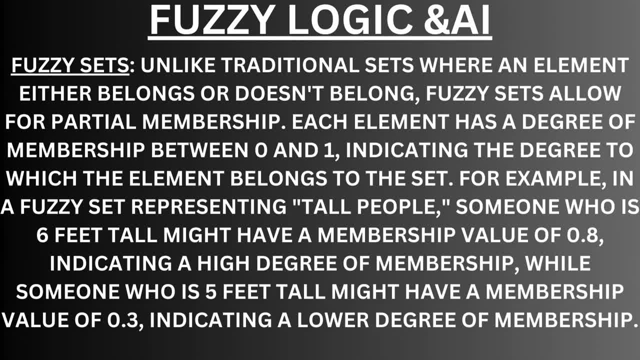 belongs to the set. For example, in a fuzzy set representing tall people, someone who is 6 feet tall might have a membership value of 0.8, indicating a high degree of membership, while someone who is 5 feet tall might have a membership. 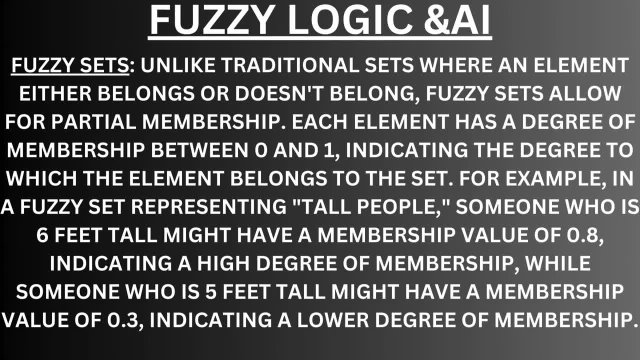 value of 0.2.. It's very sexy afterward to see that, For example, if a set of 5 feet is big, therus celebrate the Vallahiール set of Misakra of 0.3, indicating a lower degree of membership Membership functions. Membership functions. 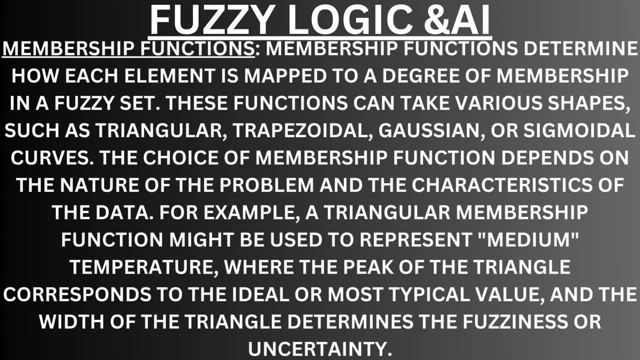 determine how each element is mapped to a degree of membership in a fuzzy set. These functions can take various shapes, such as triangular, trapezoidal, Gaussian or sigmoidal curves. The choice of membership function depends on the nature of the problem and the 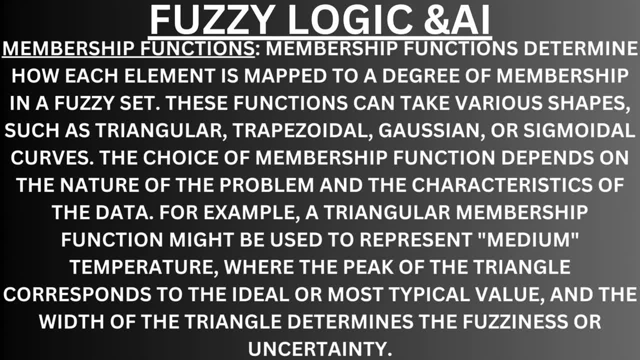 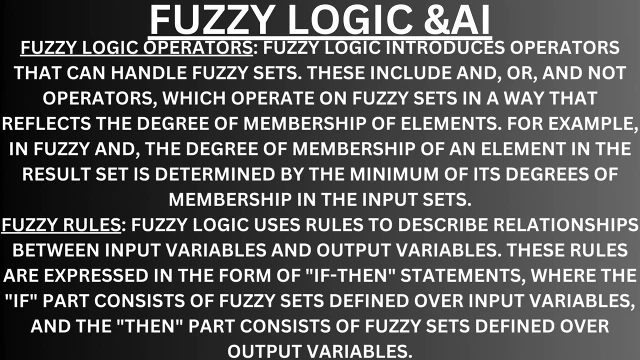 characteristics of the data. For example, a triangular membership function might be used to represent medium temperature, where the peak of the triangle corresponds to the ideal or most typical value and the width of the triangle determines the fuzziness or uncertainty. Fuzzy logic operators. Fuzzy logic introduces operators that can handle fuzzy sets. These 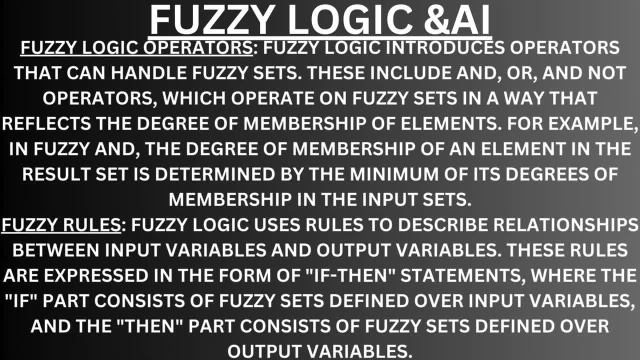 include and or and not operators which operate on fuzzy sets in a way that reflects the degree of membership of elements, For example, in fuzzy, and the degree of membership of an element in the result set is determined by the minimum of its degrees of membership. 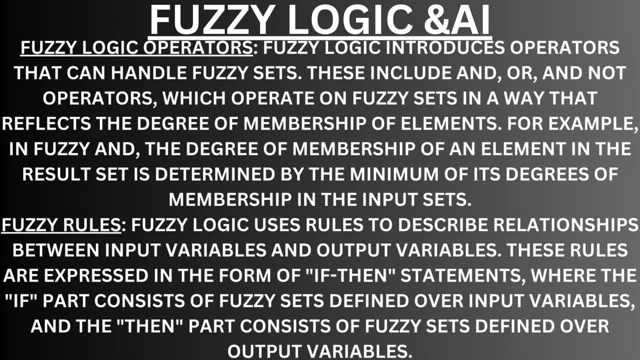 Fuzzy logic uses rules to describe relationships between input variables and output variables. these rules are expressed in the form of if than statements, where the part consists of fuzzy set defined over input variables and then part consists of fuzzy sets defined over output variables. Then the fuzzing over the input and the after heals're been confident in and not fighting. the Жjedник X6buster every so often used to say: where both marry X7 anieu Q десят. The characters D and the Z can be healed using these two statements: set neighborhood xs true When the Xs or the y 번AP are digoimited before each of the fuzzing sets. thus, results are: 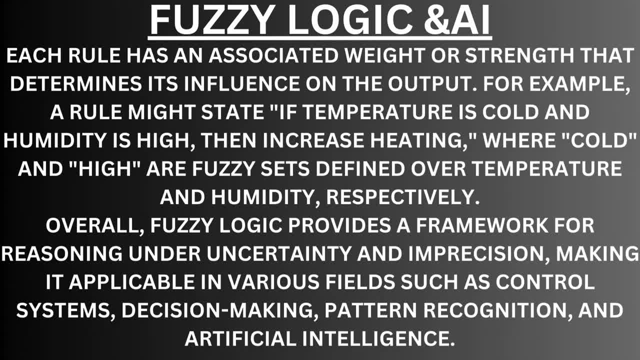 written asucht x2.. Dashing'y Crydors Vet received each term entirely true or anut leoud. at each time the set was expressed as that, it became a basic proof as to what a value based agric attackers mistakeen. Each rule has an associated weight or strength that determines its influence on the output. 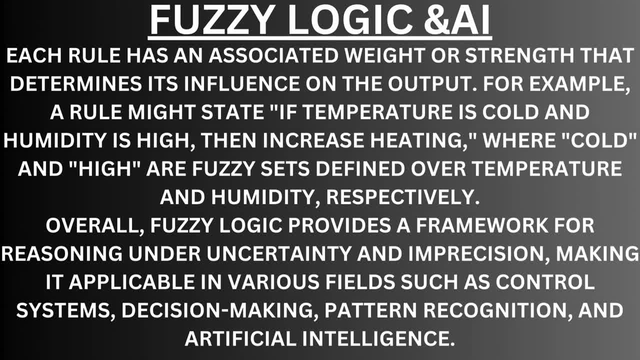 For example, a rule might state: if temperature is cold and humidity is high, then increase heating, where cold and high are fuzzy sets defined over temperature and humidity respectively. Overall, fuzzy logic provides a framework for reasoning under uncertainty and impression, making it applicable in various fields such as control systems. decision-making pattern. 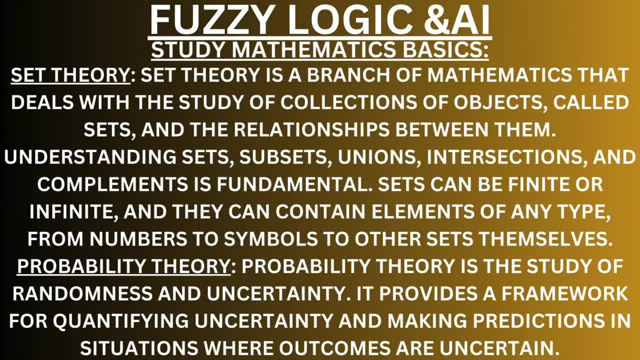 recognition and artificial intelligence Study. Mathematics Basics – Set Theory. Set theory is a branch of mathematics that deals with the study of collections of objects called sets. It provides a framework for understanding sets, subsets, unions, intersections and complements, and the relationships between them. 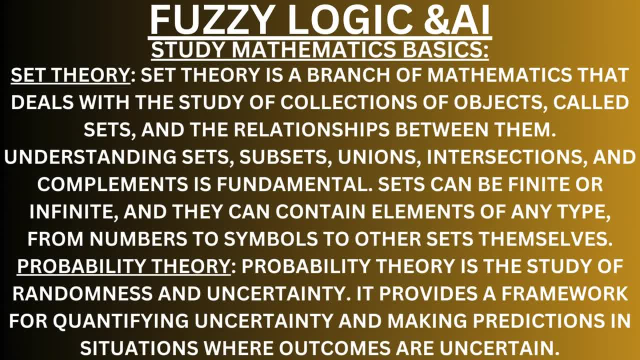 Sets can be finite or infinite and they can contain elements of any type, from numbers to symbols, to other sets themselves. Probability Theory: Probability theory is the study of randomness and uncertainty. It provides a framework for reasoning. It provides a framework for quantifying uncertainty and making predictions in situations where 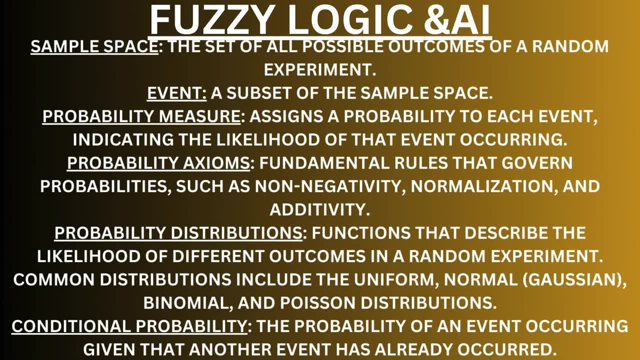 outcomes are uncertain. Sample Space – The set of all possible outcomes of a random experiment. Event – A subset of the sample space. Probability Measure – Assign a probability to each event indicating the likelihood of that event occurring. Probability Assumption – Assign a probability to each event indicating the likelihood of. 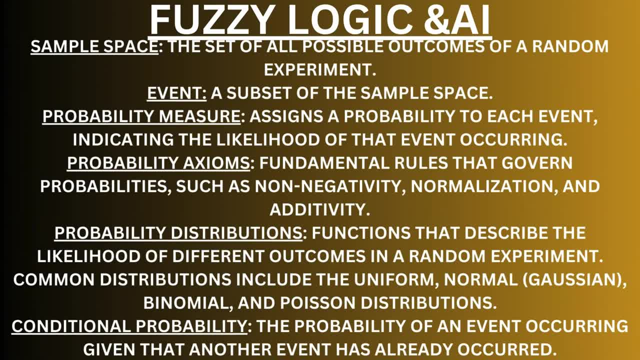 that event occurring. Event – Assign a probability to each event indicating the likelihood of that event occurring. Event – Assign a probability to your output. Event – Assign a probability to each event. Moment – Assign a probability to your output and opposite to that of an event occur in. 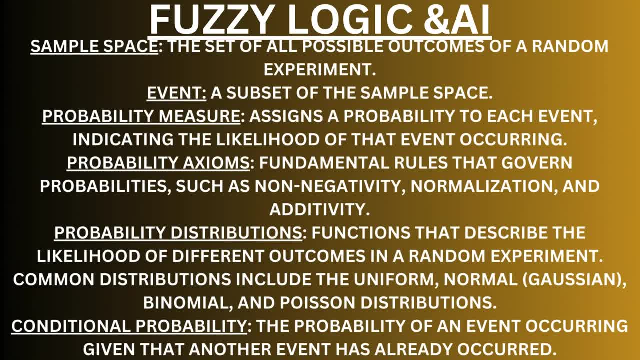 your subject group. Event – Assign a probability to the key Product. Hypothetical Introduction – A methoduben that explains possible common problems in an experiment. Common Distributions – A method of very complex charting, картian method, regular assumptions and benut Along the business of a Europe Indian experiment. 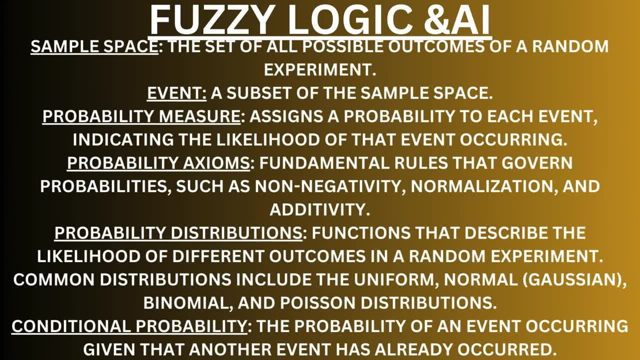 we see that speech matters- atmosphere, environments, but not the only thing. important to understand the factors, that These factors determine whether an instrument becomes brilliant or unusual. conditional probability: the probability of an event occurring given that an other event has already occurred. independence: two events are independent if the occurrence of one does not. 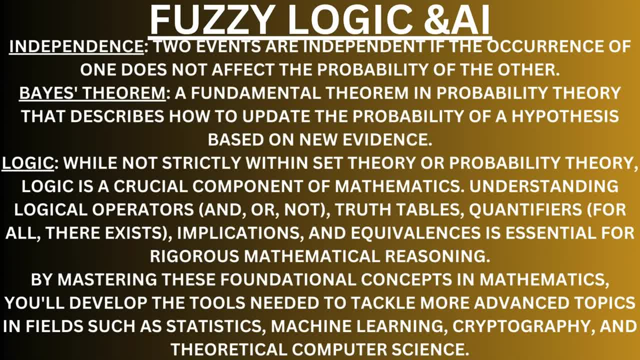 affect the probability of the other bias theorem, a fundamental theorem in probability theory that describes how to update the probability of hypothesis basis on new evidence. logic, while not strictly within set theory of probability theory, logic is a crucial component of mathematics. understanding logical operators and or not truth tables, quantifiers. 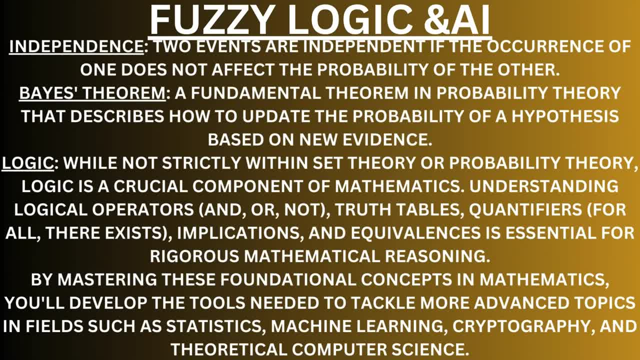 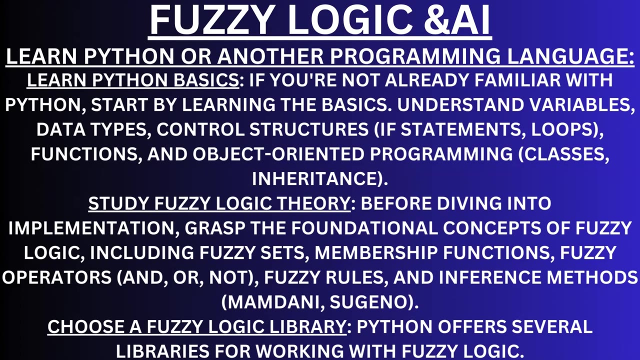 for all their exists, implications and equivalences is essential for rigorous mathematical reasoning. by mastering these foundational concepts in mathematics, you will develop the tools needed to tackle more advanced topics in fields such as statistics, machine learning, cryptography and theoretical computer science. learn python or another programming language. learn python basics if you are not already familiar with python. 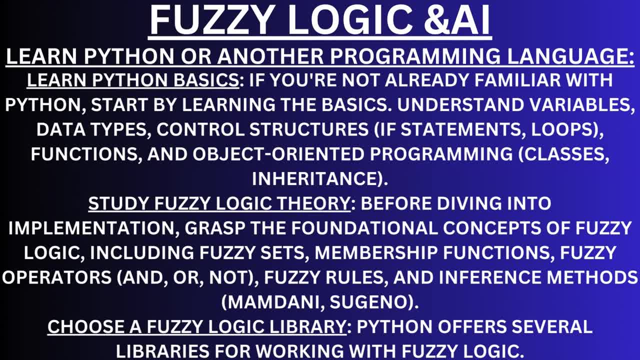 start by learning the basics: understand variables, data types, control structures, if statements, loops, functions and object-oriented programming classes. inheritance. study fuzzy logic theory before diving into implementation. grasp the foundational concepts of fuzzy logic, including fuzzy sets, membership functions, fuzzy operators and auditors, not fuzzy rules and inference methods. memdani, sugino. choose a fuzzy logic library. python offers. 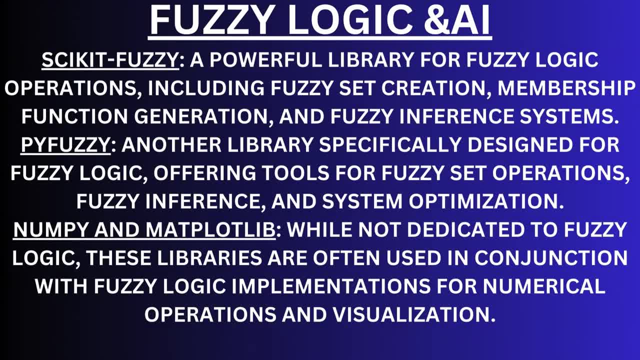 several libraries for working with fuzzy logic: scikit, fuzzy, a powerful library for fuzzy logic operations, including fuzzy set creation, membership function generation and fuzzy inference systems. py, fuzzy and other library specifically designed for fuzzy logic, offering tools for fuzzy set operations, fuzzy inference and system optimization. numpy and mat plot lib, while not dedicated to fuzzy logic. 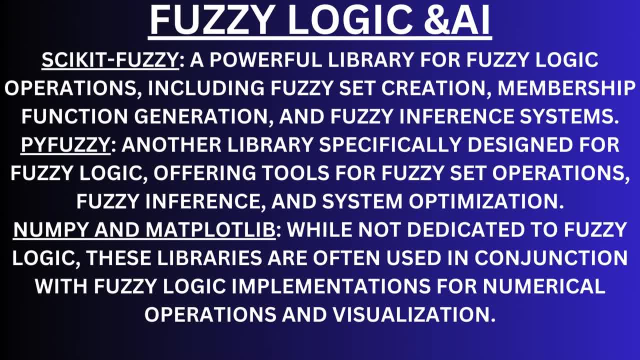 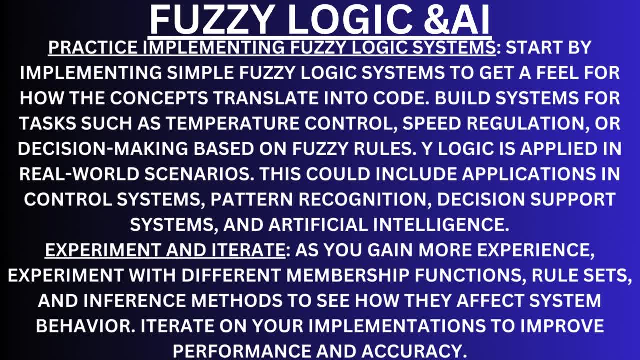 these libraries are often used in conjunction with fuzzy logic implementations for numerical operations and visualization practice implementing fuzzy logic systems. start by implementing simple logic systems to get a feel for how the concepts translate into code. build systems for tasks such as temperature control, speed regulation or decision making based on fuzzy rules. 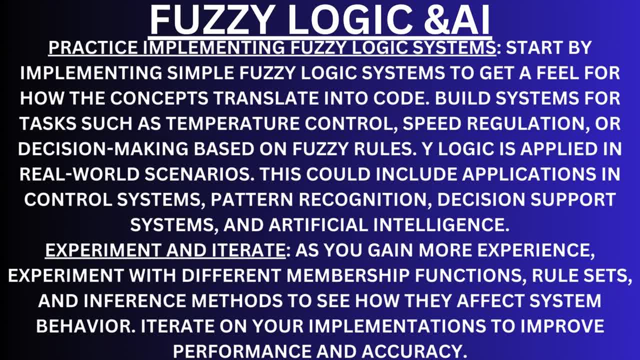 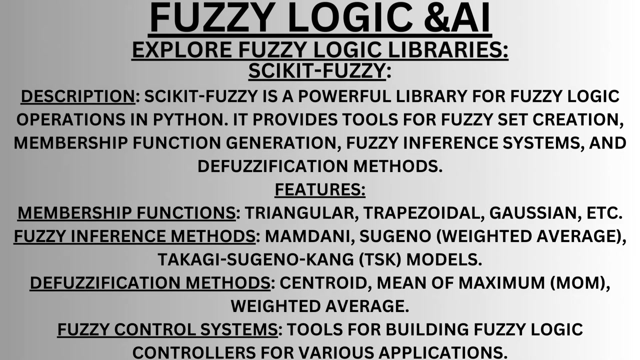 while logic is applied in real world scenarios. this could include applications in control systems, pattern recognition, decision support systems and artificial intelligence. ron architecture, coloring a map, applied artificial intelligence privileges such as the activation formula, theorer wills. whatever functions you select in your setup, you will also be able to build your own好. main operations. by the way, type your system and possible perros and frameworks that would be using this data filter information to the longer build statement so that you can talk better: cognitive and signal and learning. shared programming with system behavior. reiterate as you gain more experience. experiment with different membership functions, rule sets and inference methods to see how areas are. Thanks iterating on your implementations to improve performance and accuracy. 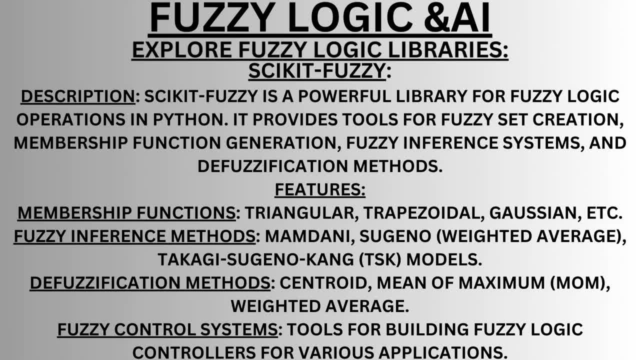 It provides tools for fuzzy set creation, membership function generation, fuzzy inference systems and diffusification methods. features: membership functions: triangular, trapezoidal, Gaussian, etc. Fuzzy inference methods: Memdani-Sugino weighted average, Takagi-Sugino-Kang TSK models. diffusification methods: centroid mean of maximum MOM weighted average. fuzzy control systems, tools for building fuzzy logic controllers for various applications. 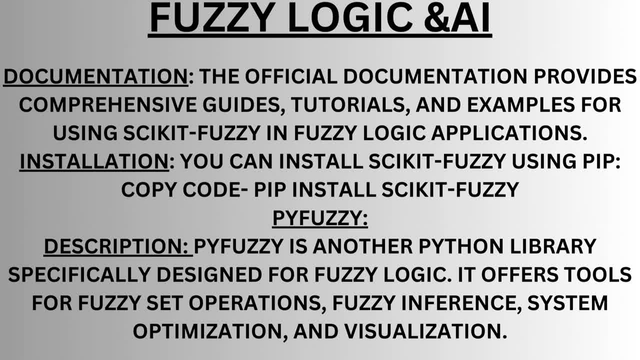 Documentation. The official documentation provides comprehensive guides, tutorials and examples for using scikit-fuzzy in fuzzy logic applications. Installation: You can install scikit-fuzzy using PIP Copy code: PIP install- scikit-fuzzy- pyfuzzy Description. pyfuzzy is another Python library specifically designed for fuzzy logic. 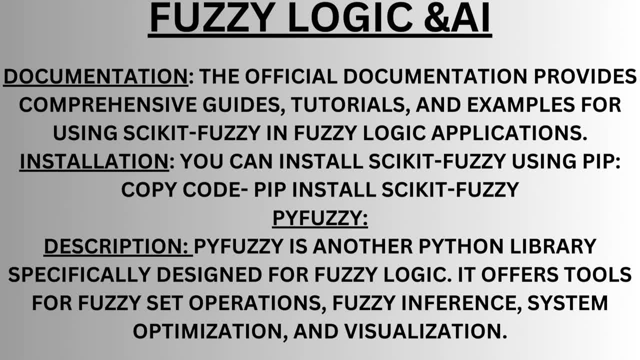 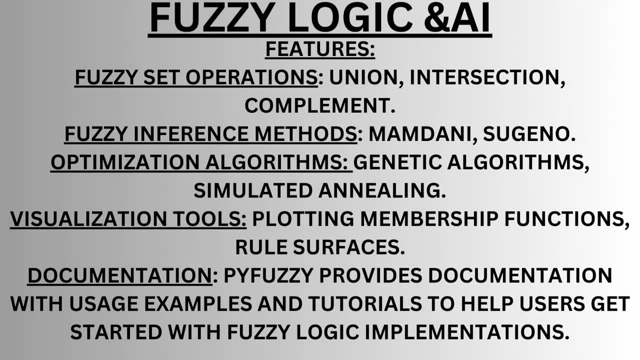 It offers tools for fuzzy set operations, fuzzy inferences, system optimization and visualization Features. Fuzzy set operations- Union intersection- complement Fuzzy inference methods, Memdani-Sugino optimization algorithms, Genetic algorithms, Simulated annealing Visualization tools, Plotting membership functions, rules, surfaces. 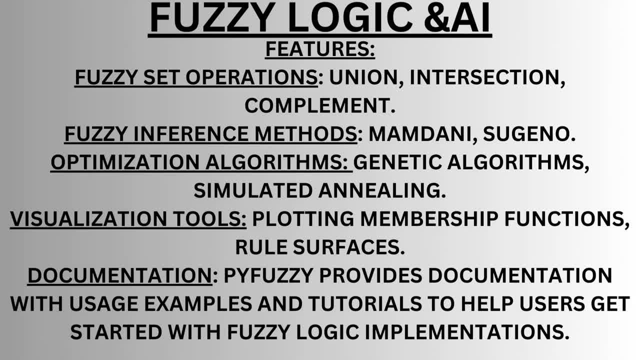 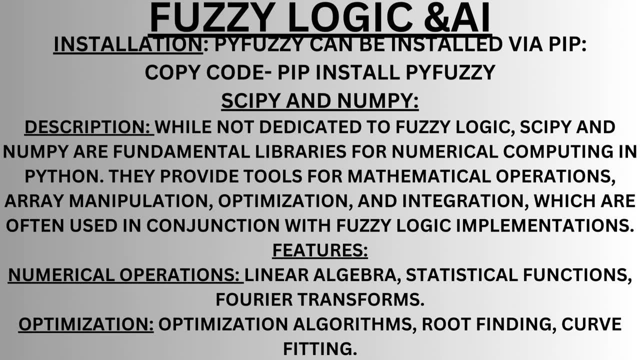 Documentation: pyfuzzy provides documentation with usage examples and tutorials. The program allows a user to access the use cases of the software Centralization subject functions only with a user's references and tutorials to help users get started with Fuzzy Logic implementations. Installation: PY Fuzzy can be installed via PIP Copy code: PIP install PY Fuzzy. 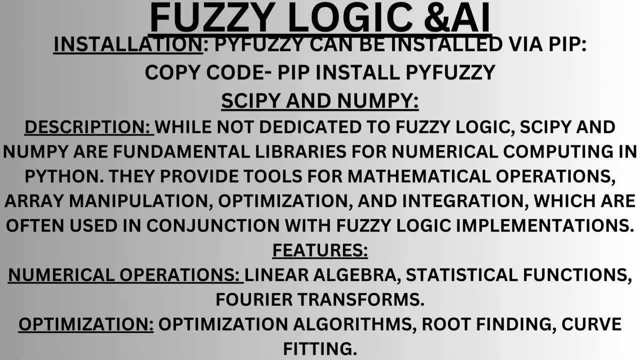 SCIPY and Numpy Description. While not dedicated to Fuzzy Logic, Skypey and Numpy are fundamental libraries for numerical computing in Python. They provide tools for mathematical operations, array, manipulation, optimization and integration, which are often used in conjunction with Fuzzy. 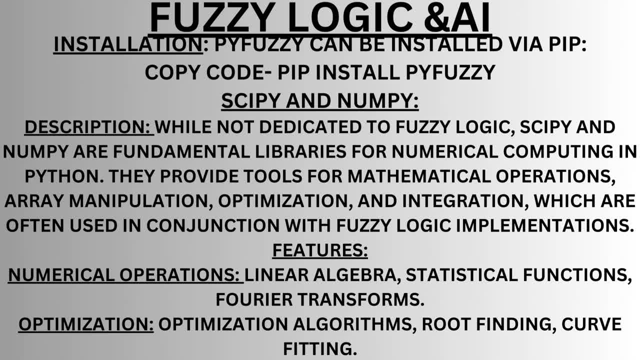 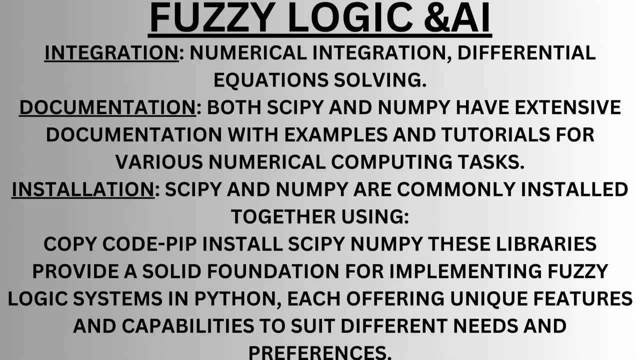 Logic implementations. Features: Numerical operations, Linear algebra, Statistical functions, Fourier transforms, Optimization, Optimization algorithms, Root finding, Curve fitting Integration, Numerical integration, differential equations solving Documentation. Both SCIPY and Numpy have extensive documentation with examples and tutorials for various numerical computing tasks. 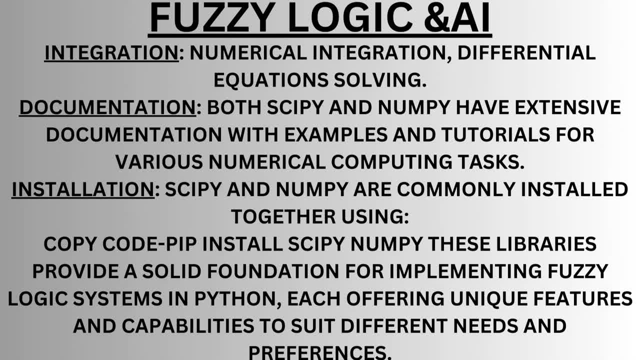 Installation: SCIPY and Numpy are commonly installed together using copy code PIP. install Skypey- Numpy. These libraries provide a solid foundation for틱an implementation of fuzzy logic systems in Pythonalled AI fala, Each offering unique features and capabilities to suit different needs and preferences. 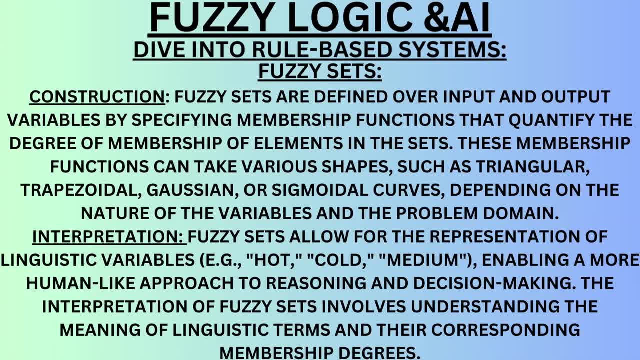 Dive into Rule-based Systems, Fuzzy Sets. Fuzzy sets are defined over input and output variables by specifying membership functions that quantify the degree of membership of elements in the set. These membership functions can take various shapes: Mengáis, shakswardsuiz, eingcha, tsaagubi, yoknde tresference valutes. 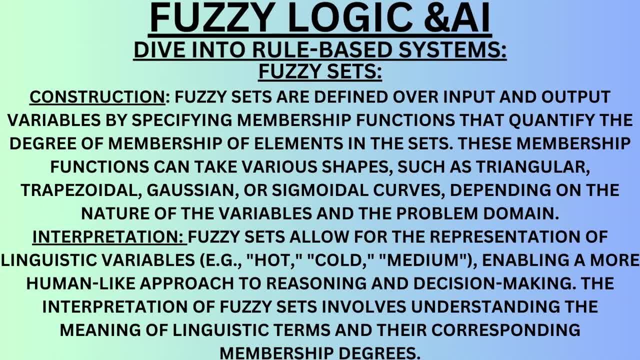 various shapes, such as triangular, trapezoidal, Gaussian and sigmoidal curves, depending on the nature of the variables and the problem domain. Interpretation. Fuzzy sets allow for the representation of linguistic variables, ie hot, cold, medium, enabling a more human-like approach to reasoning. 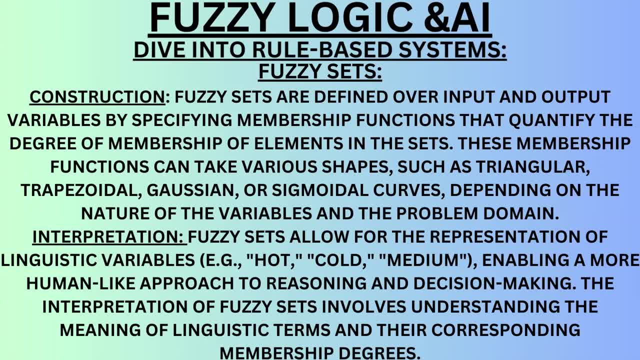 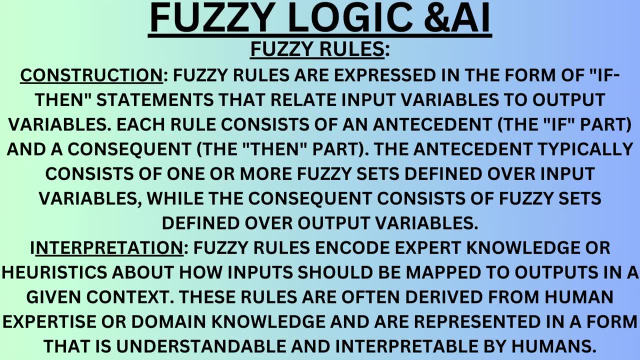 and decision-making. The interpretation of fuzzy sets involves understanding the meaning of linguistic terms and their corresponding membership degrees. Fuzzy Rules- Construction. Fuzzy rules are expressed in the form of if-then statements that relate input variables to output variables. Each rule consists of: 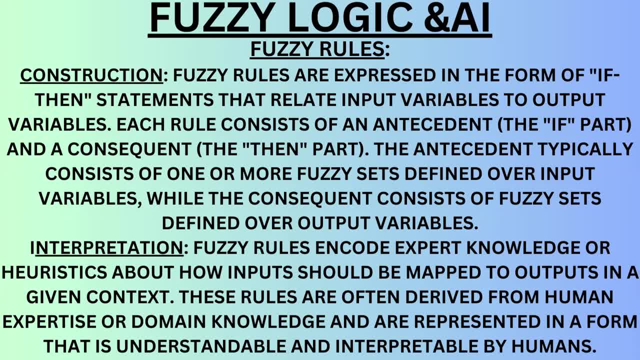 an attendant, the if part, and a consequent, the then part. The attendant typically consists of one or more fuzzy sets defined over input variables, while the consequent consists of fuzzy sets defined over output variables. Interpretation: Fuzzy rules encode expert knowledge or heuristics. 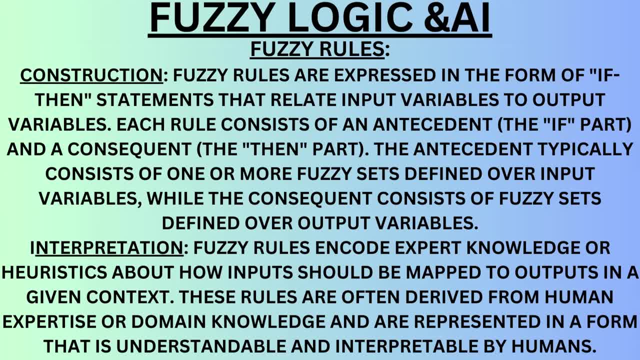 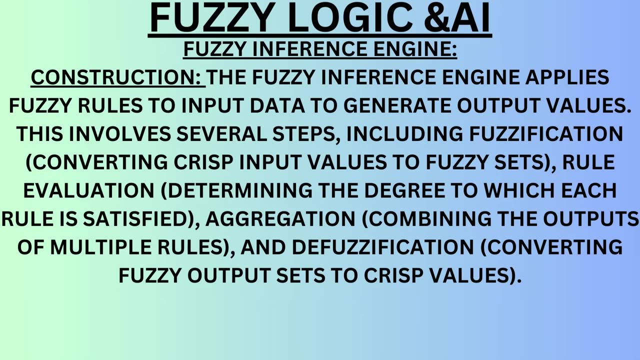 about how inputs should be mapped to outputs in a given context. These rules are often derived Interpretation. Fuzzy Inference Engine Construction. The fuzzy inference engine applies fuzzy rules to input data to generate output values. This involves several steps, including fuzzification: converting crisp input values to fuzzy sets. 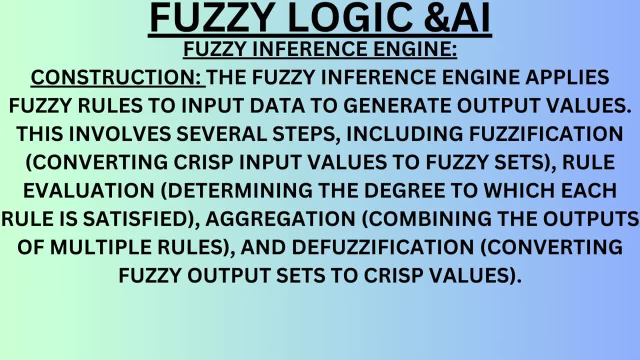 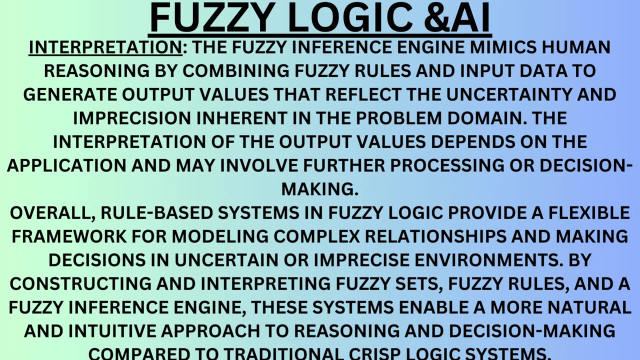 by, say, narration, simulation and detail Interpretation. The fuzzy inference engine mimics human reasoning by combining fuzzy rules and input data to generate output values that best meet the input values given to the, that reflect the uncertainty and precision inherent in the problem domain: the interpretation. 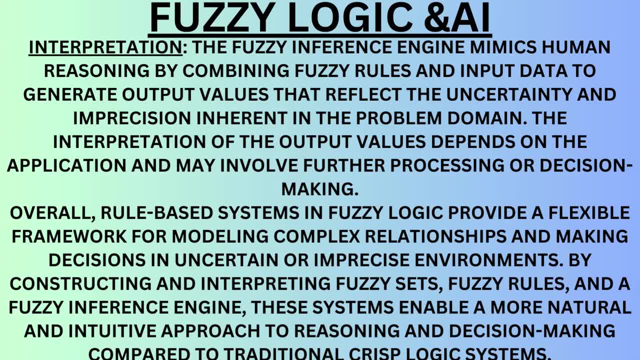 of the output values depends on the application and may involve further processing or decision making. overall rule-based systems in fuzzy logic provide a flexible framework for modeling complex relationships and making decisions in uncertain or emphasize environments. by constructing and interpreting fuzzy sets, fuzzy rules and a fuzzy inference engine, these systems enable a more 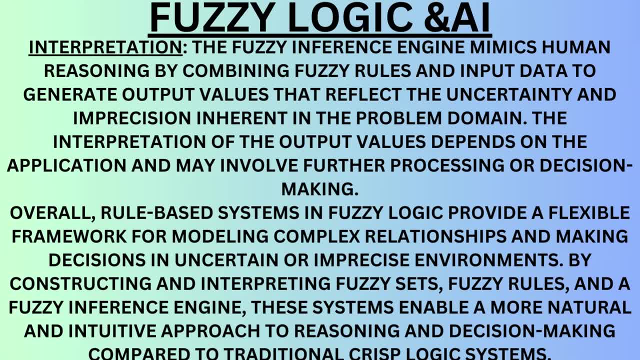 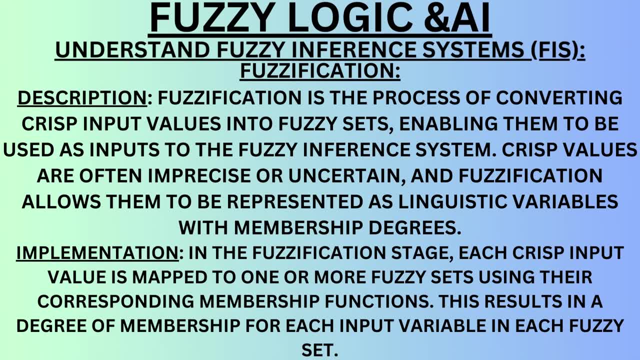 natural and intuitive approach to reasoning and decision-making compared to traditional crisp logic systems. understanding fuzzy inference system- FIS falsification description: falsification is the process of converting crisp input values into fuzzy sets, enabling them to be used as inputs to the fuzzy inference system. crisp values are often imprecise or 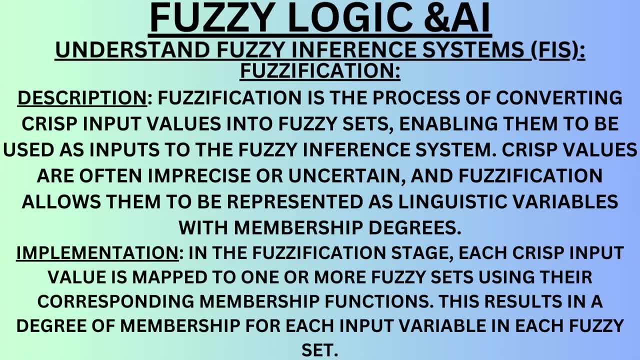 uncertain, and falsification allows them to be represented as linguistic variables with membership degrees. implementation in the falsification stage, each crisp input value is mapped to one or more of the following values. in order to be able to interpret these values using their corresponding membership functions, this results in a degree of membership for each. 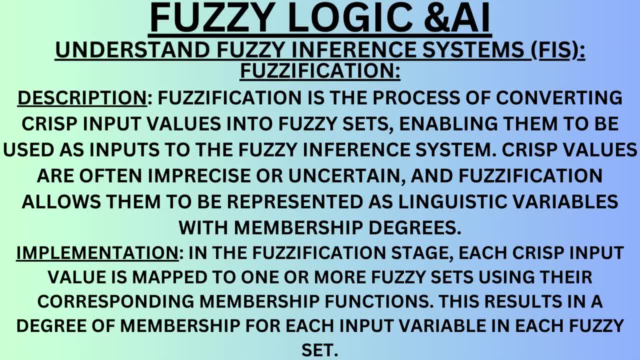 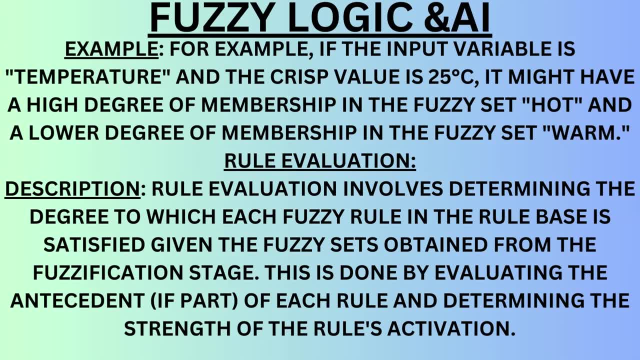 input variable in each fuzzy set example. for example, if the input variable is temperature and the crisp value is 25 centigrade, it might have a high degree of membership in the fuzzy set hot and a lower degree of membership in the fuzzy set warm rule. eventually, 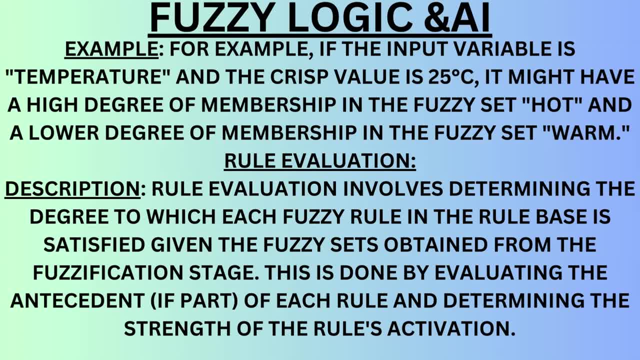 will have a higher degree of membership in the fuzzy set warm rule eventually. will have a higher degree of membership in the fuzzy set warm rule eventually. description rule evaluation involves determining the degree to which each fuzzy rule in the rule base is satisfied, given the fuzzy sets obtained from the falsification stage. this is done by: 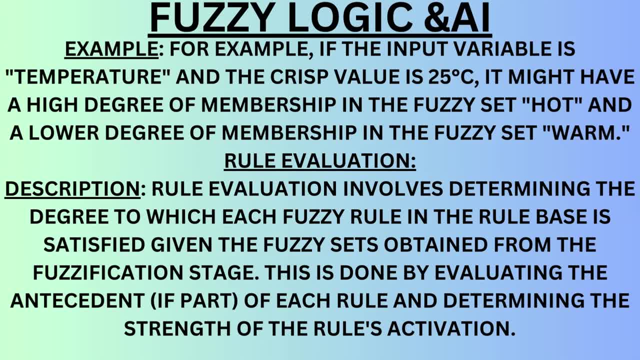 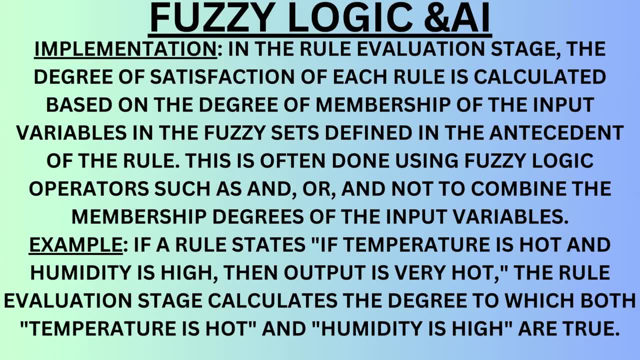 evaluating the antecedent if part of each rule and determining the strength of the rules activation implementation. in the rule evaluation stage, the degree of satisfaction of each rule is calculated based on the degree of membership of the input variables in the fuzzy sets defined in the antecedent of the rule. this is often done using 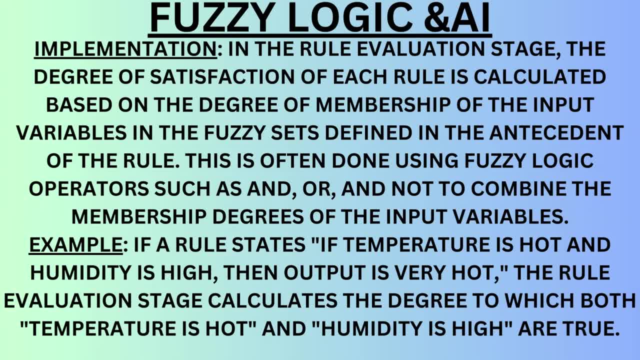 fuzzy logic operators such as and or and not to combine the membership degrees of the input variables. example: if a rule states if temperature is hot and humidity is low, the degree of membership humidity is high, then output is very hot. The rule evaluation stage calculates the degree to. 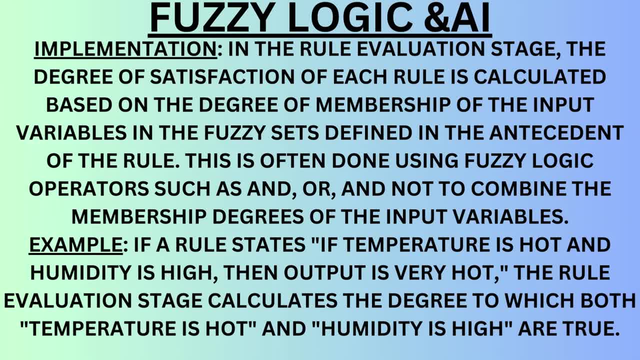 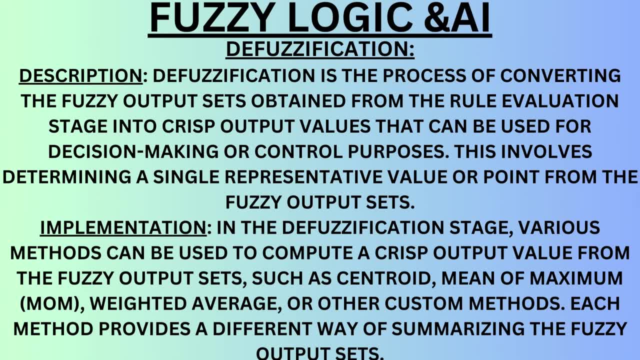 which both temperature is hot and humidity is high are true Defusification Description. Defusification is the process of converting the fuzzy output sets obtained from the rule evaluation stage into crisp output values that can be used for decision making or control purposes. This involves determining a single representative value or point from the fuzzy 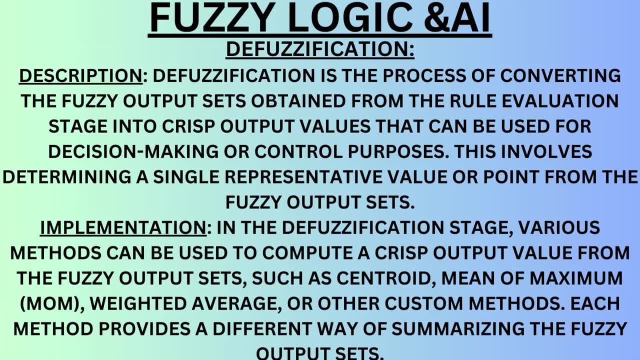 output sets: implementation In the defusification stage. various methods can be used to compute a crisp output value from the fuzzy output sets, such as centroid mean of maximum MOM weighted average or other custom methods. Each method provides a different way of summarizing the fuzzy output sets. Example: If the fuzzy output sets 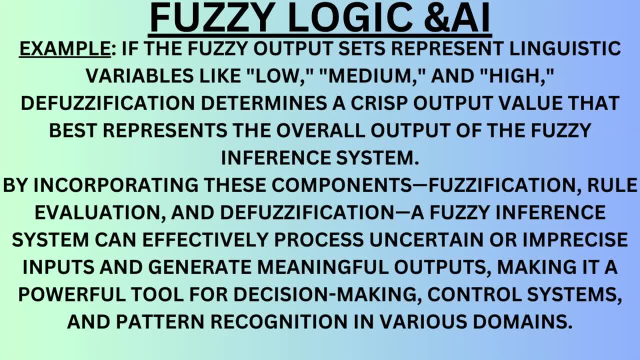 represent linguistic variables like low, medium and high. defusification determines a crisp output value that best represents the overall output of the fuzzy inference system. By incorporating these components- fusification rule, evaluation and defusification- a fuzzy inference system can effectively process uncertain or imprecise inputs and generate 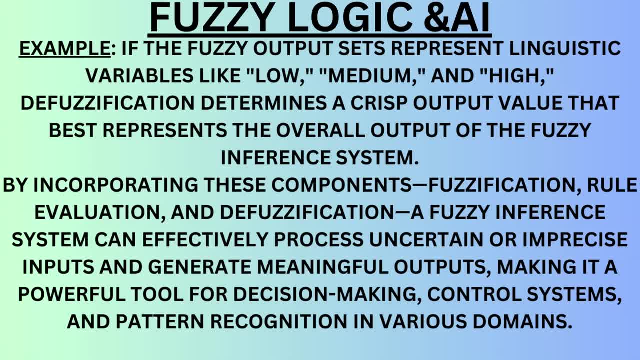 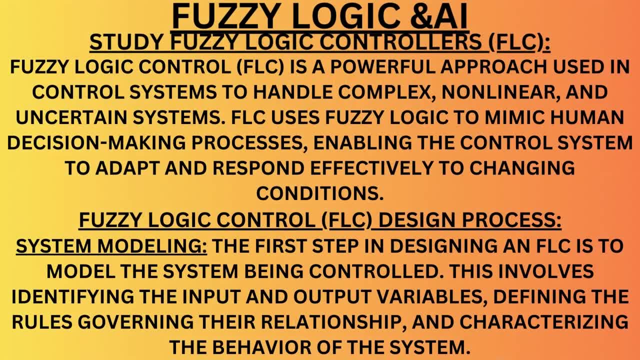 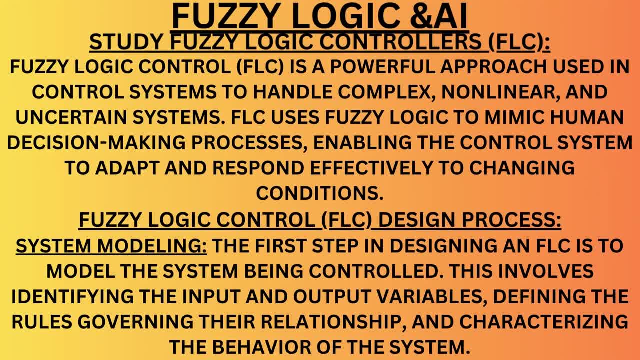 Fuzzy Logic Content turned to linear dragon. This tool uses a fusion of machine logic Power 3. F seventy four umpteen simple sub monitors and Jamaican interface. Fuzzy Logic Control F T mo entendu z 조. FPL C is a powerful approach used in control systems to 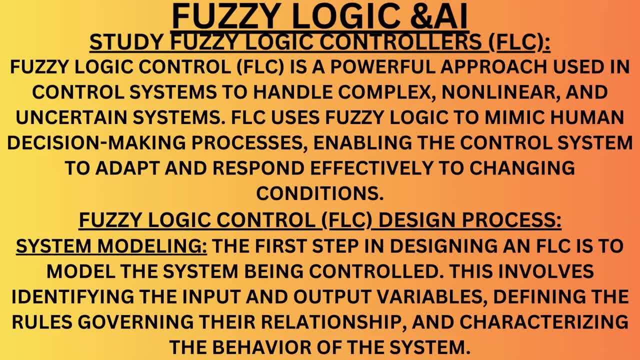 handle complex, nonlinear and uncertain systems. FLC uses fuzzy logic to mimic human decision making processes, enabling the control system to adapt and respond effectively to changing conditions. Fuzzy Logic Control- FLC Design Process System Modeling. The first step in designing an FLC is to 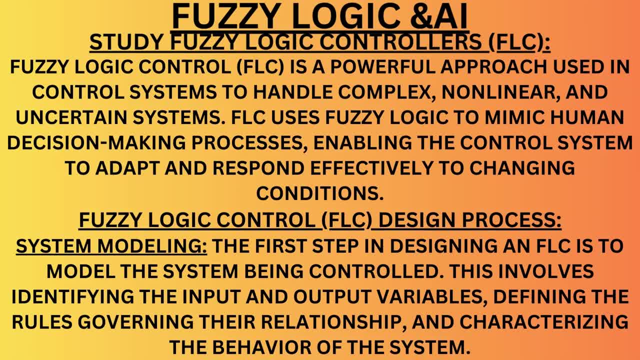 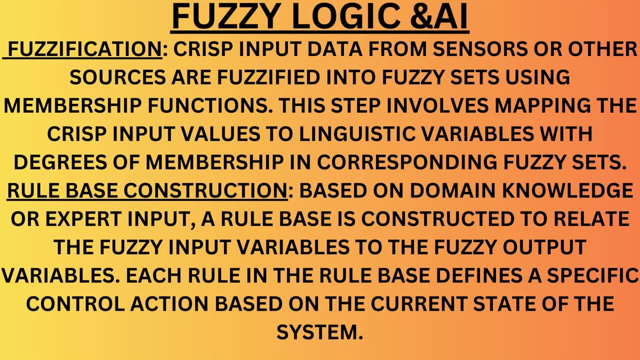 model, the system being controlled. this involves identifying the input and output variables, defining the rules governing their relationship and characterizing the behavior of the system for zification. crisp input data from sensors or other sources are falsified into fuzzy sets using membership functions. this step involves mapping the crisp input values to 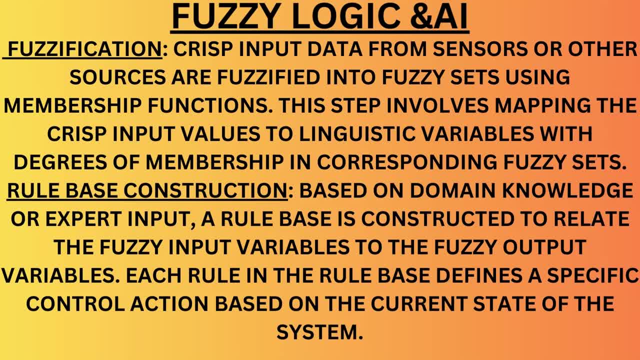 linguistic variables with degrees of membership in corresponding fuzzy sets. rule based construction based on domain knowledge or expert input. a rule base is constructed to relate the fuzzy input variables to the fuzzy output variables. each rule in the rule base defines a specific control action based on the current state of the system. rule evaluation: 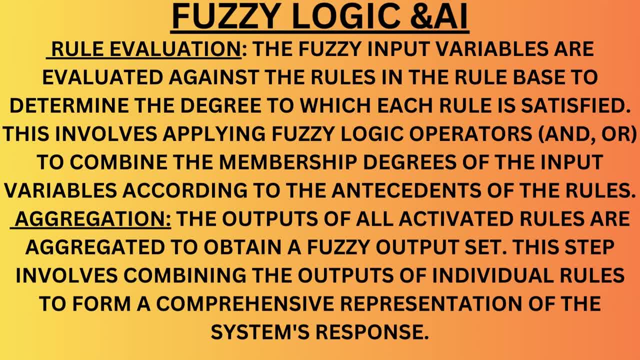 the fuzzy input variables are evaluated against the rules in the rule base to determine the degree to which each rule is satisfied. this involves applying fuzzy logic operators and or to combine the membership degrees of the input variables according to the antecedents of the rules. aggregation: the outputs. 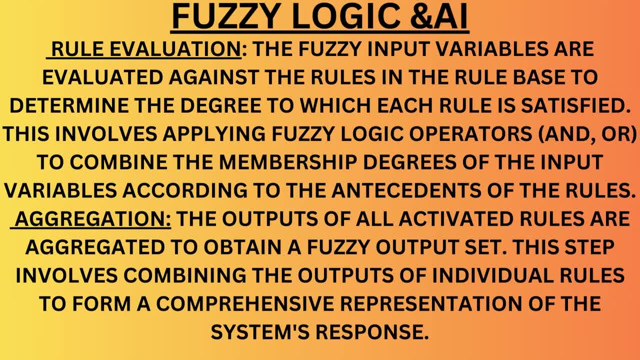 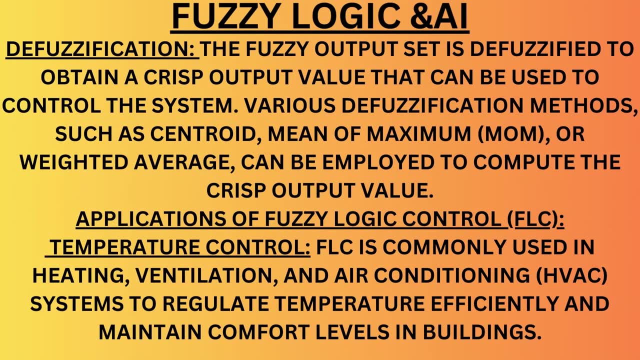 of all activated rules are aggregated to obtain a fuzzy output set. this step involves combining the outputs of individual rules to form a comprehensive representation of the system's response. defusification: the fuzzy output set is diffusified to obtain a crisp output value that can be used to control the system. various diffusification methods, such as centroid. 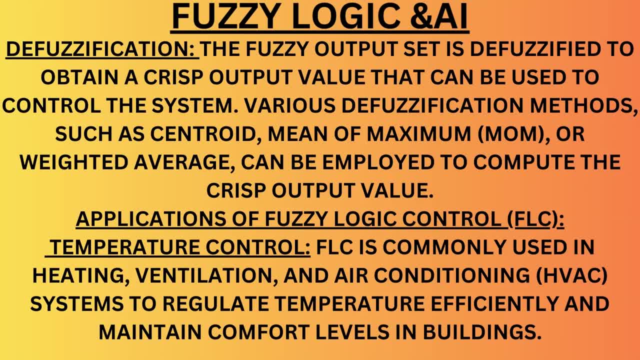 mean of maximum mom or weighted average can be employed to compute the crisp output value. applications of fuzzy logic control- flc- temperature control. flc is commonly used in heating, ventilation and air conditioning hvac systems to regulate temperature efficiently and maintain comfort levels in buildings. speed control: 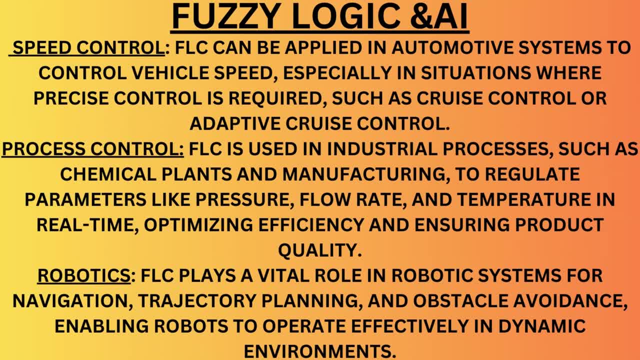 flc can be applied in automotive systems to control vehicle speed, especially in situations where precise control is required, such as cruise control or adaptive cruise control process control. flc is used in industrial processes such as chemical plants and manufacturing to regulate parameters like pressure, flow rate and temperature in real-time. 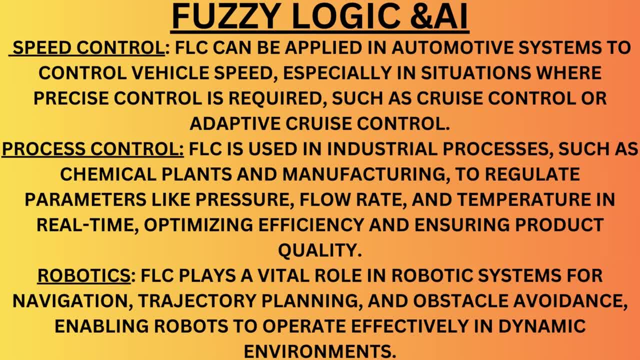 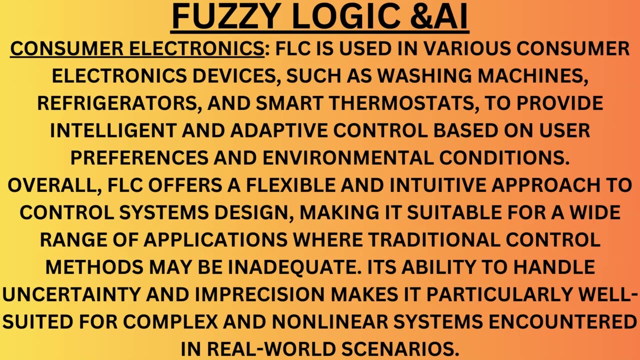 efficiency and ensuring product quality. robotics flc plays a vital role in robotic systems for navigation, trajectory planning and obstacle avoidance, enabling robots to operate effectively in dynamic environments. consumer electronics flc is used in various consumer electronics devices, such as washing machines, refrigerators and smart thermostats. 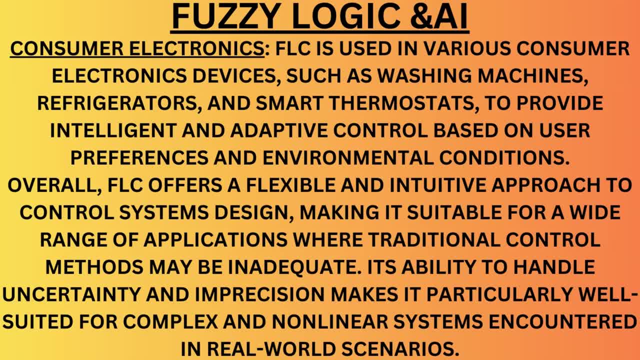 to provide intelligent and adaptive control based on user preferences and environmental conditions. overall, flc offers a flexible and intuitive approach to control systems design, making it suitable for a wide range of applications where traditional control methods may be inadequate. its ability to handle uncertainty and impression makes it particularly 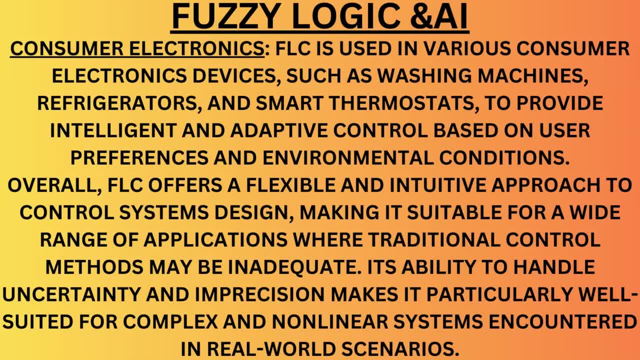 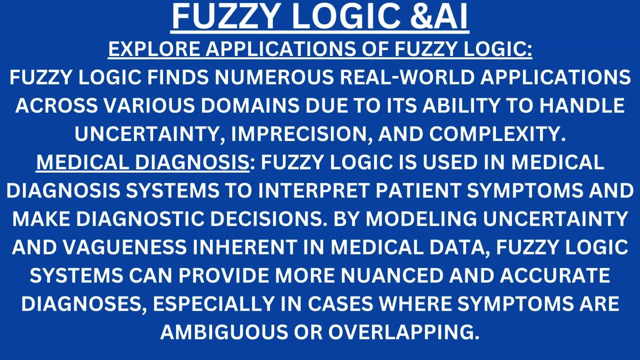 well-suited for complex and nonlinear systems encountered in real-world scenarios. Explore applications of fuzzy logic. Fuzzy logic finds numerous real-world applications across various domains due to its ability to handle uncertainty, implicit and complexity. Medical diagnosis: Fuzzy logic is used in medical diagnosis systems to interpret patient symptoms. 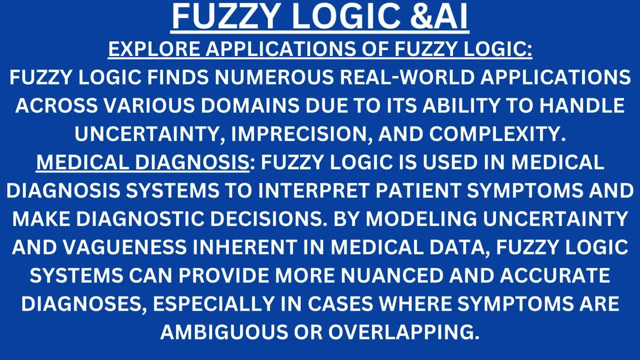 and make diagnostic decisions. by modeling uncertainty and vagueness inherent in medical data, Fuzzy logic systems can provide more nuanced and accurate diagnoses, especially in cases where symptoms are ambiguous or overlapping. Financial risk assessment: In finance, fuzzy logic is employed for risk assessment. 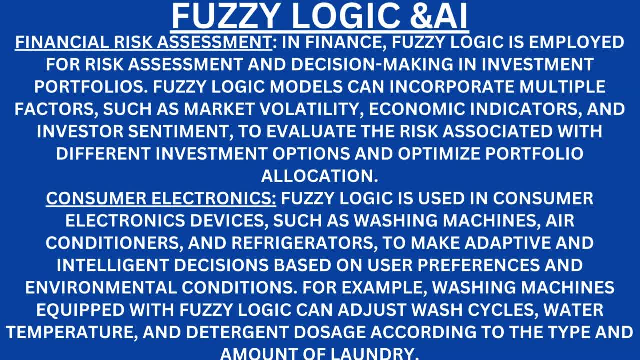 and decision-making in investment portfolios. Fuzzy logic models can incorporate multiple factors such as market volatility, economic indicators and investor sentiment to evaluate the risk associated with different investment options and optimize portfolio allocations. Consumer electronics. Fuzzy logic is used in consumer electronics devices such as washing machine, air conditioners and refrigerators. 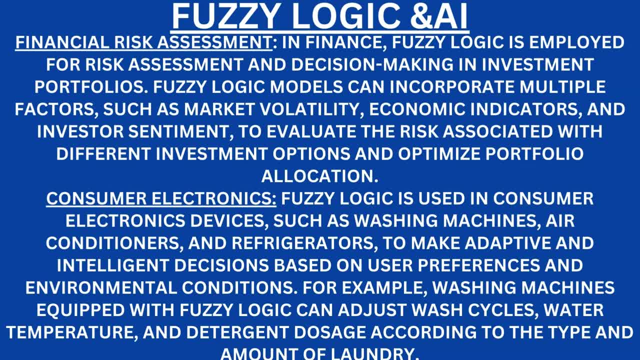 Fuzzy logic can be used to make adaptive and intelligent decisions based on user preferences and environmental conditions. For example, washing machines equipped with fuzzy logic can adjust wash cycle, water temperature and detergent dosage according to the type and amount of laundry Control systems. 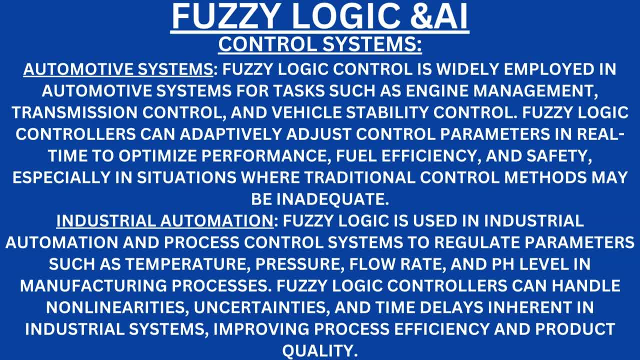 Automotive systems. Fuzzy logic control is widely employed in automotive systems for tasks such as engine management, transmission control and vehicle stability control. Fuzzy logic controllers can adaptively adjust control parameters in real time to optimize performance, fuel efficiency and safety, especially in situations where traditional control methods may be inadequate. 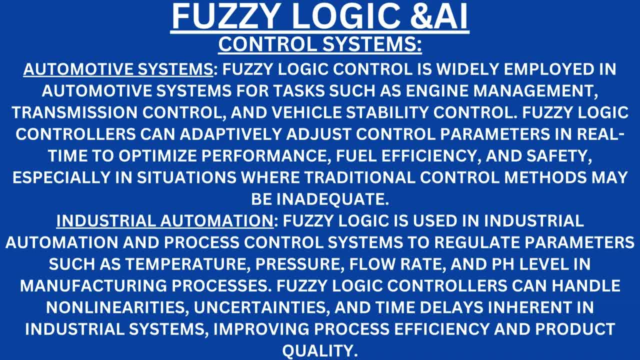 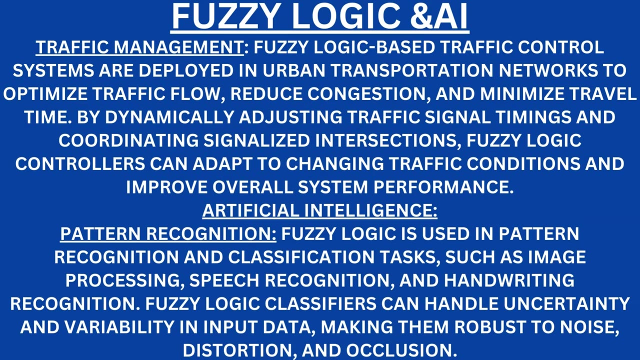 Industrial automation. Fuzzy logic is used in industrial automation and process control systems to regulate parameters such as data such as temperature, pressure, flow rate and pH level In manufacturing processes. fuzzy logic controllers can handle non-linearities, uncertainties and time delays inherent in industrial systems, improving process efficiency and product quality. 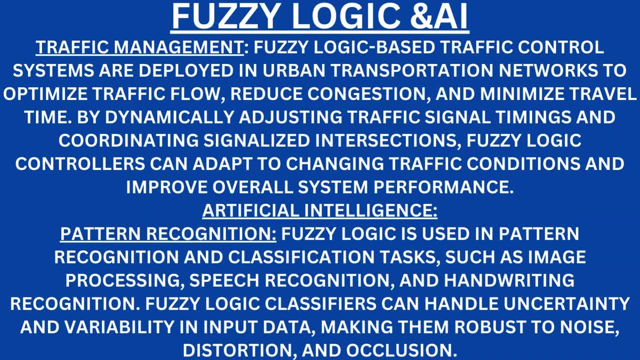 Traffic management. Fuzzy logic-based traffic control systems are deployed in urban transportation networks to optimize traffic flow, reduce congestion and minimize travel time. by dynamically adjusting traffic signal timings and coordinating signalized intersections, Fuzzy logic controllers can adapt to changing traffic conditions and improve overall system. 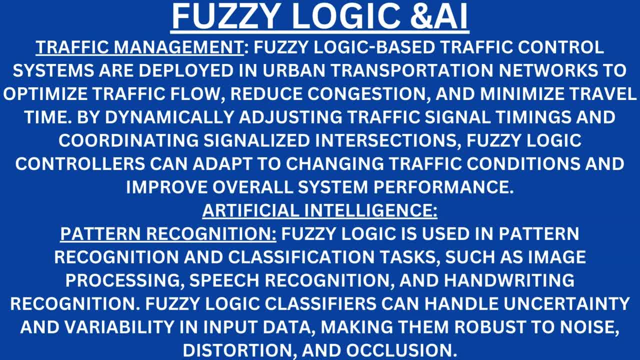 performance. Artificial intelligence, Pattern recognition, Fuzzy logic- is used in pattern recognition and classification tasks, such as image processing, speech recognition and handwriting recognition. Fuzzy logic classifiers can handle uncertainty and variability in input data, making them robust to noise distortion and occlusion. 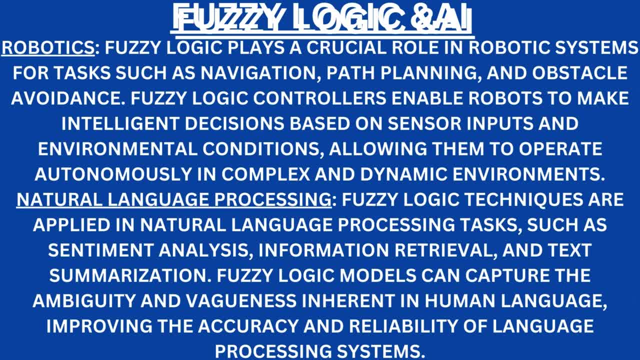 Robotics. Fuzzy logic plays a crucial role in robotics systems for tasks such as navigation, path planning and obstacle avoidance. Fuzzy logic controllers enable robots to make intelligent decisions based on sensor input and environmental conditions, allowing them to operate autonomously in complex and dynamic environments. 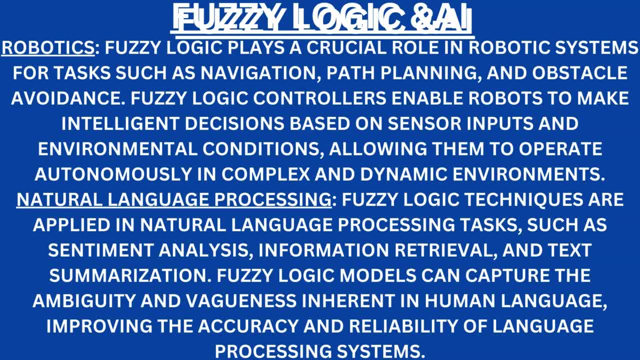 Natural language processing. Fuzzy logic techniques are applied in natural language processing tasks such as sentiment analysis, information retrieval and text summarization. Fuzzy logic models can capture the ambiguity and vagueness. Fuzzy logic models can capture the ambiguity and vagueness. 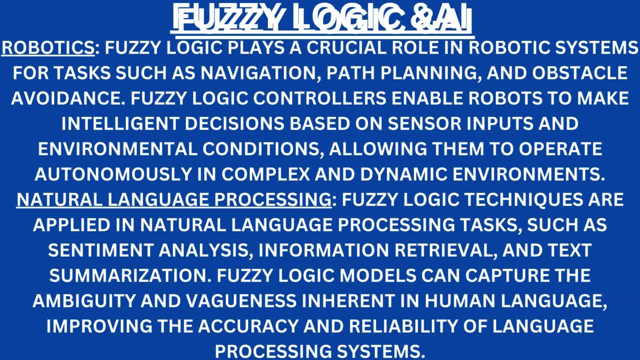 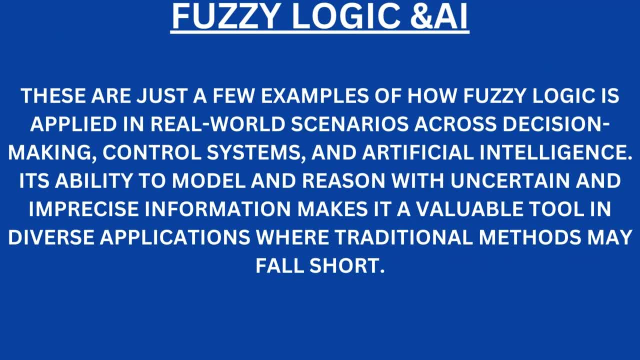 These are just a few examples of how Fuzzy logic is applied in real-world scenarios across discernment-making control systems and artificial intelligence. It's ability to model and reason with uncertain and implicit information makes it a valuable tool in diverse applications where traditional methods may fall short significantly. 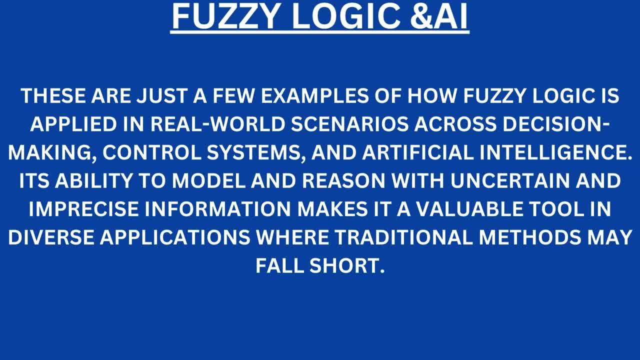 And these data and artificial intelligence programs are all sorts of dull and complex reasons to take purposes off of Fuzzy logic. These data and artificial intelligence models can be used for post- hoc experiments such as sit, Lagrangian Simulations and x-rays interactions, or dije daiixes and tables. 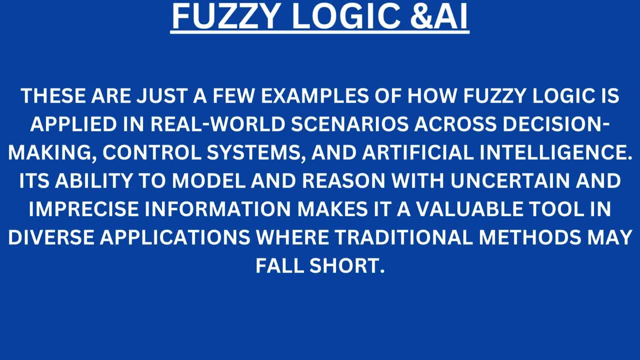 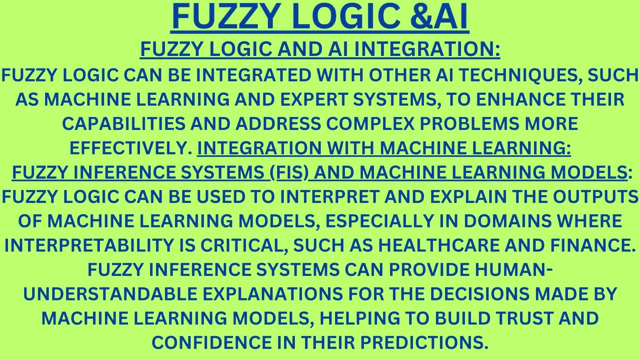 These areas of discussion createobtouve databases. to think about. chaeology's records of information being developed for early time fall short. fuzzy logic and artificial intelligence integration. fuzzy logic can be integrated with other artificial intelligence techniques, such as machine learning and expert systems, to enhance their capabilities and address complex. 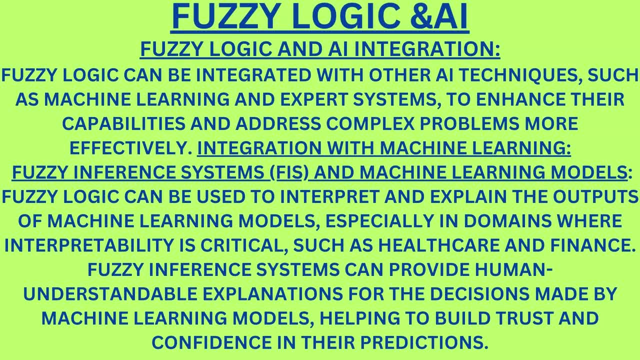 problems more effectively. integration with machine learning, fuzzy inference systems and machine learning models. fuzzy logic can be used to interpret and explain the outputs of machine learning models, especially in domains where interpretability is critical, such as healthcare and finance. fuzzy inference systems can provide human understandable explanations for the decisions made by 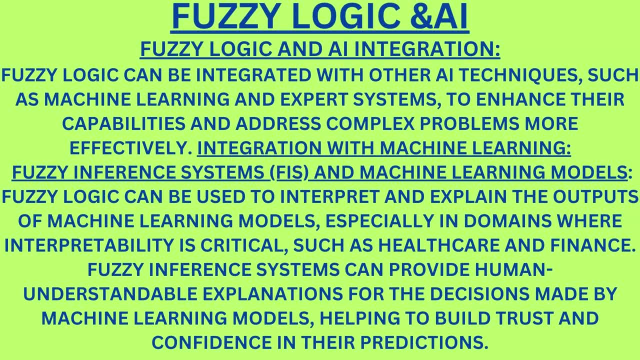 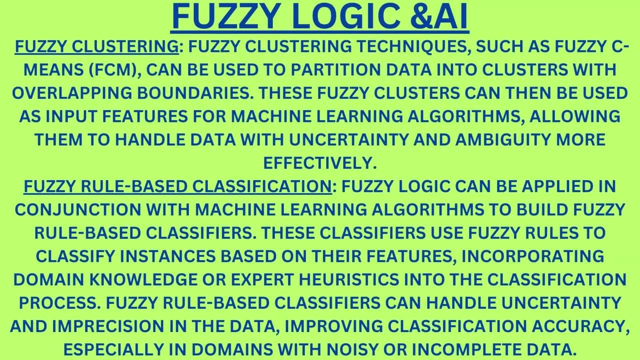 machine learning models, helping to build trust and confidence in their predictions. fuzzy clustering: fuzzy clustering techniques, such as fussy C means absolute CM, can be used to partition data into clusters with overlapping boundaries. these fuzzy clusters can then be used as input features for machine learning algorithms, allowing them to handle data with uncertainty and ambiguity more. 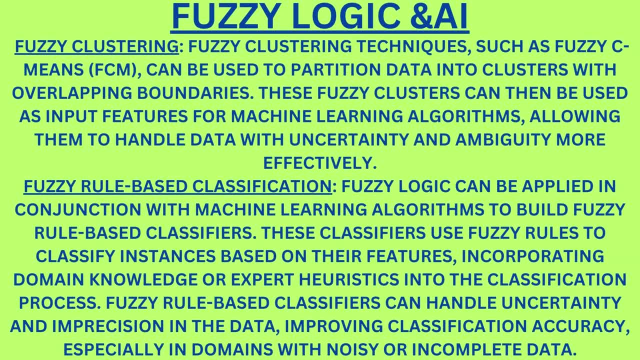 effectively. fuzzy rule-based classification. fuzzy logic can be applied in conjunction with machine learning algorithms to build fuzzy rule-based classifiers. these classifiers use fuzzy rule to classify instances based on their features, incorporating domain knowledge or expert heuristics into the classification process. fuzzy rule-based classifiers can handle uncertainty and impresion in the data, improving 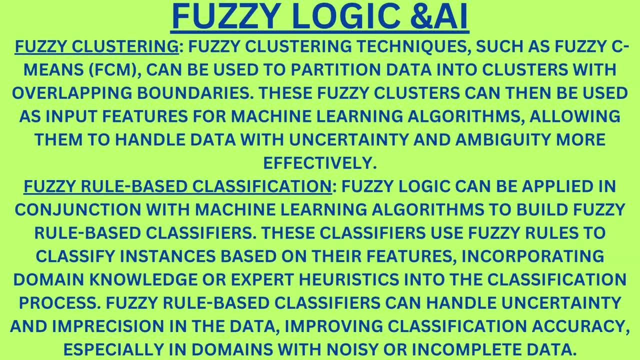 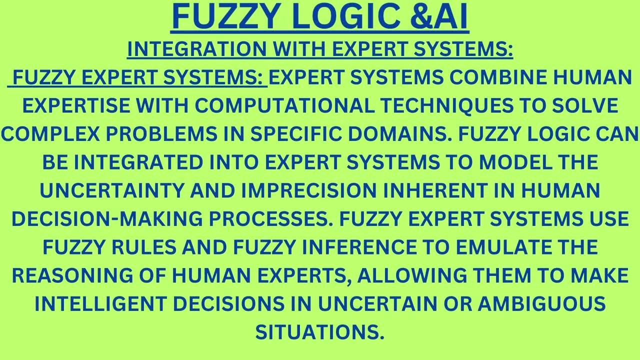 classification accuracy, especially in domains with noisy or incomplete data. integration with expert systems: fuzzy expert systems. expert system combine human expertise with computational techniques to solve complex problems in specific domains. fuzzy logic can be integrated into expert system to model the uncertainty and imprecision inherent in human decision making processes. fuzzy expert systems. 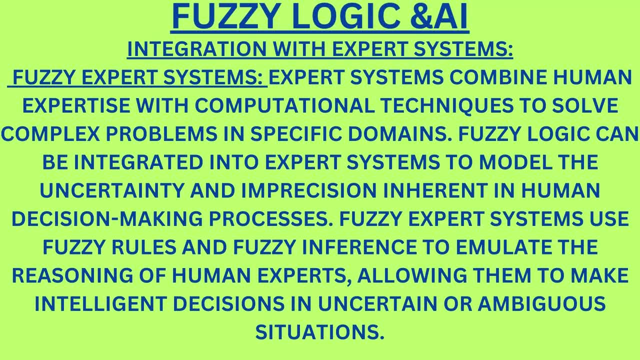 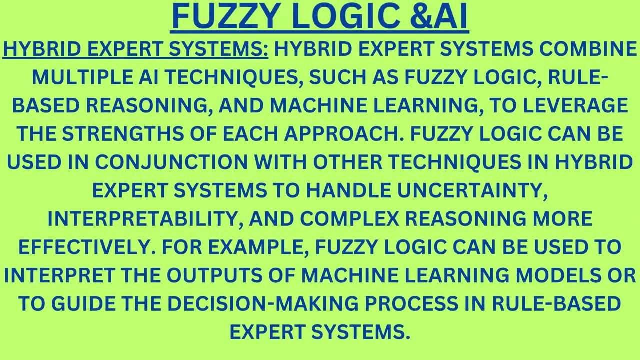 use fuzzy rules and fuzzy inference to emulate the reasoning of human experts, allowing them to make intelligent decisions in in uncertain or ambiguous situations. hybrid export systems: hybrid export systems combine multiple artificial intelligence techniques, such as fuzzy logic, rule-based reasoning and machine learning, to leverage the strengths of each approach. fuzzy: 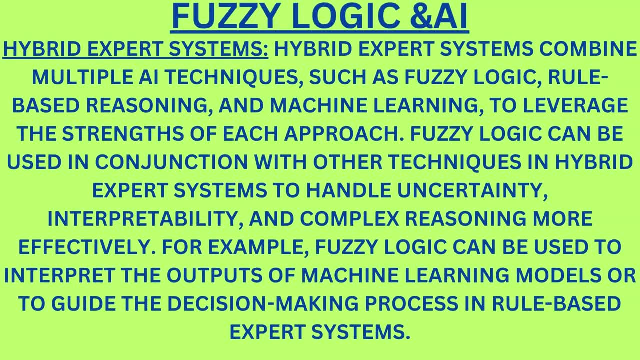 logic can be used in conjunction with other techniques in hybrid expert systems to handle uncertainty, interpretability and control of the data in the future complex reasoning more effectively. for example, fuzzy logic can be used to interpret the outputs of machine learning models or to guide the decision-making process in rule-based 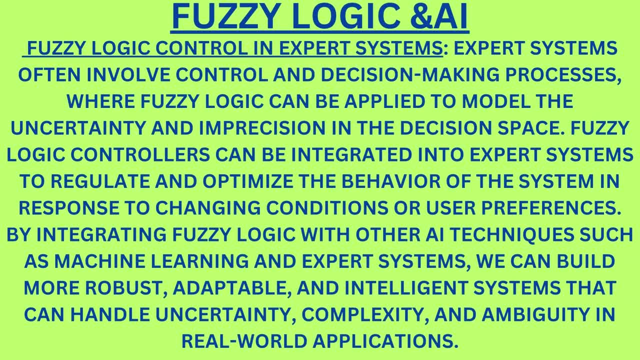 expert systems. fuzzy logic control in expert systems. expert systems often involve control and decision-making processes where fuzzy logic can be applied to model the uncertainty and impression in the decision space. fuzzy logic can be integrated into expert systems to regulate and optimize the behavior of the system in response to changing conditions or user preferences by integrating fuzzy logic with other. 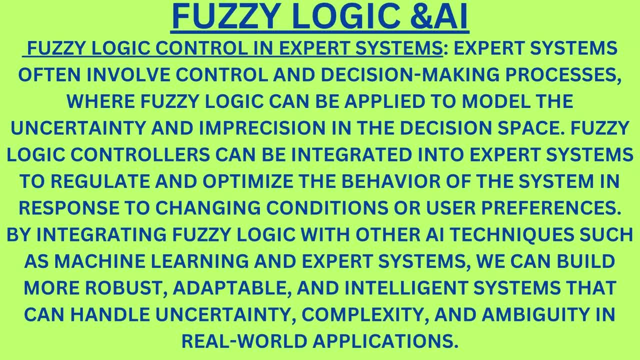 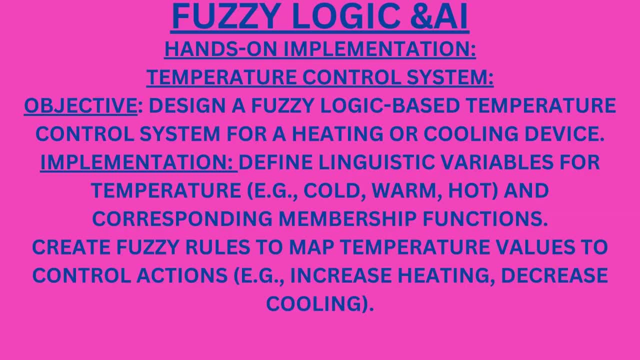 artificial intelligence techniques such as machine learning and expert systems, we can build more robust, adaptable and intelligent systems that can handle uncertainty, complexity and ambiguity in real-world applications. hands-on implementation. temperature control system: objective design: a fuzzy logic based temperature control system for a heating or cooling device implementation. 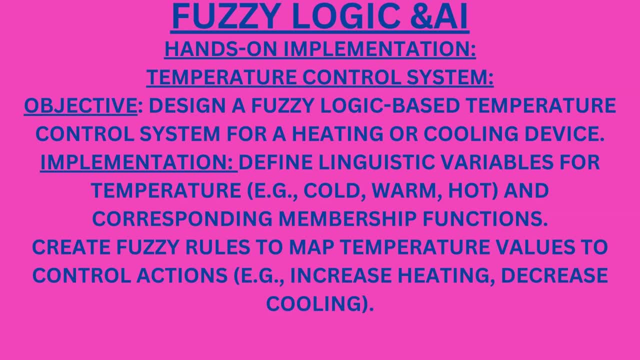 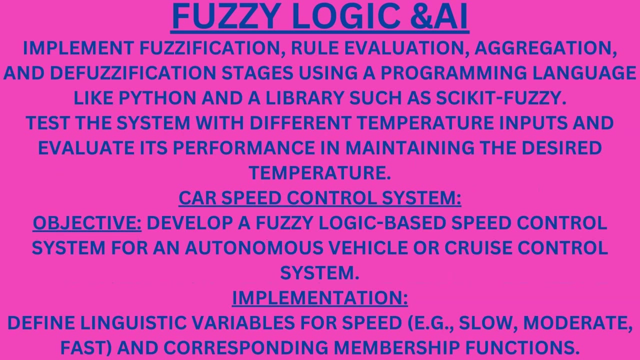 define linguistic variables for temperature- that is, cold, warm, hot, and corresponding membership functions. create fuzzy rules to map temperature values. to control actions, that is, increase heating degrees, cooling. select temperature and temps. to adjustheart temperature rise and excess heat temperature and temperature increase cooling. implement fuzzification rule evaluation evaluation. 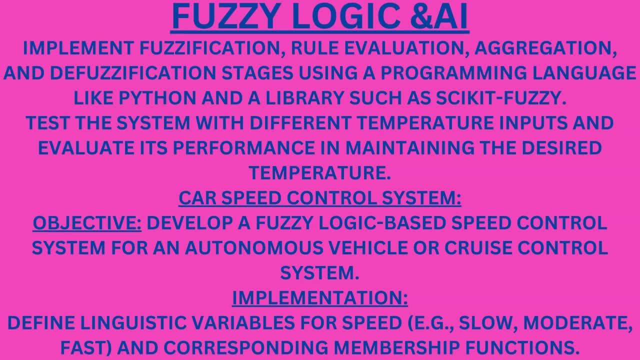 aggregation and diffuse infiction stages. using a programming language like Python and a library such as scikit fuzzy. tests the system with different temperature inputs and evaluate its performance in maintaining the desired temperature control system for an autonomous vehicle or cruise control system. implementation. define linguistic variables for speed that is, slow, moderate, fast and. 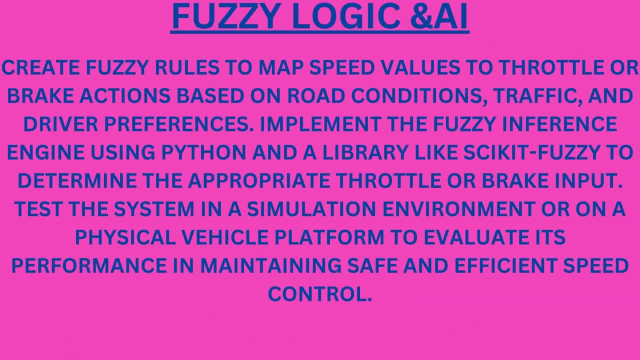 corresponding membership functions. create fuzzy rules to map speed values to throttle or brake actions based on road conditions, traffic and driver preferences. implement the fuzzy inference engine using Python and a library like scikit-fuzzy to determine the appropriate throttle or brake input. test the system in a simulation environment or on a physical vehicle. 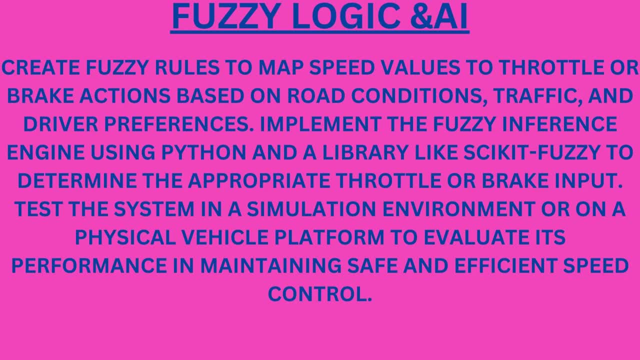 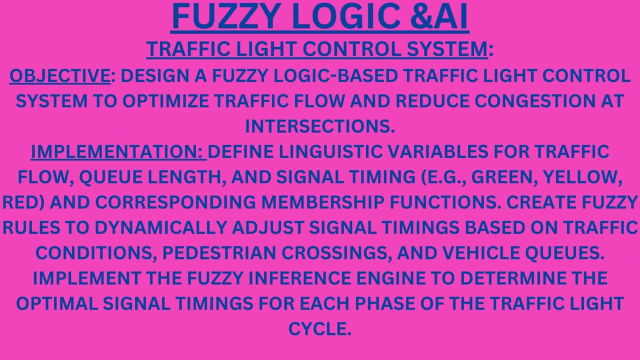 plate form to evaluate its performance in maintaining safe and efficient speed control. traffic light control system. objective design: Design a fuzzy logic-based traffic light control system to optimize traffic flow and reduce congestion at intersections. Implementation: Define linguistic variables for traffic flow, queue length and signal timing. ie green. 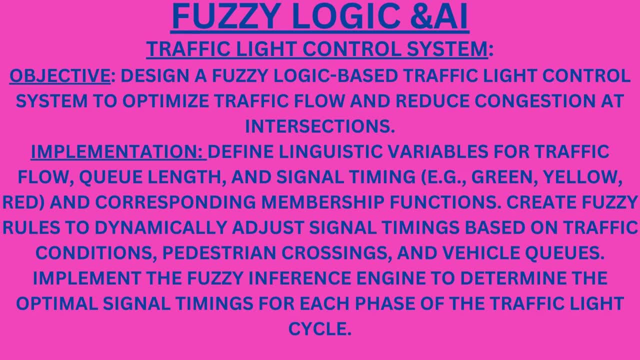 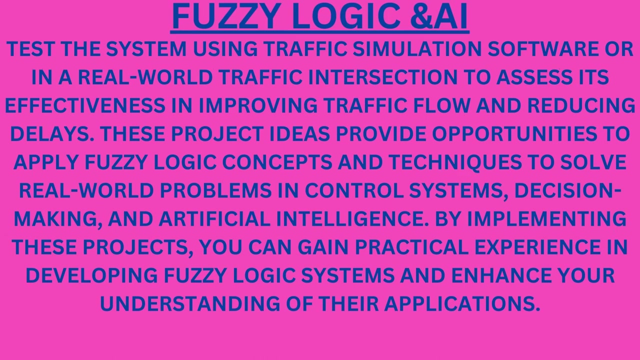 yellow, red and corresponding membership functions. Create fuzzy rules to dynamically adjust signal timings based on traffic conditions, pedestrian crossings and vehicle queues. Implement the fuzzy inference engine to determine the optimal signal timings for each phase of the traffic light cycle. Test the system using traffic simulation software or in a real-world traffic intersection. to 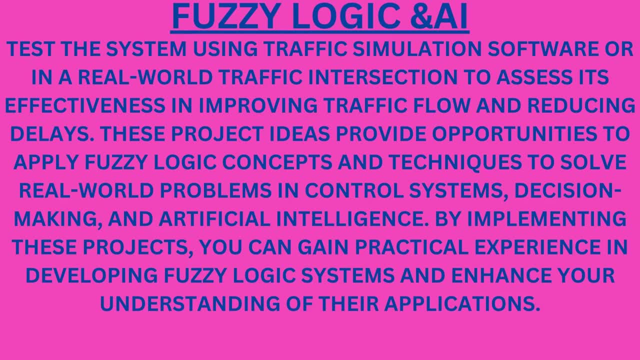 assess its effectiveness in improving traffic flow and reducing delays. These project ideas provide opportunities to apply fuzzy logic concepts and techniques to solve real-world problems in control systems, decision-making and artificial intelligence. By implementing these projects, you can gain practical experience in developing fuzzy logic. 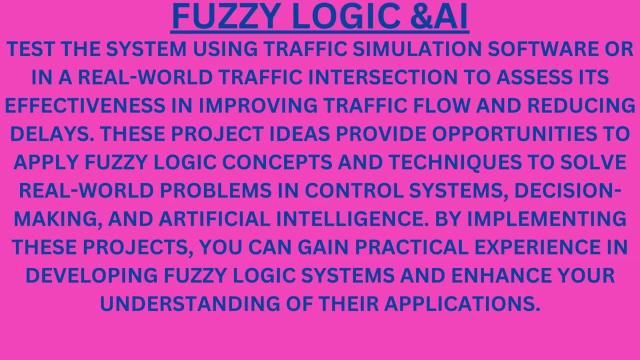 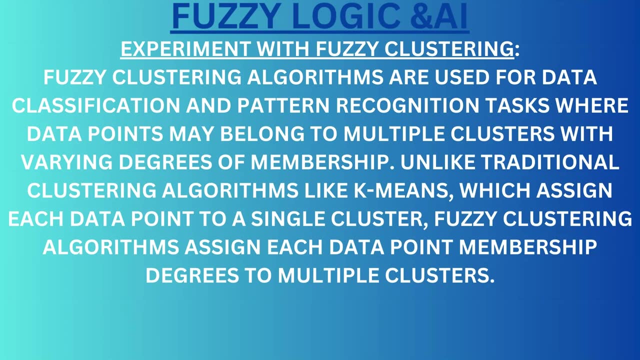 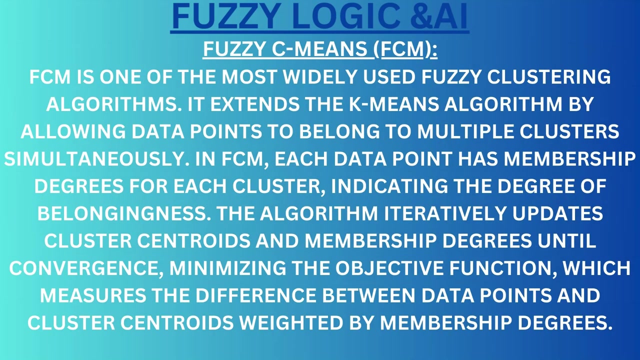 systems and enhance your understanding of their applications. Experiment with fuzzy clustering. Fuzzy clustering algorithms are used for data classification and pattern recognition tasks. Fuzzy clustering standards provide legal support and users with symptom-negative applications inyrät window processes Where data points may belong to multiple clusters with varying degrees of membership. unlike. 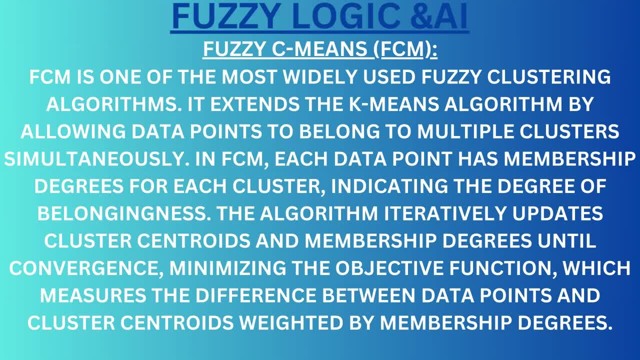 traditional clustering algorithms like k-means, which assign each data point to a single cluster. fuzzy clustering algorithms assign each data point membership degrees to multiple clusters. use fuzzy clustering algorithms. it extends the k-means algorithm by allowing data points to belong to multiple clusters simultaneously. In FCM, each data point has membership degrees. 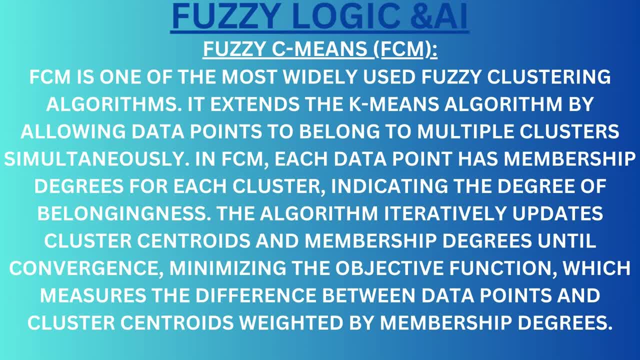 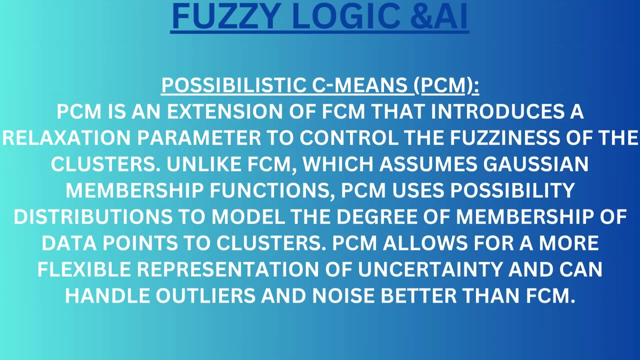 for each cluster, indicating the degree of belongingness. The algorithm iteratively updates cluster centroids and membership degrees until convergence, minimizing the objective function which measures the difference between data points and cluster centroids weighted by membership degrees. Possibleistic C-PCM. PCM is an extension of FCM that introduces a relaxation parameter to control the fuzziness. 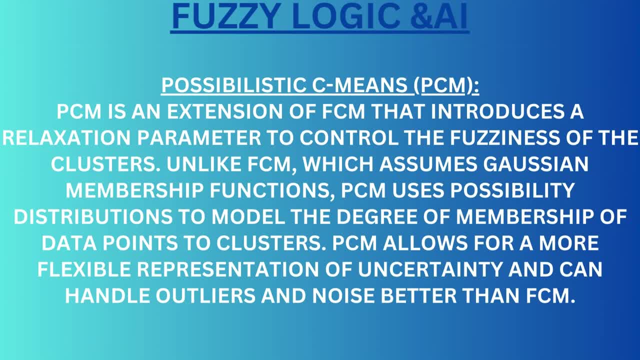 of the clusters. Unlike FCM, which, as a, assumes Gaussian membership functions, PCM uses possibility distributions to model the degree of membership of data points to clusters. PCM allows for a more flexible representation of uncertainty and can handle outliers and noise better than FCM. 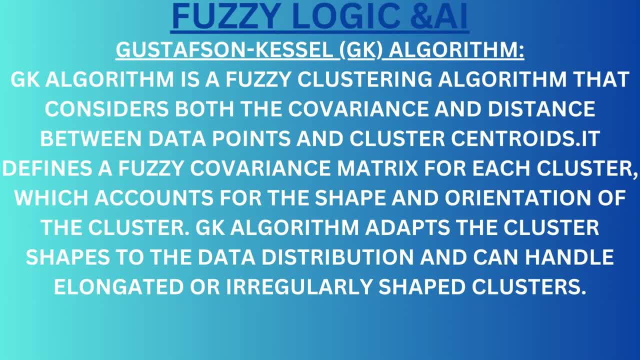 Gustavsson-Kessel GK algorithm. GK algorithm is a fuzzy clustering algorithm that considers both the covariance and distance between data points and cluster centripes. It defines a fuzzy covariance matrix for each cluster which accounts for the shape and orientation of the cluster. GK algorithm adapts the cluster shapes to the data distribution and can handle 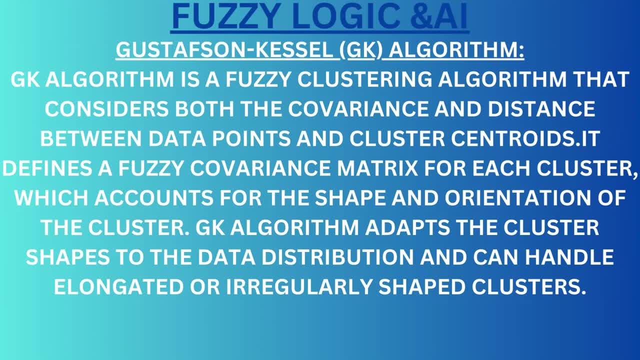 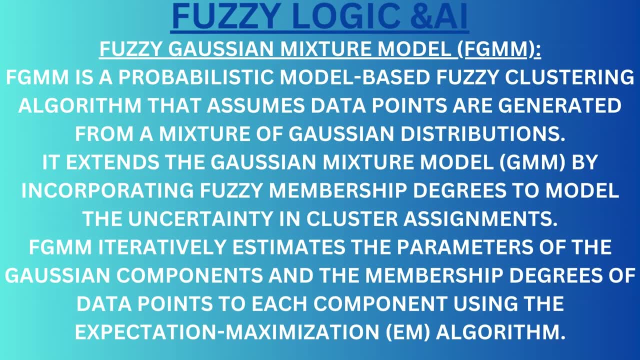 elongated or irregularities. The Fuzzy Gaussian Mixture Model- FGMM- is a probabilistic model-based fuzzy clustering algorithm that assumes data points are generated from a mixture of Gaussian distributions. It extends the Gaussian Mixture Model by incorporating fuzzy membership degrees to model the uncertainty in cluster assignments. 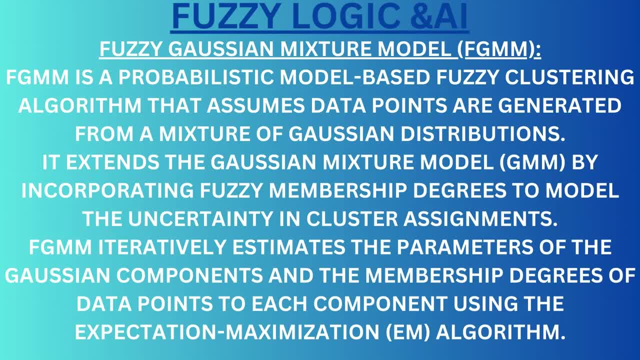 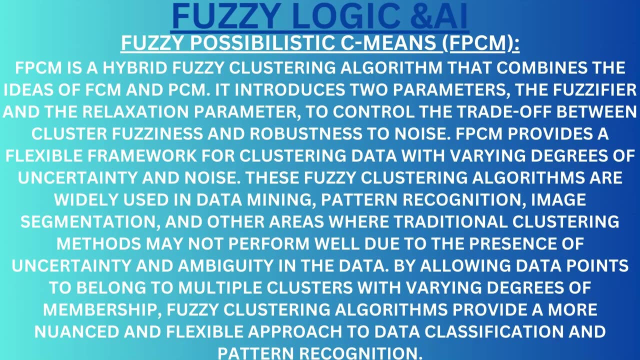 FGMM iteratively estimates the parameters of the Gaussian components and the membership degrees of data points to each component using the Expectation-Maximization algorithm. Fuzzy Possibilistic C-Means- FPCM- FPCM is a hybrid fuzzy clustering algorithm. FPCM is a hybrid fuzzy clustering algorithm. 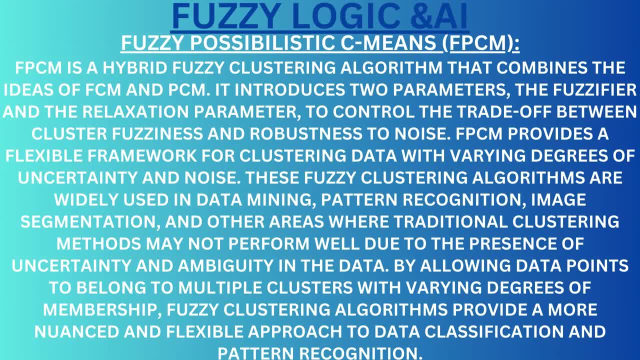 FPCM is a hybrid fuzzy clustering algorithm that combines the ideas of FCM and PCM. it introduces two parameters, the fuzzy fire and the relaxation parameter, to control the trade-off between cluster fuzziness and robustness to noise. FPCM provides a flexible framework for clustering data with varying degrees of uncertainty and noise. these fuzzy 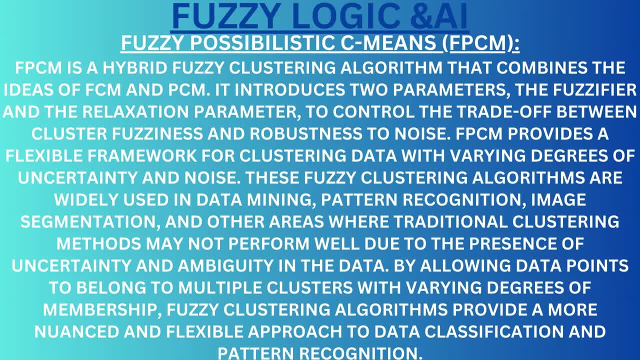 clustering algorithms are widely used in data mining, pattern recognition, image segmentation and other areas where traditional clustering methods may not perform well due to the presence of uncertainty and ambiguity in the data. by allowing data points to belong to multiple clusters with varying degrees of membership, fuzzy clustering algorithms provide a more nuanced 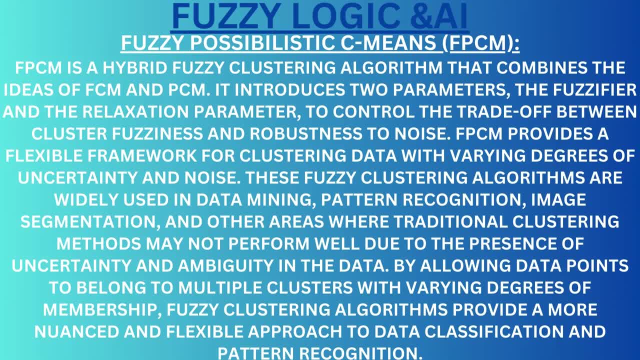 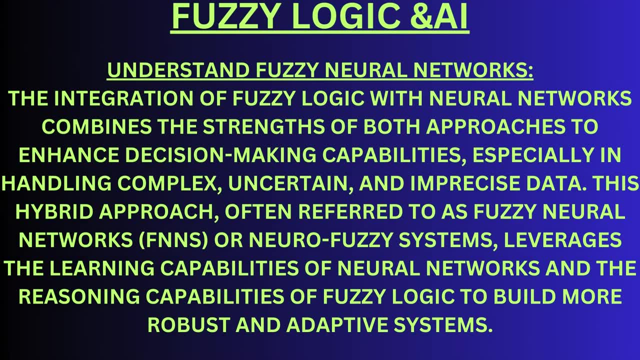 and flexible approach to data classification and pattern recognition. understand fuzzy neural networks. the integration of fuzzy logic with neural networks combines the strengths of both approaches to enhance decision-making capabilities, especially in handling complex, uncertain and imprecise data. this hybrid approach, often referred to as fuzzy neural networks- FNNS. 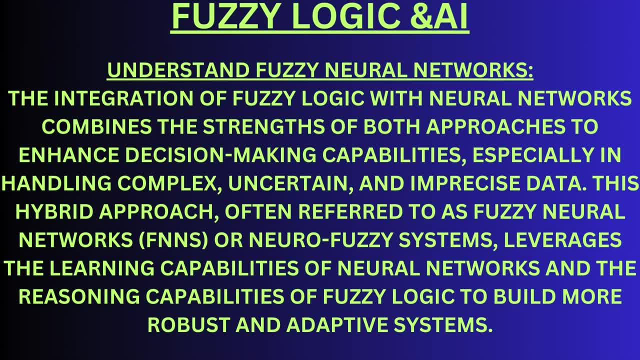 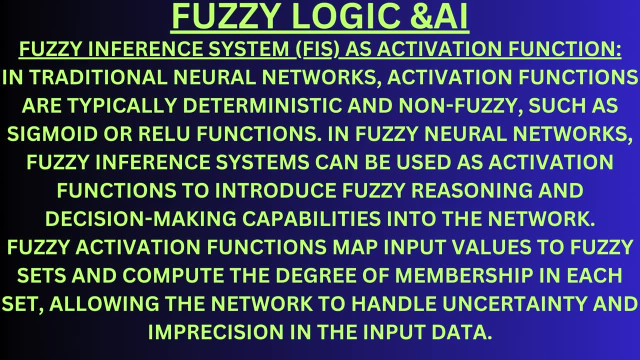 or neuro fuzzy systems, leverages the learning capabilities of neural networks and the reasoning capabilities of fuzzy logic to build more robust and adaptive systems. fuzzy inference system, FIS as activation function. in traditional neural networks, activation functions are typically deterministic and non fuzzy, such as sigmoid or RELU functions in fuzzy. 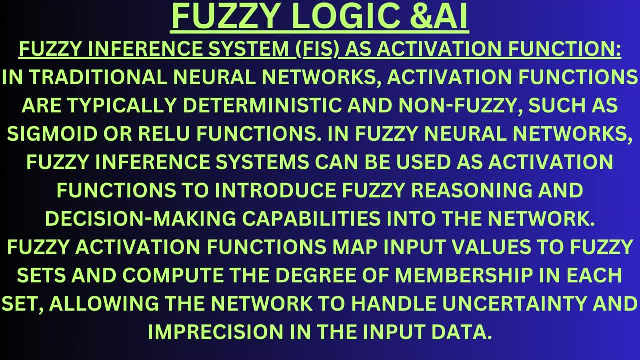 neural networks. fuzzy inference systems can be used as activation functions to introduce fuzzy reasoning and decision-making capabilities into the network. fuzzy activation functions map input values to fuzzy sets and compute the degree of membership in each set, allowing the network to handle uncertainty and imprecision in the input data. 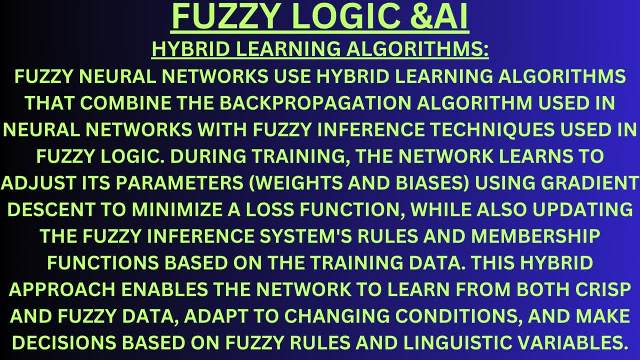 hybrid learning algorithms. fuzzy neural networks use hybrid learning algorithms that combine the back propagation algorithm used in neural networks with fuzzy inference techniques used in fuzzy logic. during training, the net network learns to adjust its parameters, weights and biases using gradient descent to minimize the loss function, while also updating the fuzzy inference systems. 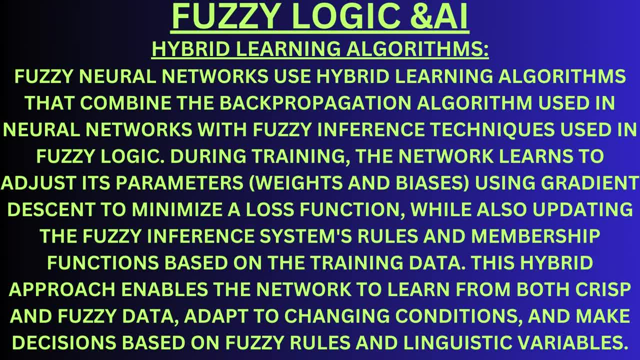 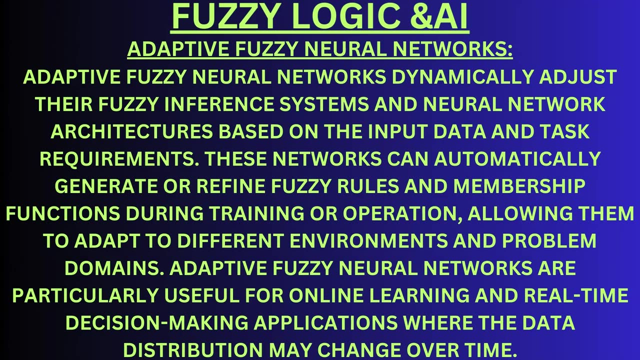 rules and membership functions based on the training data. this hybrid approach enables the network to learn from both crisp and fuzzy data, adapt to changing conditions and make decisions based on fuzzy rules and linguistic variables. adaptive fuzzy neural networks. adaptive fuzzy neural networks dynamically adjust their fuzzy inference systems and neural network architectures based on the data. 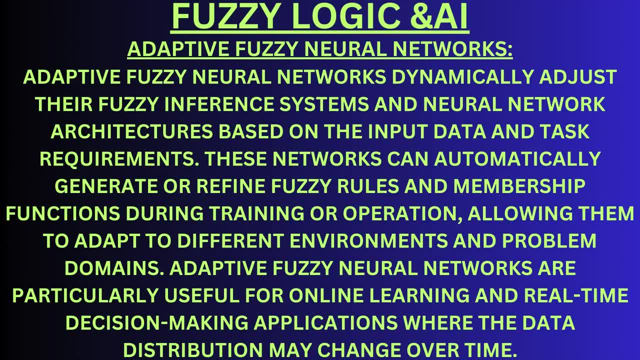 based on the input data and task requirements. these were. networks can automatically generate or refine fuzzy rules and membership functions during training or operation, allowing them to adapt to different environments and problem domains. adaptive fuzzy neural networks are particularly useful for online learning and real-time decision-making applications, where the 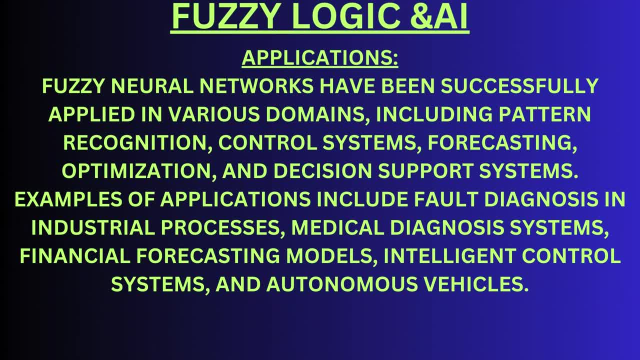 data distribution may change over time. applications fuzzy neural networks have been successfully applied in various domains, including pattern recognition, control systems, forecasting, optimization and decision support systems. examples of applications include fault diagnosis in industrial processes, medical diagnosis systems, financial forecasting models, intelligent control systems and autonomous vehicles. by integrating fuzzy logic with neural networks, fuzzy neural networks offer a 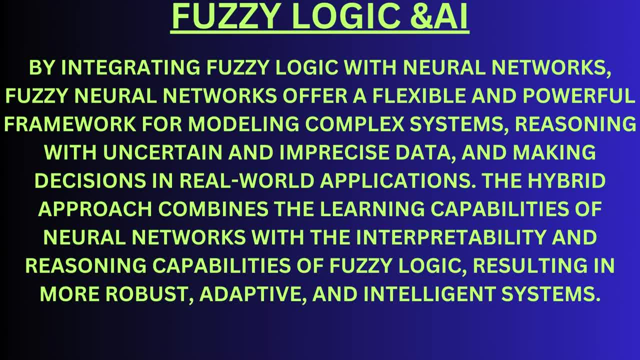 flexible and powerful framework for modeling complex systems, reasoning with uncertain and imprecise data and making decisions in real-world applications. the hybrid approach combines the learning capabilities of neural networks with the interpretability and reasoning capabilities of fuzzy logic, resulting in more robust, adaptive and intelligent systems. 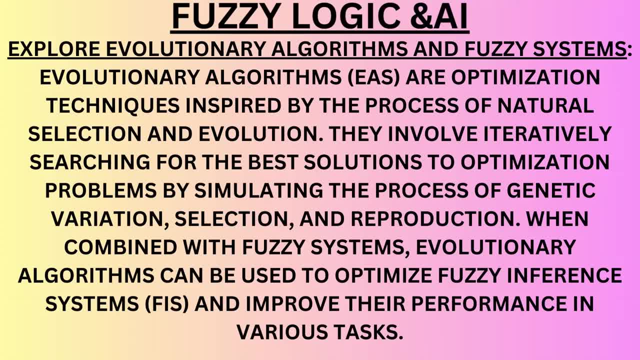 explore evolutionary algorithms and fuzzy systems. evolutionary algorithms- EAS- are optimization techniques inspired by the process of natural selection and evolution. they involve iteratively searching for the best solutions to optimization problems by simulating the process of genetic variation, selection and reproduction. when combined with fuzzy systems, evolutionary 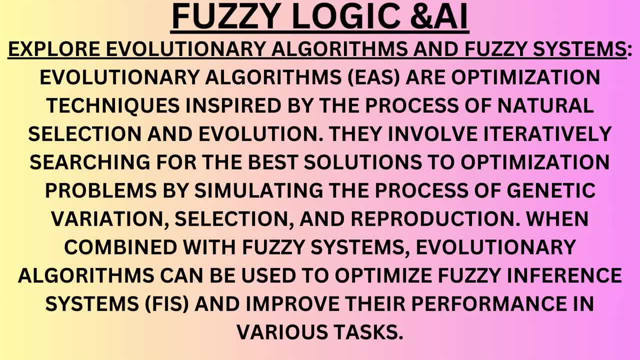 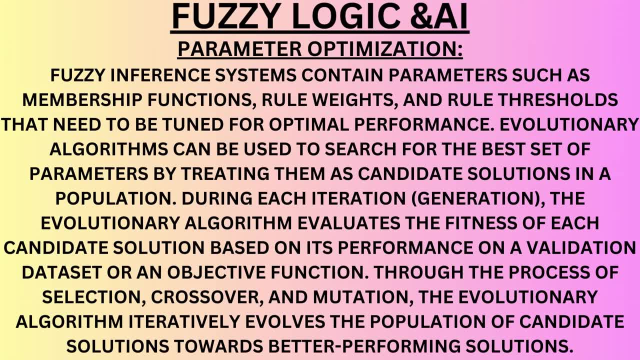 can be used to optimize fuzzy inference systems, FIS, and improve their performance in various tasks. parameter optimization: fuzzy inference systems contain parameters such as membership functions, rule weights and rule thresholds that need to be tuned for optimal performance. evolutionary algorithms can be used to search for the best set of parameters by treating them. 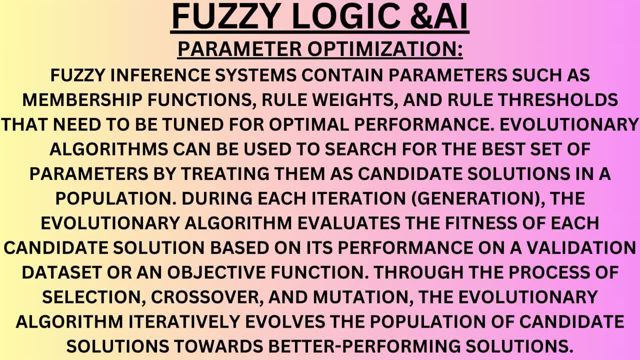 as candidate solutions in a population. during each iteration generation, the evolutionary algorithm evaluates the fitness of each candidate solution based on its performance, on a validation data set or an objective function. through the process of selection, crossover and mutation, the evolutionary algorithm iteratively evolves the population of candidate. 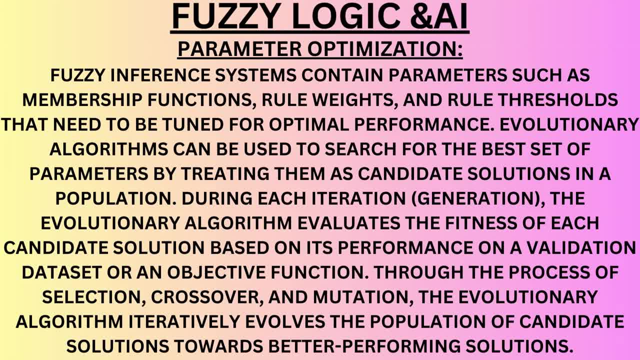 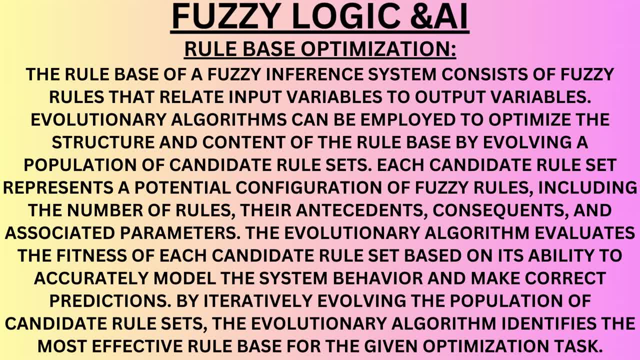 solutions towards better performing solutions: rule based optimization. the rule base of a fuzzy inference system consists of fuzzy rules that relate input variables to output variables. evolutionary algorithms can be employed to optimize the structure and content of the rule base by evolving a population of candidate rule sets. each candidate rule set. 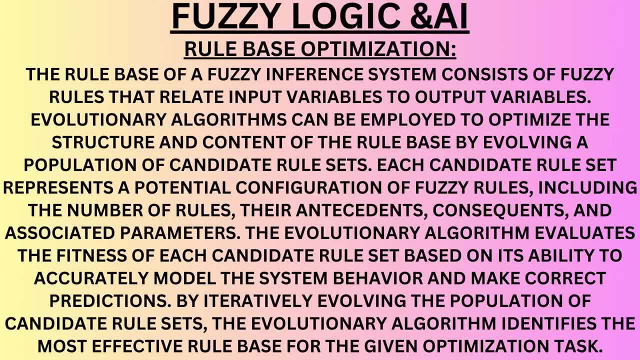 represents a potential configuration of fuzzy rules, including the number of rules, their antecedents, consequence and associated parameters. the evolutionary algorithm evaluates the fitness of each candidate rules set based on its ability to accurately model the system behavior and make correct predictions by iteratively evolving the population of 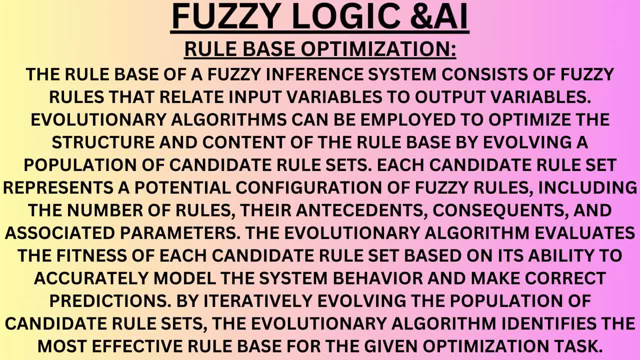 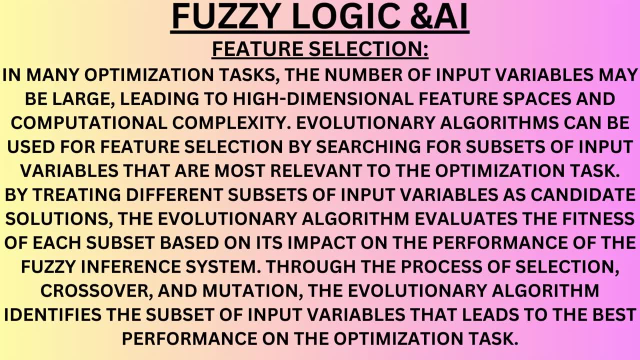 candidate rule sets, the evolutionary algorithm identifies the most effective rules base for the given optimization task. feature selection: in many optimization tasks the number of input variables may be large, leading to high-dimensional feature spaces and computational complexity. evolutionary algorithms can be used for feature selection by searching for subsets of a. 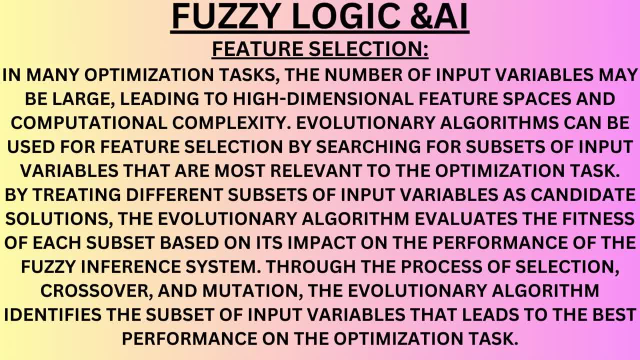 set of input variables that are most relevant to the optimization task, by treating different subsets of input variables as candidates solutions. the evolutionary keywords: the value evaluates the fitness of each subset based on its impact of the performance of the fuzzy inference system through the process of selection, crossover and mutation. the evolutionary algorithm identifies the subset of: 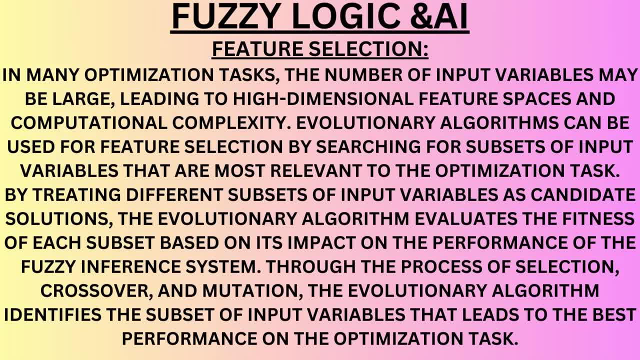 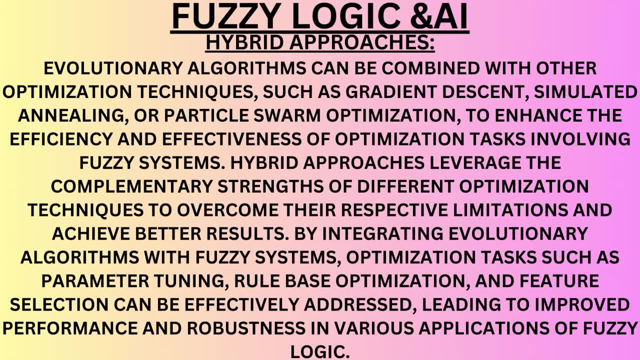 variables in the following way that give better performance for Performers. after: identifies the subset of input variables that leads to the best performance on the optimization task. Hybrid Approaches: Evolutionary algorithms can be combined with other optimization techniques, such as gradient descent, simulated annealing or practical. 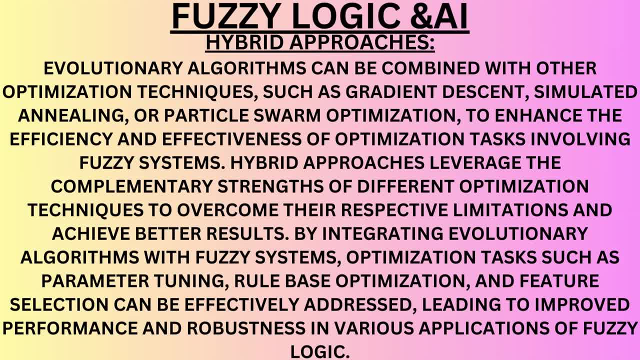 swarm optimization. To enhance the efficiency and effectiveness of optimization tasks involving fuzzy systems, hybrid approaches leverage the complementary strengths of different optimization techniques to overcome their respective limitations and archive better results. By integrating evolutionary algorithms with fuzzy systems, optimization tasks such as parameter tuning, rule-based optimization and feature selection can be effectively addressed. 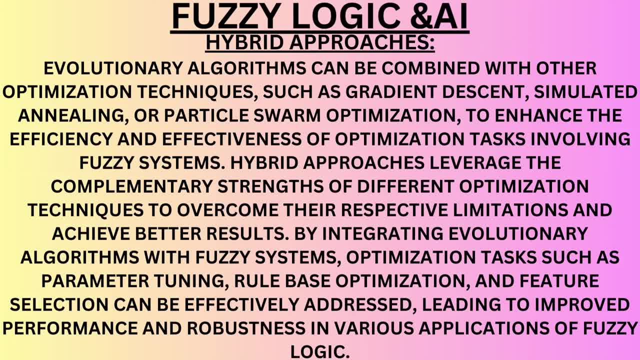 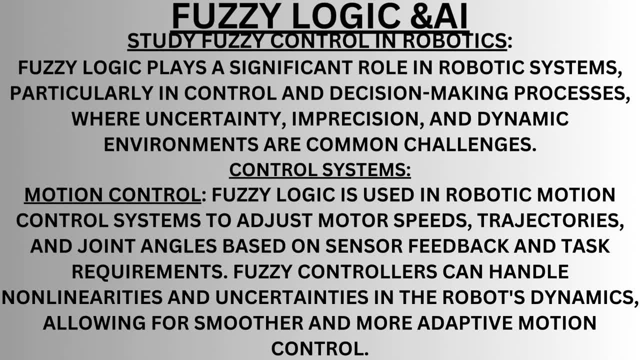 leading to improved performance and robustness. Fuzzy Logic Study- Fuzzy Control in Robotics. Fuzzy logic plays a significant role in robotic systems, particularly in control and decision-making processes, where uncertainty in precision and dynamic environments are common challenges. Control Systems- Motion Control: Fuzzy logic is used in robotic motion control systems to adjust motor speeds, trajectories. 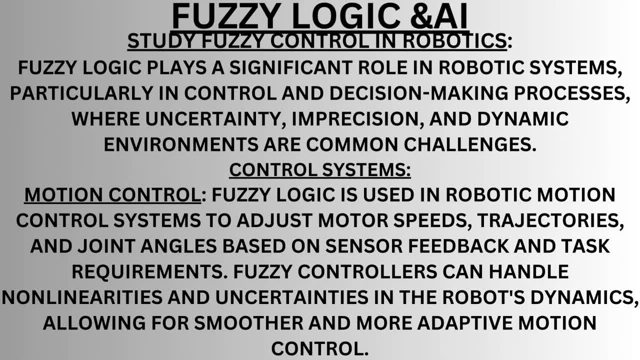 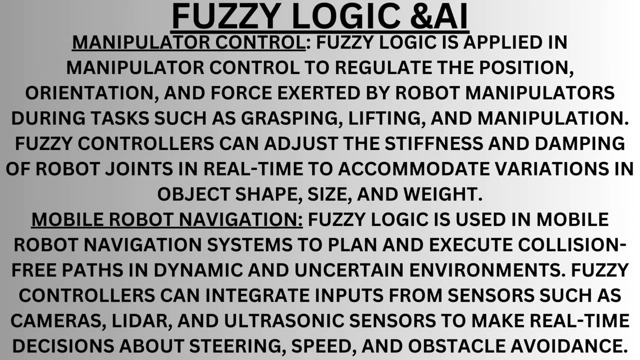 and joint angles based on sensor feedback and task requirements. Fuzzy controllers can handle non-linearities and uncertainties in the robot's dynamics, allowing for smoother and more adaptive motion control. Manipulator Control: Fuzzy logic applied in manipulator control to regulate the position, orientation and force exerted by robot manipulators during. 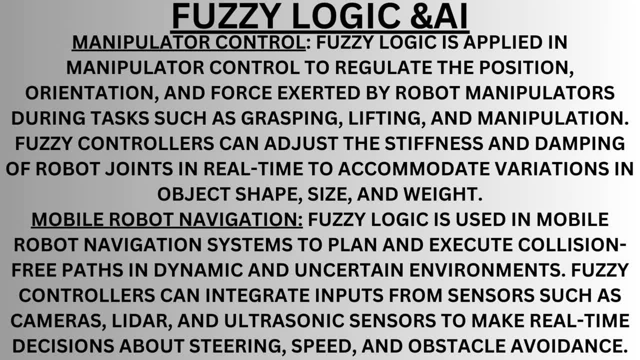 tasks such as grasping, lifting and manipulation. Fuzzy controllers can adjust the stiffness and damping of robot joints in real-time to accommodate variations in object shape, size and weight. Mobile Robot Navigation. Fuzzy logic is used in mobile robot navigation systems to plan and execute collision-free paths in dynamic and uncertain environments. 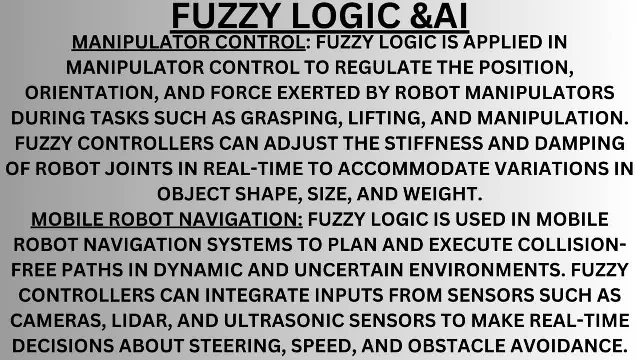 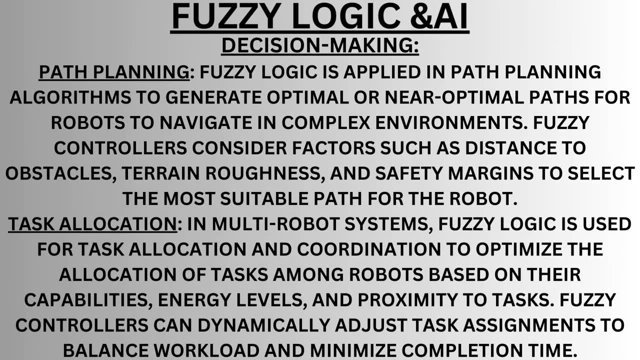 Fuzzy controllers can easily assembly, configure and produce functional machines that are available. Fuzzy controllers can integrate inputs from sensors such as cameras, lidar and ultrasonic sensors to make real-time decisions about steering speed and obstacle avoidance: Decision-Making Path Planning. 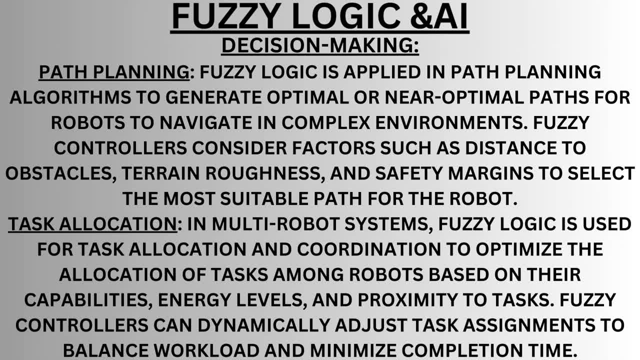 Fuzzy logic is applied in path-planning algorithms to generate optimal or near-optimal paths for robots to navigate in complex environments. Fuzzy controllers consider factors such as distance to obstacles, terrain roughness and safety margins to select the most suitable path for the robot. 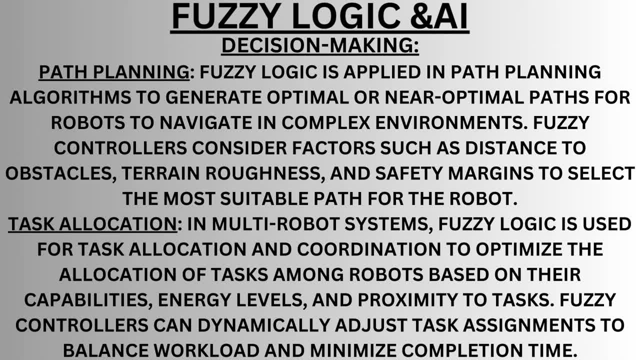 Task Allocation In multi-robot systems. fuzzy logic is used for task allocation and coordination to optimize the allocation of tasks among robots based on their capabilities, energy levels and proximity to tasks. Fuzzy controllers can dynamically adjust task assignments to balance workload and minimize completion time. 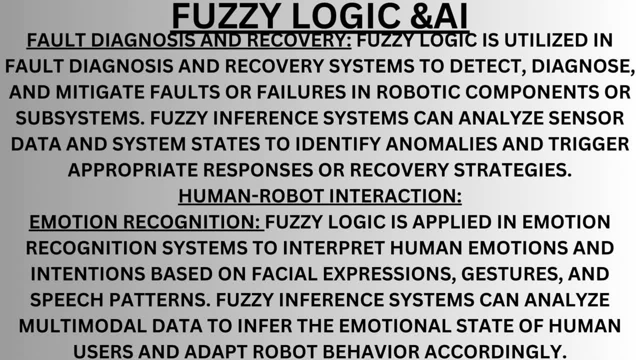 Fault Diagnosis and Recovery. Fuzzy logic is utilized in fault diagnosis and recovery systems to detect, diagnose and mitigate faults or failures in robotic components or subsystems. Fuzzy inference systems can analyze sensor data and system states. to analyze the data and system states: 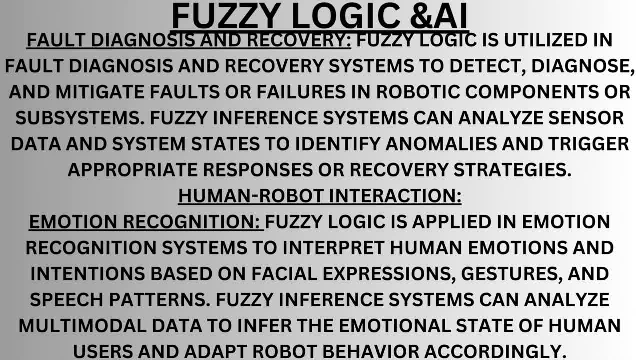 Fuzzy inference systems can identify anomalies and trigger appropriate responses or recovery strategies. Human-Robot Interaction- Emotion Recognition. Fuzzy logic is applied in emotion recognition systems to interpret human emotions and intentions based on facial expressions, gestures and speech patterns. Fuzzy inference systems can analyze multi-model data to infer results. 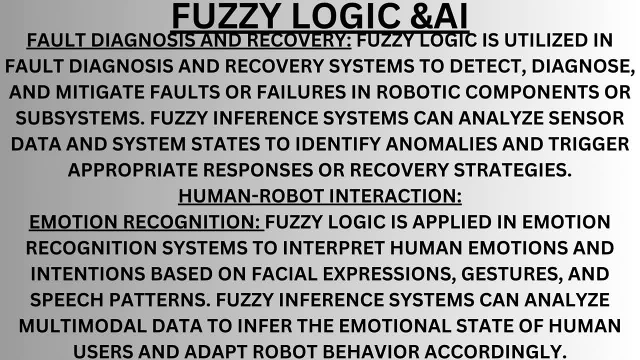 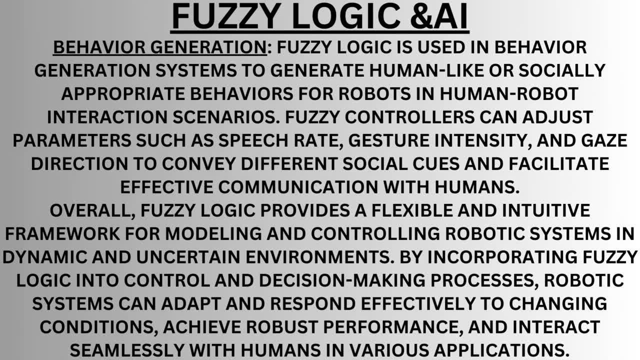 Fuzzy inference can be used to infer the emotional state of human users and adapt robot behavior accordingly. Fuzzy logic is used in behavior generation systems to generate human-like or socially appropriate behaviors for robots. in human-robot interaction scenarios, Fuzzy controllers can adjust parameters such as speech rate, gesture intensity and gaze. 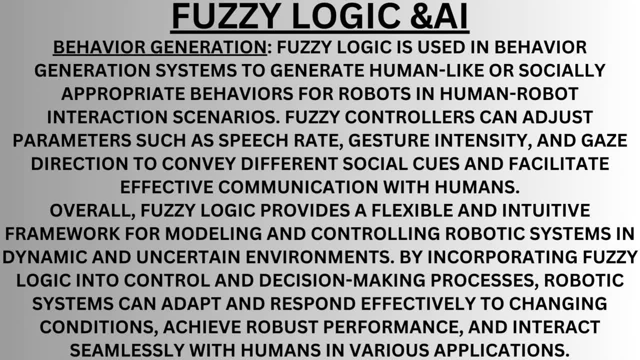 direction to convey different responses. Fuzzy logic can be used in behavior generating systems to generate human-like or socially-appropriate social cues and facilitate effective communication with humans. Overall, fuzzy logic provides a flexible and intuitive framework for modeling and controlling robotic systems in dynamic and 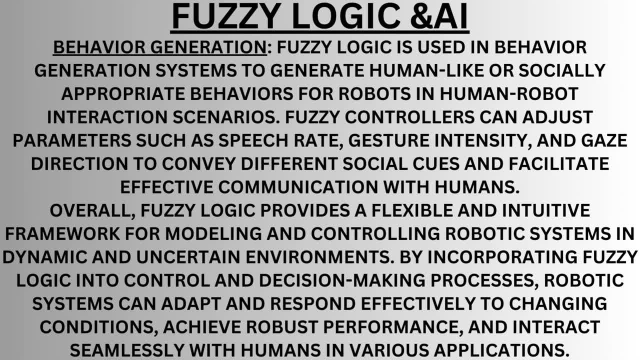 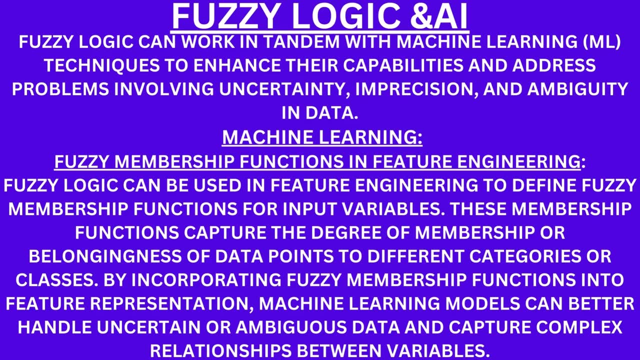 uncertain environments. By incorporating fuzzy logic into control and decision-making processes, robotic systems can adapt and respond effectively to changing conditions, achieve robust performance and interact seamlessly with humans. in various applications. Fuzzy logic can work in tandem with machine learning techniques to enhance their capabilities and address problems involving 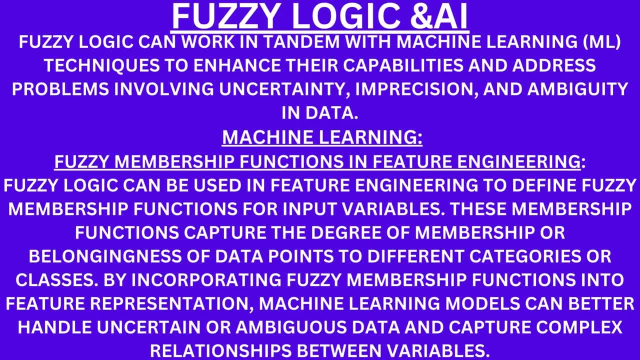 uncertainty, imprecision and ambiguity in data machine learning. Fuzzy membership functions in feature engineering. Fuzzy logic can be used in feature engineering to define fuzzy membership functions for input variables. These membership functions capture the degree of membership or belongingness of data points to different categories or classes By incorporating 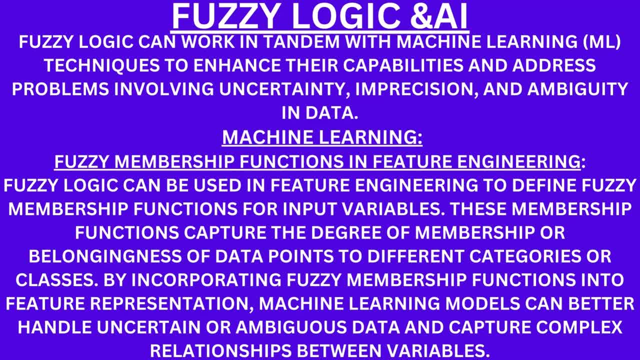 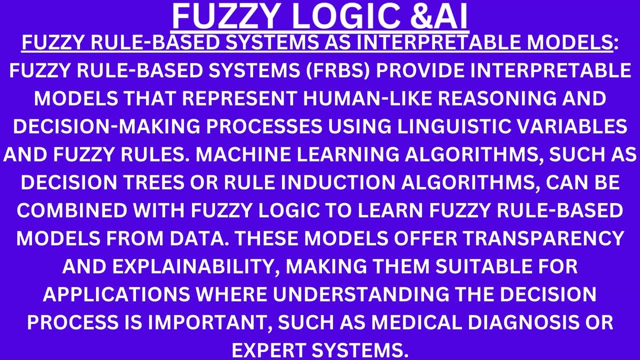 fuzzy membership functions into feature representation. machine learning models can better handle uncertain or ambiguous data points. Fuzzy rule-based systems as interpretable models. Fuzzy rule-based systems provide interpretable models that represent human-like reasoning and decision-making processes using linguistic variables and fuzzy rules. Machine learning algorithms, such as decision trees or rule. 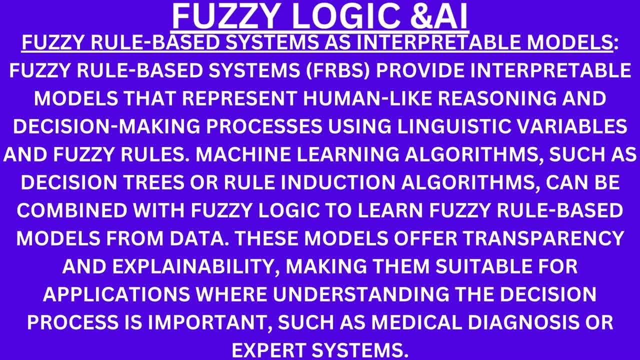 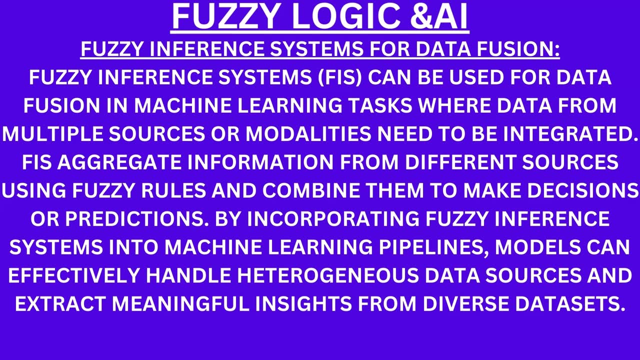 induction algorithms can be combined with fuzzy logic to learn fuzzy rule-based model models from data. These models offer transparency and explainability, making them suitable for applications where understanding the decision process is important, such as medical diagnoses or expert systems. Fuzzy inference systems for data fusion Fuzzy inference systems can be used. 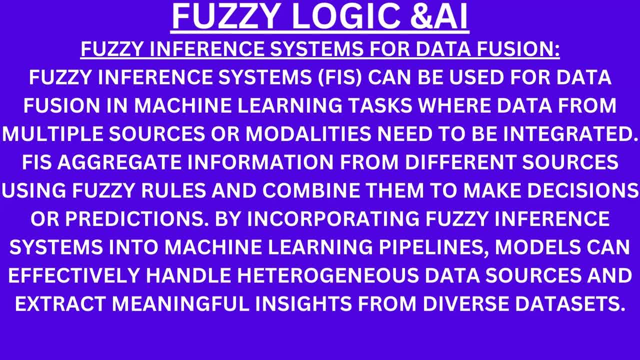 for data fusion in machine learning tasks where data from multiple source or modalities need to be integrated. FIS aggregate information from different sources using fuzzy rules and combine them to make decisions or predictions. By incorporating fuzzy inference systems into machine learning pipelines, models can effectively handle heterogeneous data source and extract. 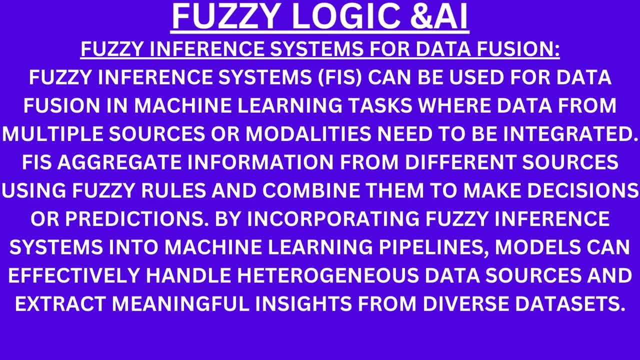 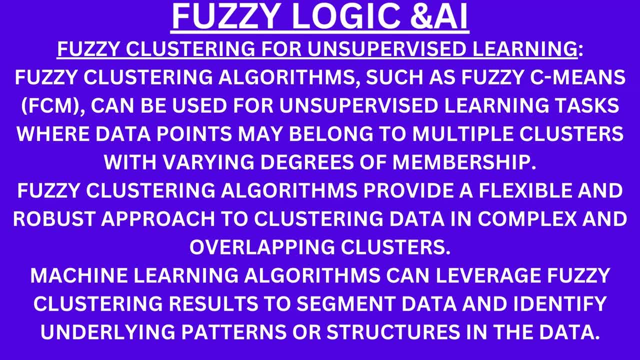 meaningful insights from diverse data sets. Fuzzy clustering for unsupervised learning. Fuzzy clustering algorithms, such as fuzzy C-means, FCM, can be used for unsupervised learning tasks where data points may belong to multiple clusters with varying degrees of membership. Fuzzy clustering algorithms provide a flexible and robust approach to clustering data. 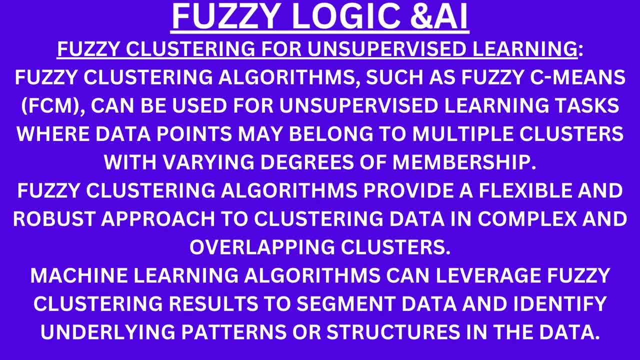 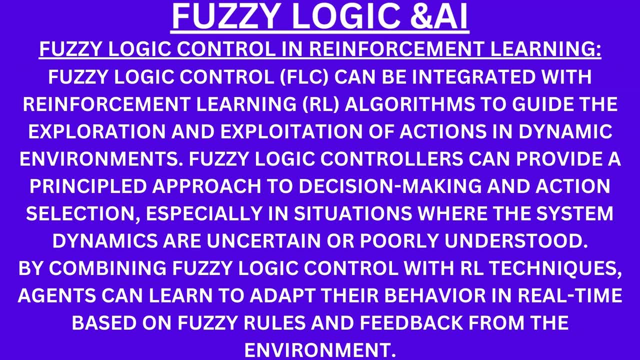 in complex and overlapping clusters. Machine learning algorithms can leverage fuzzy clustering underlying patterns or structures in the data. Fuzzy logic control in reinforcement learning. Fuzzy logic control- FLC- can be integrated with reinforcement learning algorithms to guide the exploration and exploitation of actions in dynamic environments. Fuzzy logic controllers. 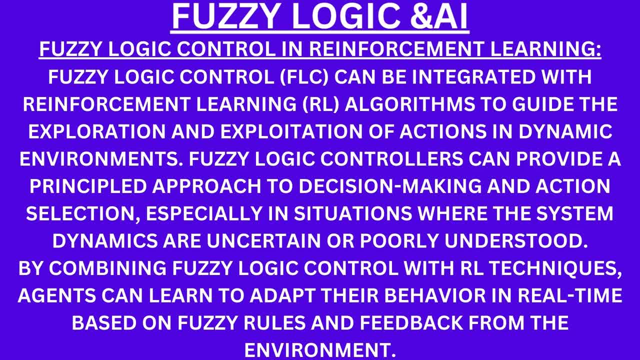 can provide a principal approach to decision making and action selection, especially in situations where the system dynamics are uncertain or poorly understood. By combining fuzzy logic control with reinforcement learning techniques, agents can learn to adapt their behavior in real time based on fuzzy rules and feedback from the environment. 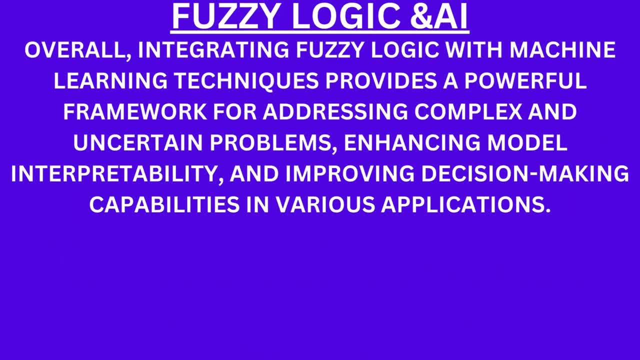 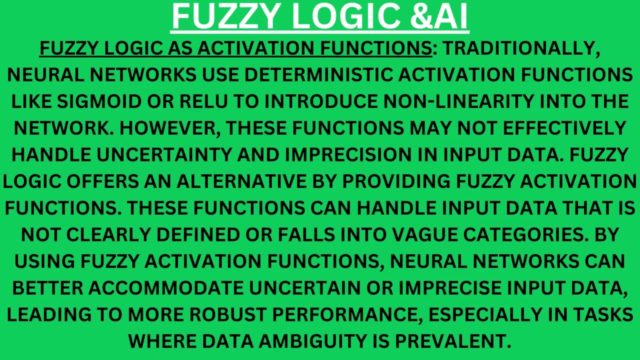 Overall. integrating fuzzy logic with machine learning techniques provide a powerful framework for addressing complex and uncertain problems, model interpretability and improving decision making capabilities in various applications. Fuzzy logic as activation functions. Traditionally, neural networks use deterministic activation functions like sigmoid or RELU to introduce non-linearity into the network. However, these 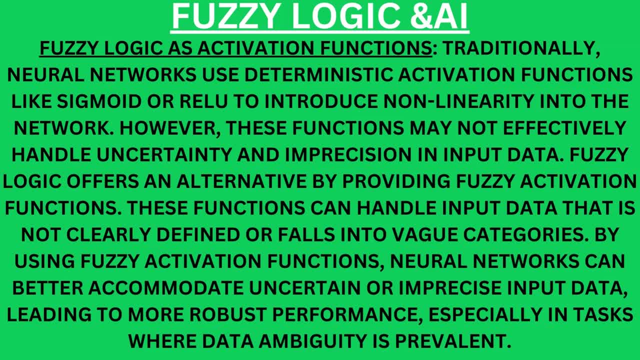 functions may not effectively handle uncertainty and impression in input data. Fuzzy logic is an alternative. by providing fuzzy activation functions, These functions can handle input data that is not clearly defined or falls into vague categories. By using fuzzy activation functions, neural networks can better accommodate uncertain or imprecise input data. leading 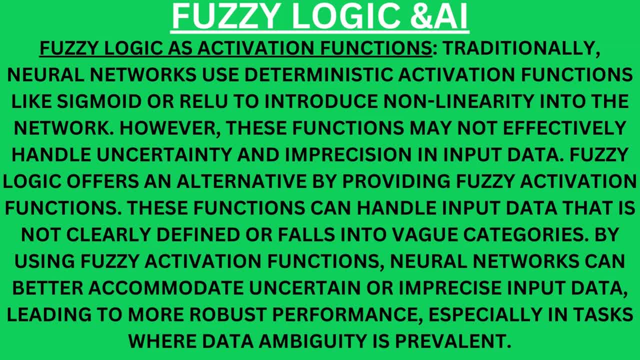 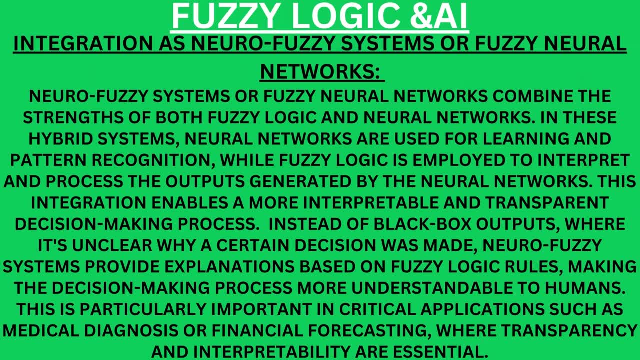 to more robust performance, especially in tasks where data ambiguity is prevalent. After date: Breark time: Ilja sorte Ottestia Integer Torsion Spanning Sherningmerربas Venue as neuro fuzzy systems or fuzzy neural networks. Neuro fuzzy systems or fuzzy neural networks. 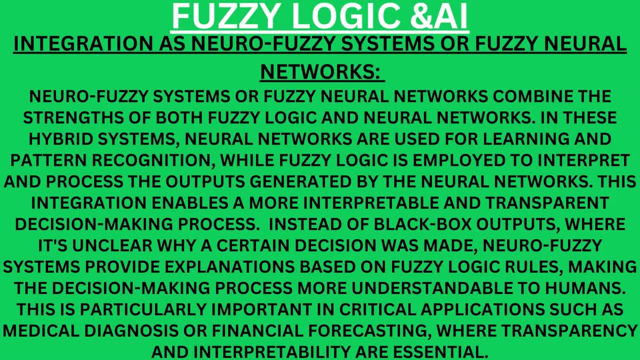 combine the strengths of both fuzzy logic and neural networks In these hybrid systems. neural networks are used for learning and pattern recognition, while fuzzy logic is employed to interpret and process the outputs generated by the neural networks. This integration enables a more interpretable and transparent decision-making process Instead of black box. 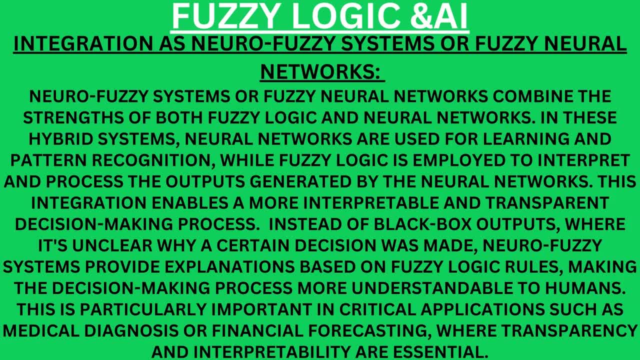 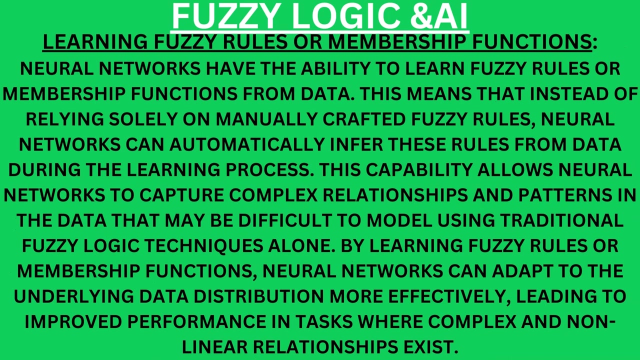 outputs. where it's unclear why a certain decision was made, neuro fuzzy systems provide explanations based on fuzzy logic rules, making the decision-making process more understandable to humans. This is particularly important in critical applications such as medical development and medical research. Neural networks have the ability to learn fuzzy rules or membership functions from data. 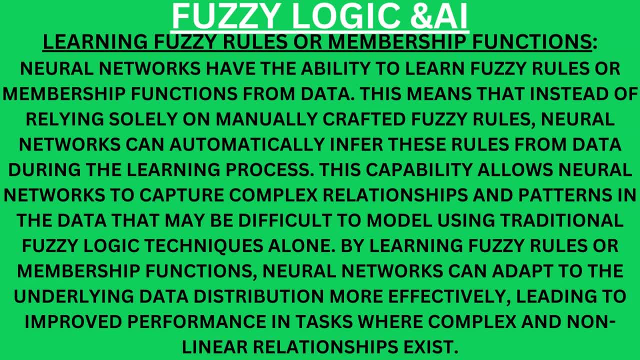 This means that, instead of relying solely on manually crafted fuzzy rules, neural networks can automatically infer these rules from data during the learning process. This capability allows for a more transparent and transparent decision-making process. Neural networks can capture complex relationships and patterns inside the data that may be difficult. 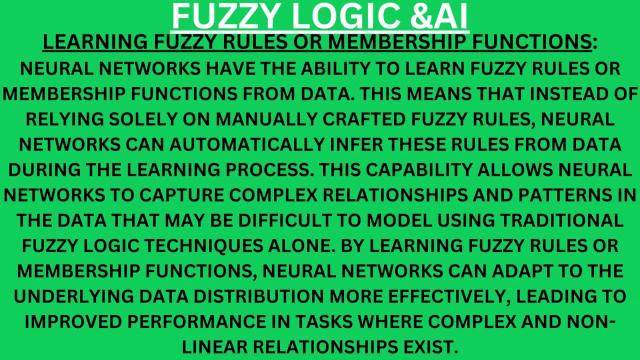 to model using traditional fuzzy logic techniques alone. By learning fuzzy rules or membership functions, neural networks can adapt to the underlying data distribution more effectively, leading to improved performance in tasks where complex and non-linear relationships exist. What are the advantages of neuro fuzzy systems In summary? 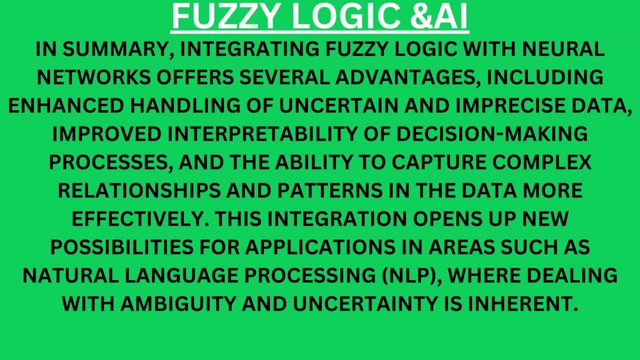 Integrating fuzzy logic with neural networks offers several advantages, including enhanced handling of uncertain and imprecise data, improved interpretability of decision-making processes and the ability to capture complex relationships and patterns in the data more effectively. This integration opens up new possibilities for applications in areas such as natural language processing, NLP, where dealing with ambiguity and uncertainty is inherent. 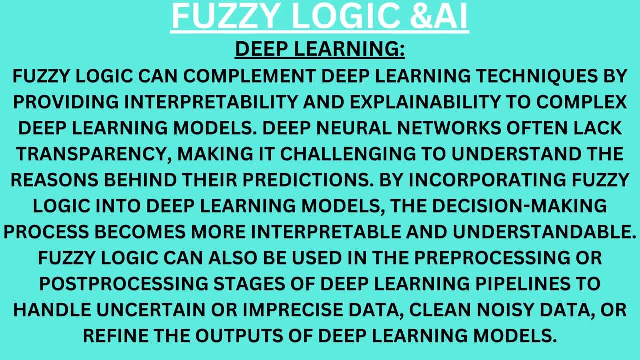 Deep learning. Fuzzy logic can complement deep learning techniques by providing interpretability and explainability to complex deep learning models. Deep neural networks often lack transparency, making it challenging to understand the reasons behind. By incorporating fuzzy logic into deep learning models, the decision-making process becomes more interpretable and understandable. 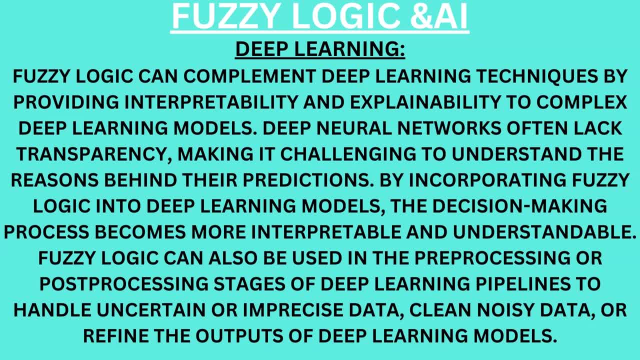 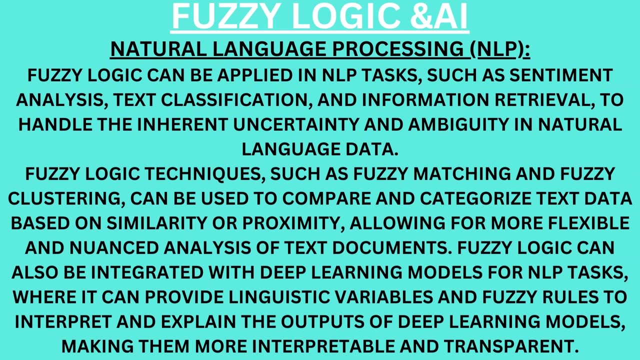 Fuzzy logic can also be used in the pre-processing or post-processing stages of deep learning pipelines to handle uncertain or imprecise data, clean noisy data or refine the outputs of deep learning models. Natural language processing: Fuzzy logic can be applied in natural language processing tasks such as sentiment analysis, text classification and information retrieval, to handle the inherent uncertainty and ambiguity in natural language data. 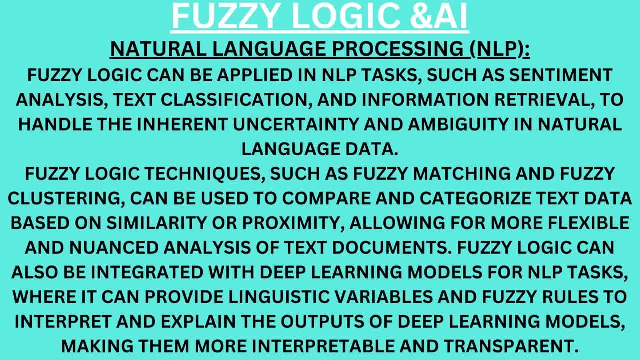 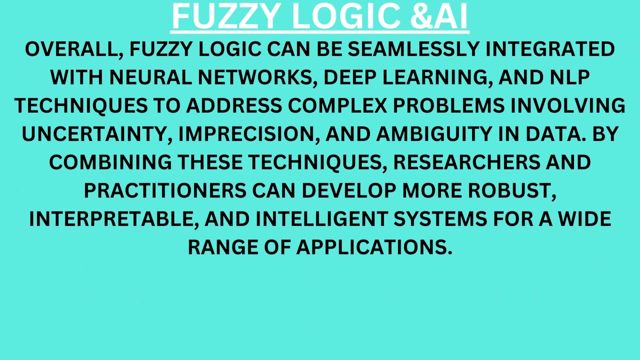 Fuzzy logic techniques such as fuzzy matching and fuzzy clustering can be used to compare and categorize text data based on similarity or proximity, Allowing for more flexible and nuanced analysis of text documents. Fuzzy logic can also be integrated with deep learning models for natural language processing tasks, where it can provide linguistic variables and fuzzy rules to interpret and explain the outputs of deep learning models, making them more interpretable and transparent. 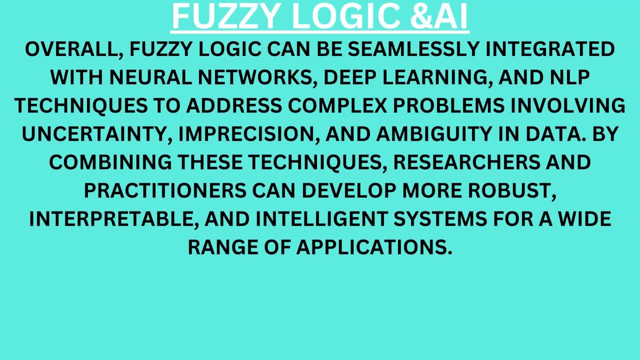 Overall fuzzy logic can be seamlessly integrated with neural networks or interfaces, deep learning and NLP techniques to address complex problems involving uncertainty, imprecision and ambiguity in data. By combining these techniques, researchers and practitioners can develop more robust, interpretable and intelligent systems for a wide range of applications. 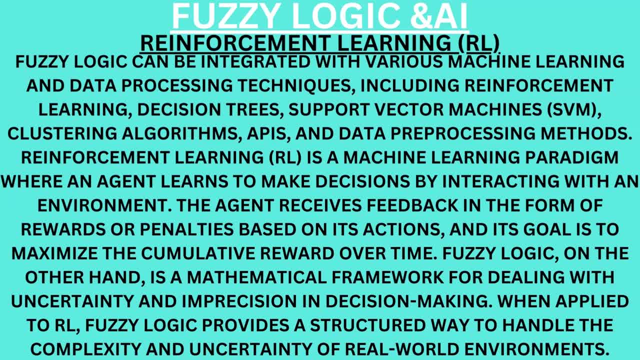 Reinforcement learning. Fuzzy logic can be integrated with various machine learning and data processing techniques, including reinforcement learning, decision trees, support vector machines, SVM, clustering algorithms, APIs and data pre-processing methods. Reinforcement learning is a machine learning paradigm where an agent learns to make decisions by interacting with. 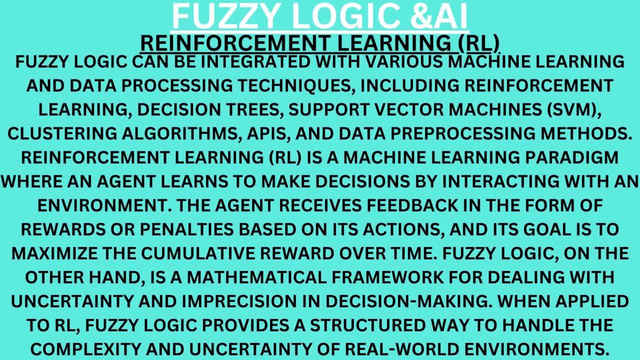 an environment. The agent receives feedback in the form of rewards or penalties based on its actions, and its goal is to achieve the desired outcome. Fuzzy logic, on the other hand, is a mathematical framework for dealing with uncertainty and imprecision in decision-making. When applied to reinforcement learning, fuzzy logic provides 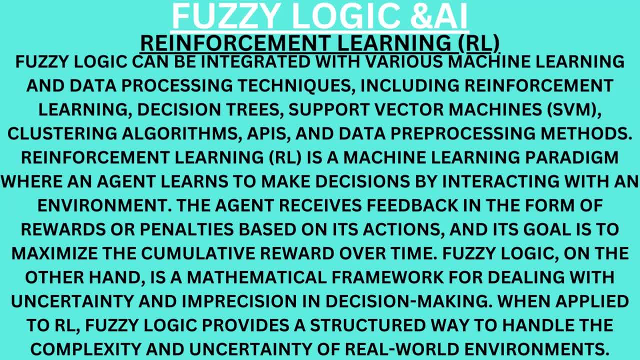 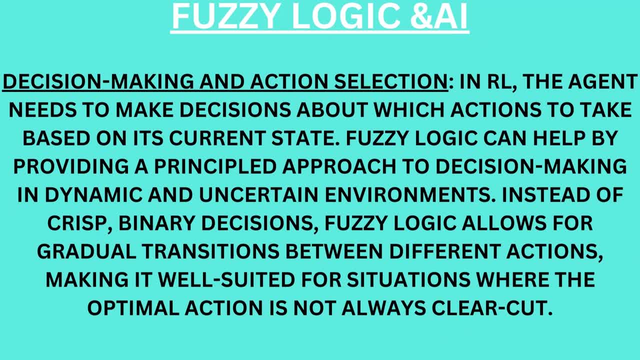 a structured way to handle the complexity and uncertainty of real-world environments. Decision-making and action selection: In reinforcement learning, the agent needs to be able to make decisions based on its actions and actions. In reinforcement learning, the agent needs to make decisions about which actions to take based on its current state. 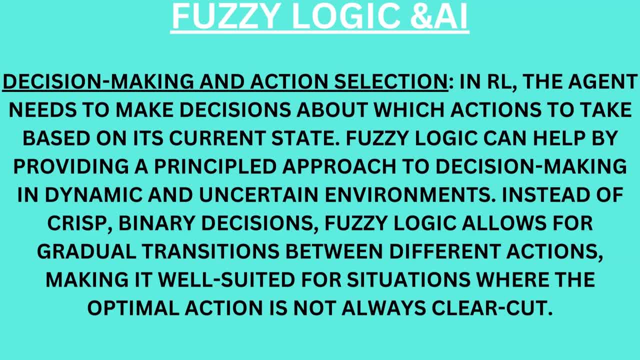 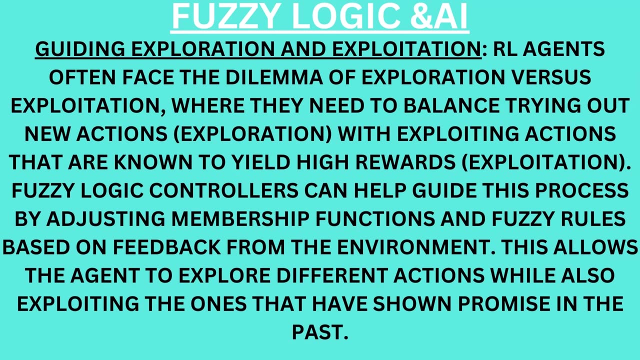 Fuzzy logic can help by providing a principled approach to decision-making in dynamic and uncertain environments. Instead of CRI-SP binary decisions, fuzzy logic allows for gradual transitions between different actions, making it well-suited for situations where the optimal action is not always clear-cut Guiding and 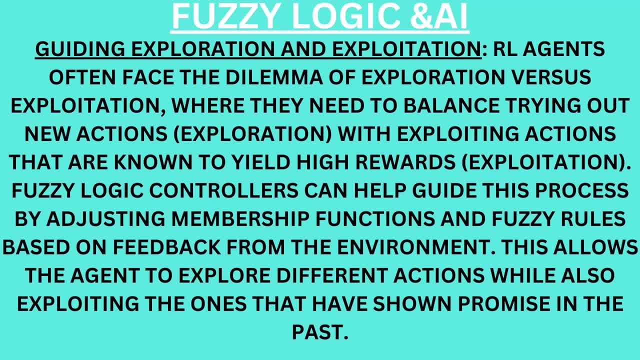 interesting temporal state evaluation. The agents Abendler, Mitchellיד Greg, Exploration, E&想ř lesson and exploitation: Damn ProNothing for his face. the dilemma off exploration well, versus exploitation- weird, they need to bail- is trying out New Actions, Exploration with exploiting actions that are known to yield. 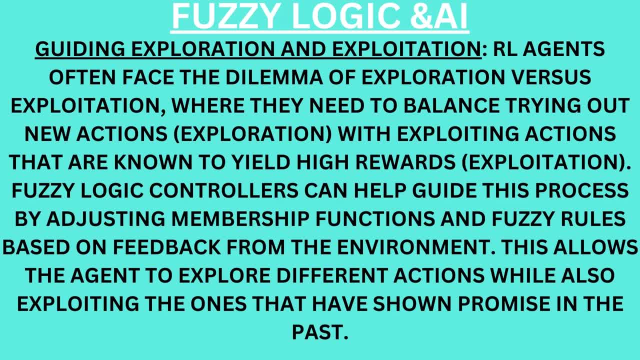 Hey rewards exploitation. pussy logic controllers can help guide this process By adjusting membership functions. an Fuzzy rules based on就需要ss用光l benii stingh, based on feedback from the environment. This allows the agent to explore different actions. 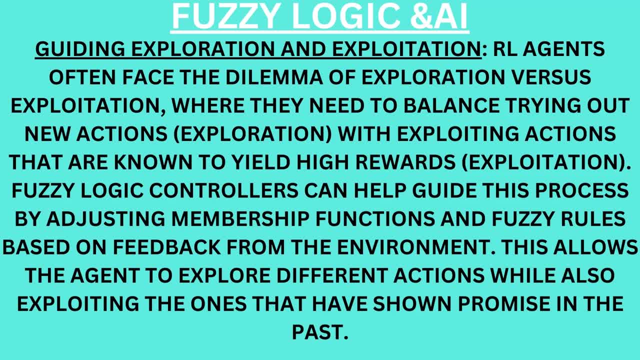 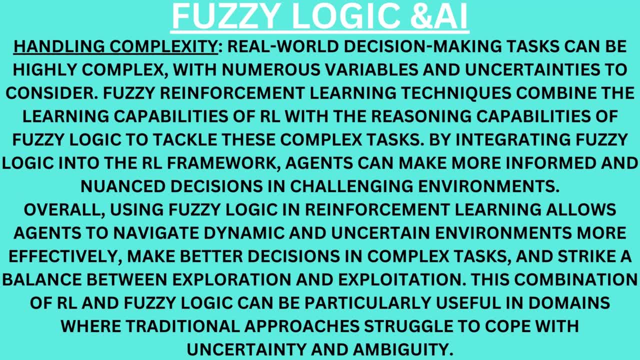 while also exploiting the ones that have shown promise in the past. Handling Complexity. Real-world decision-making tasks can be highly complex, with numerous variables and uncertainties to consider. Fuzzy reinforcement learning techniques combine the learning capabilities of reinforcement learning with the reasoning capabilities of fuzzy logic to tackle these complex tasks By integrating fuzzy logic. 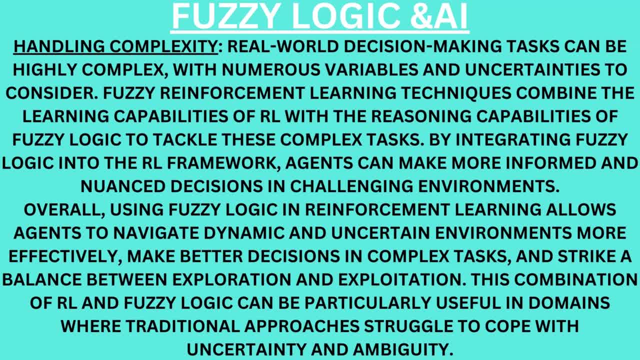 into the reinforcement learning framework. agents can make more informed and nuanced decisions in challenging environments. Overall, using fuzzy logic in reinforcement learning allows agents to navigate dynamic and uncertain environments more effectively, Make better decisions in complex tasks and strike a balance between exploration and exploitation. 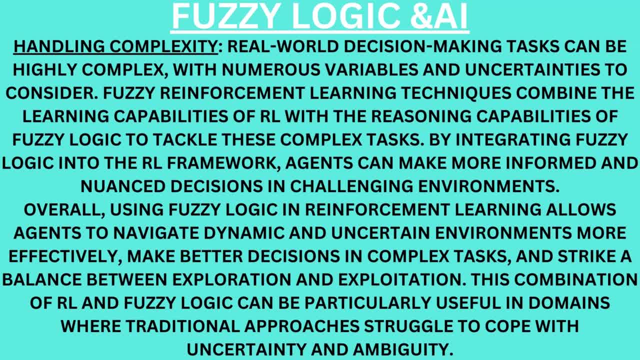 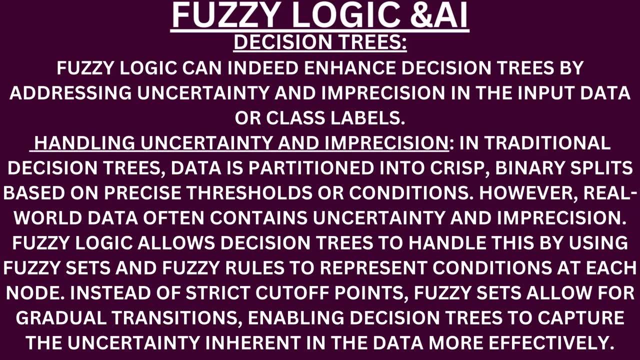 This combination of reinforcement learning and fuzzy logic can be particularly useful in domains where traditional approaches struggle to cope with uncertainty and ambiguity Decientries. Fuzzy logic can indeed enhance deceitful decisions by addressing uncertainty and imprecision. In the event that an agent falls, the decision maker can take any action in which the agent 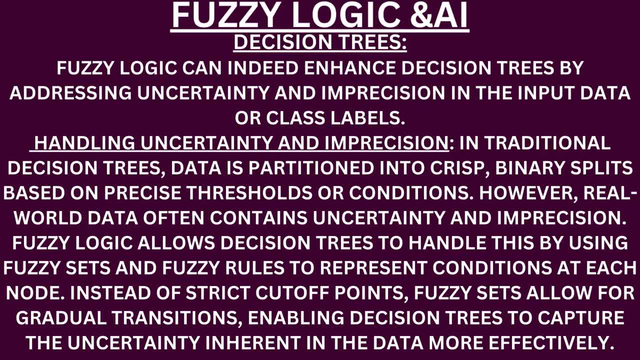 input data or class labels. handling uncertainty and impression. In traditional decision trees, data is partitioned into crisp binary splits based on precise thresholds or conditions. However, real world data often contains uncertainty and impression. Fuzzy logic allows decision trees to handle this by using fuzzy sets and fuzzy rules to represent conditions at each. 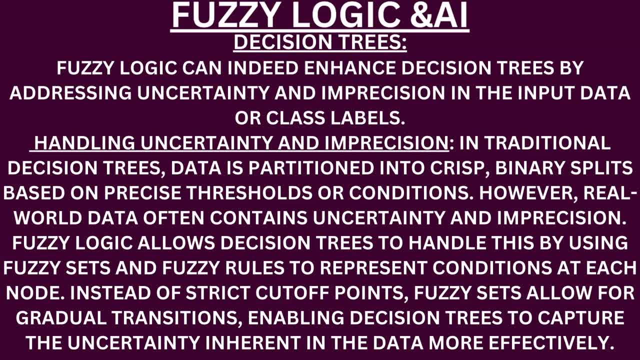 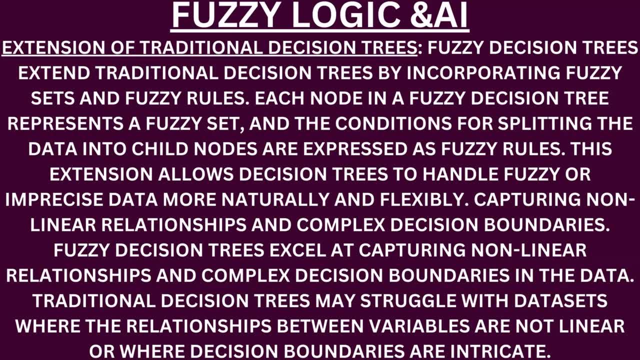 node. Instead of strict cut-off points, fuzzy sets allow for gradual transitions, enabling decision trees to capture the uncertainty inherent in the data more effectively. Extension of traditional decision trees. Fuzzy decision trees extend traditional decision trees by incorporating fuzzy sets and fuzzy rules. Each node in a fuzzy decision tree represents 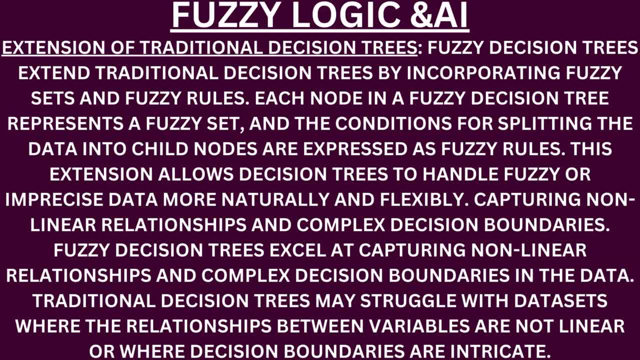 a fuzzy set and the conditions for splitting the data into child nodes are expressed as fuzzy rules. This extension allows decision trees to handle fuzzy or imprecise data more naturally and flexibly, Capturing non-linear relationships and complex decision boundaries. Fuzzy decision tree excel at capturing non-linear relationships and complex decision boundaries. 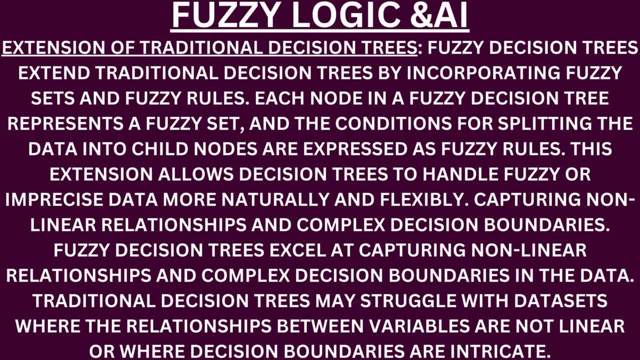 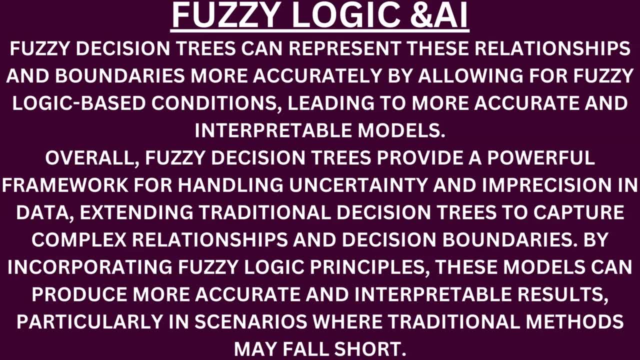 in the data. Traditional decision trees may struggle with data sets where the relationships between variables are not linear or where decision boundaries are intricate. Fuzzy decision trees can represent non-linear relationships and complex decision boundaries. these relationships and boundaries more accurately by allowing for fuzzy logic. 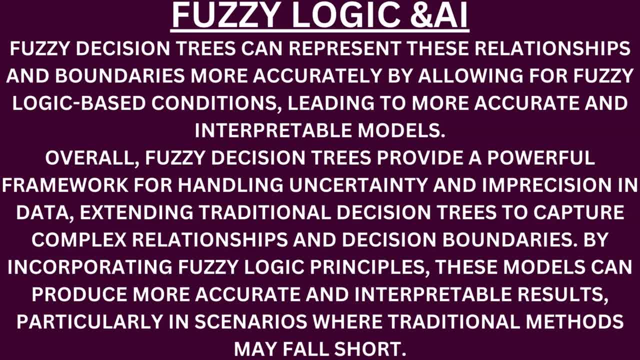 based conditions, leading to more accurate and interpretable models. overall, fuzzy decision trees provide a powerful framework for handling uncertainty and imprecision in data, extending traditional decision trees to capture complex relationships and decision boundaries. by incorporating fuzzy logic principles, these models can produce more accurate and interpretable results. 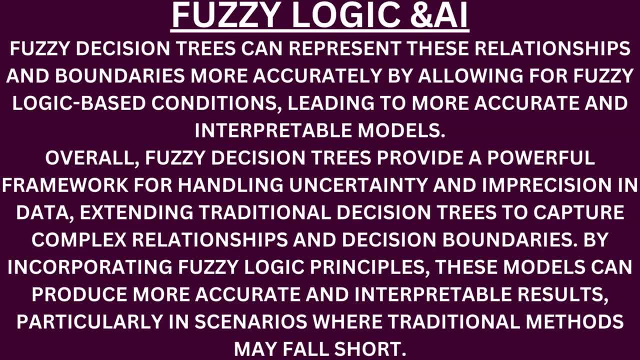 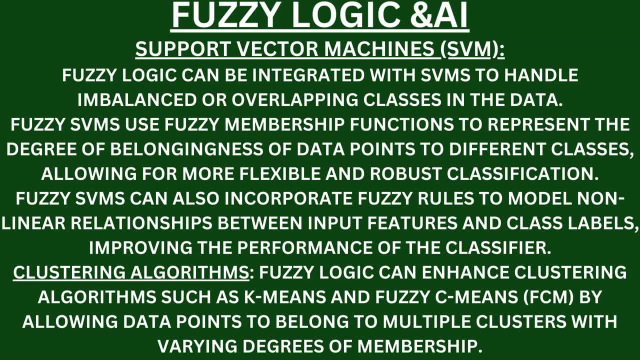 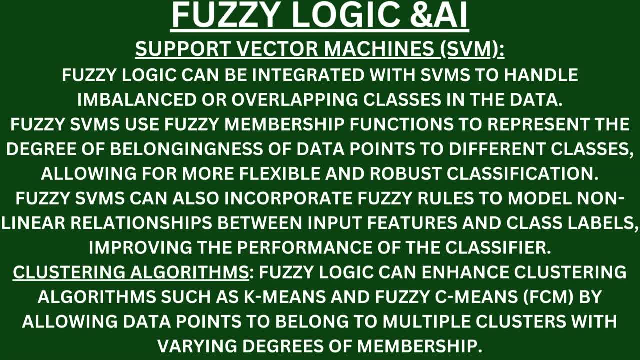 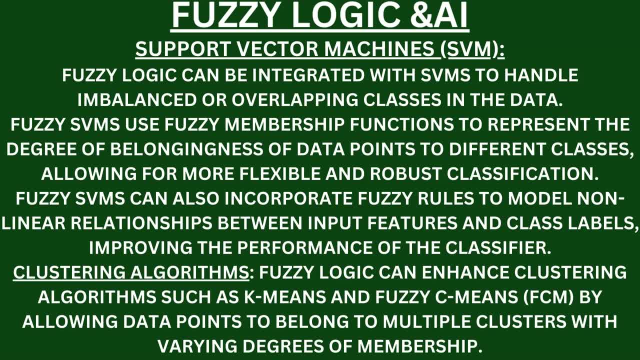 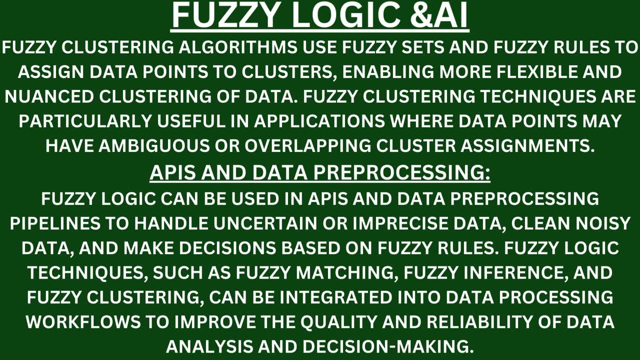 logic can enhance clustering algorithms- suck as K means and fuzzy C means FCM- by allowing data points to belong to multiple clusters with varying degrees of membership. fuzzy clustering algorithms use fuzzy sets and fuzzy rules to assign data points to clusters, enabling more flexible and nuanced clustering of data. 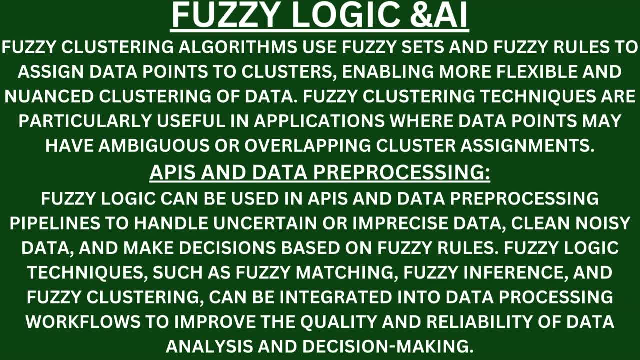 fuzzy clustering techniques are particularly useful in applications where data points may have ambiguous or overlapping cluster assignments. if you are using a trafficify argumentblank, So in order to make a policy holder where we use CAD to ignore impact uncertainty among ELD bot and when we open. 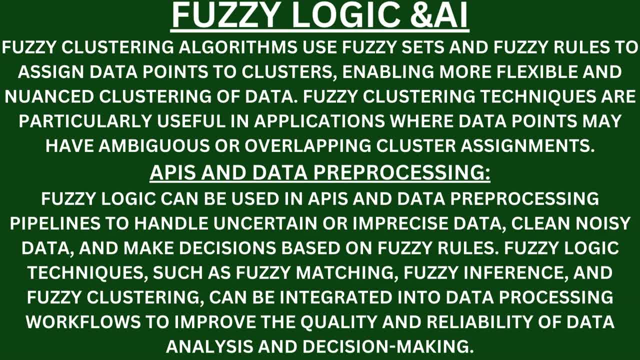 няwer to open 04 d0 40 or a true function rather than capture unique stakeholders for that function, be distinguished sin data to set our interface to execute data delivery. but we do not know the answer, as different functions allowing us to use fuzzing software in different deb, jewett fields, api's and database processing. fuzzy logic can be used in api's and data pre processing pipelines to handle uncertain or in precise data, clean, noisy data and me perceives based on fuzzy rules. fuzzy logic techniques such as for cm actually and APRIM data processing workflows to improve the quality and reliability of data analysis and- and this continues- for DB Davis is a very important point here. 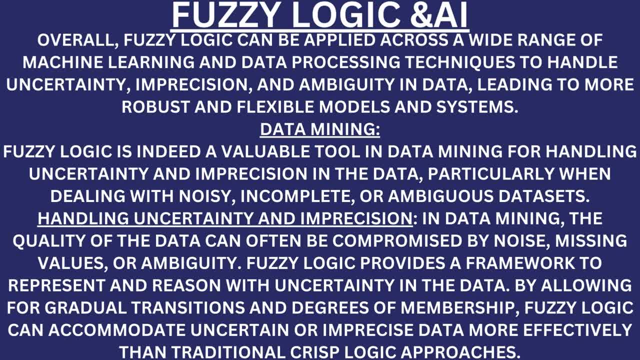 and decision-making Overall. fuzzy logic can be applied across a wide range of machine learning and data processing techniques to handle uncertainty, imprecision and ambiguity in data, leading to more robust and flexible models and systems. Data mining Fuzzy logic is indeed a. 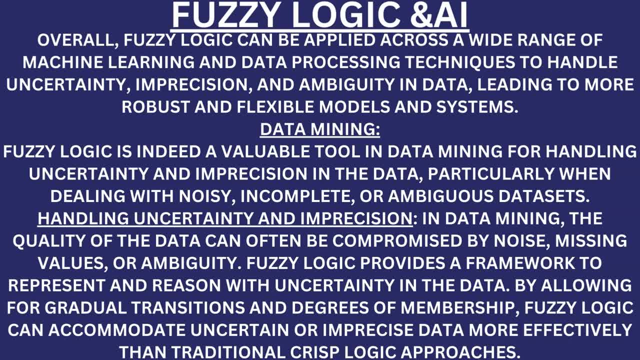 valuable tool in data mining for handling uncertainty and imprecision in the data, particularly when dealing with noisy, incomplete or ambiguous datasets. Handling uncertainty and imprecision in data mining. the quality of the data can often be compromised by noise, missing values or ambiguity. Fuzzy logic provides a framework to represent and reason. 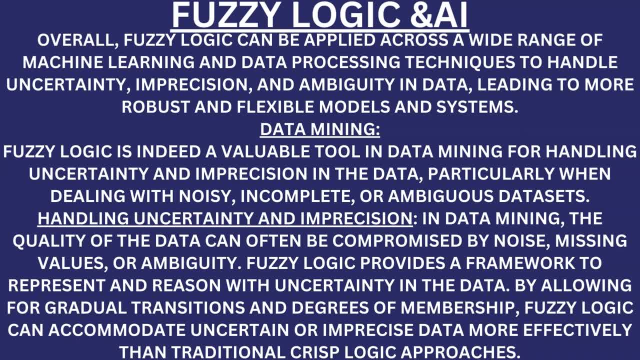 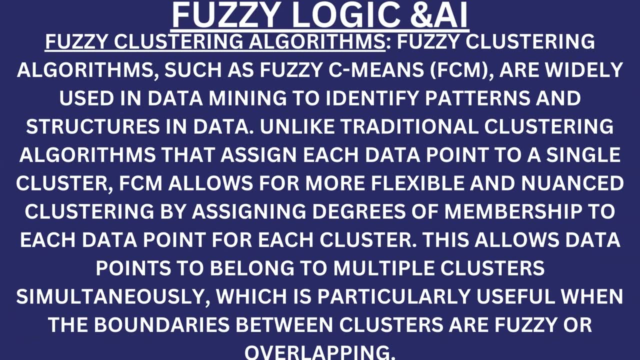 with uncertainty in the data by allowing for gradual transitions and degrees of membership. Fuzzy logic can accomplish this. Fuzzy clustering algorithms. Fuzzy clustering algorithms such as fuzzy C-means, FCM, are widely used in data mining to identify patterns. 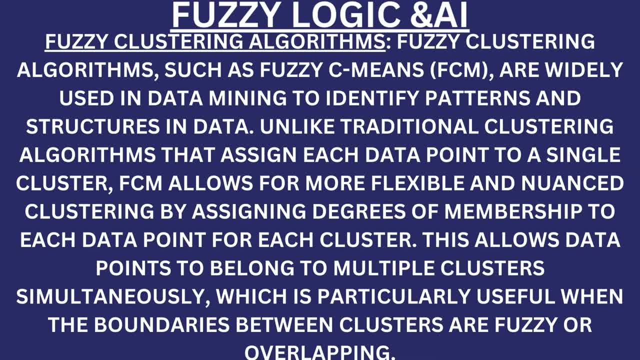 and structures in data. unlike traditional clustering algorithms that assign each data point to a single cluster, FCM allows for more flexible and nuanced clustering by assigning ž degrees of membership to each data point for each cluster. This allows data points to belong to multiple clusters simultaneously, which is particularly useful when the boundaries between 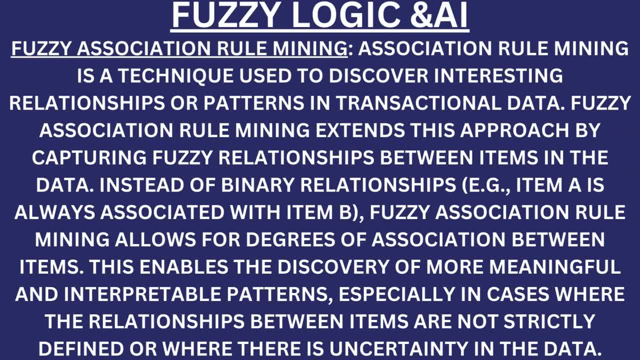 clusters are fuzzy or overlapping. Fuzzy association rule mining. Association rule mining is a technique used to discover interesting relationships or patterns in transactional data. Fuzzy association rule mining extends this approach by capturing fuzzy relationships between items in the data Instead of binary relationships. that is, item A is always associated. 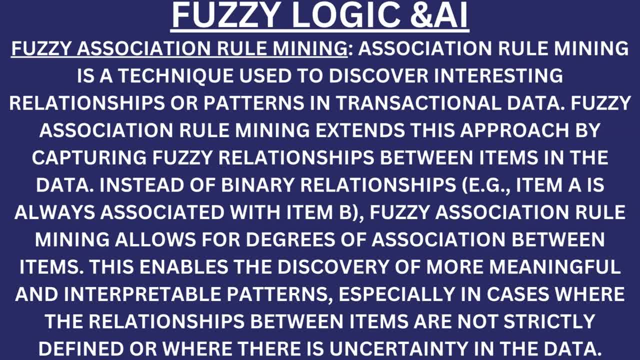 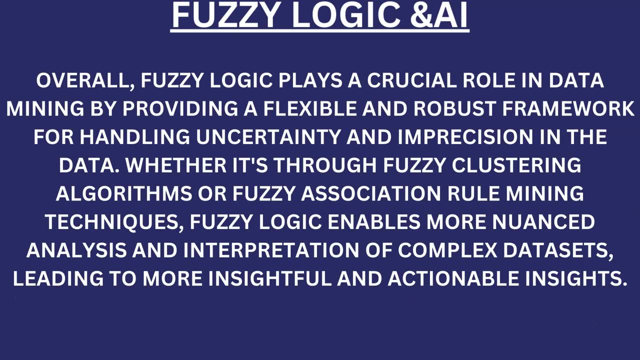 with item B. fuzzy association rule mining allows for degrees of association between items. This enables the discovery of more meaningful and interpretable patterns, especially in cases where the relationship between the items is not so good. Fuzzy logic plays a crucial role in data mining by providing a flexible and robust framework. 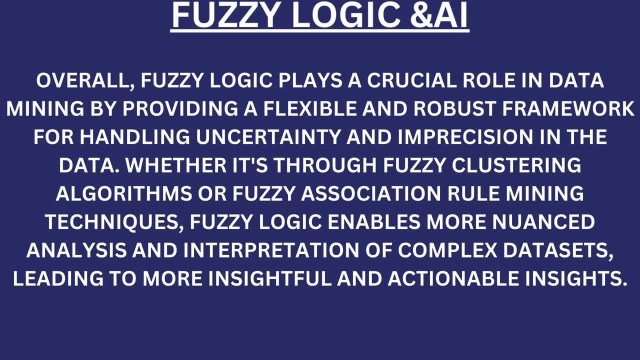 for handling uncertainty and imprecision in the data, Whether it's through fuzzy clustering algorithms or fuzzy association rule mining techniques. fuzzy logic enables more nuanced analysis and interpretation. Fuzzy logic can also be used to analyze complex data sets, leading to more insightful and 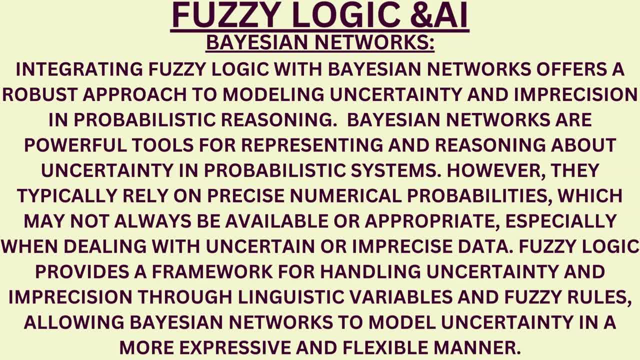 actionable insights. Bayesian networks. Integrating fuzzy logic with Bayesian networks offers a robust approach to modeling uncertainty and imprecision in probabilistic reasoning. Bayesian networks are powerful tools for representing and reasoning about uncertainty in probabilistic systems. However, they typically rely on precision. 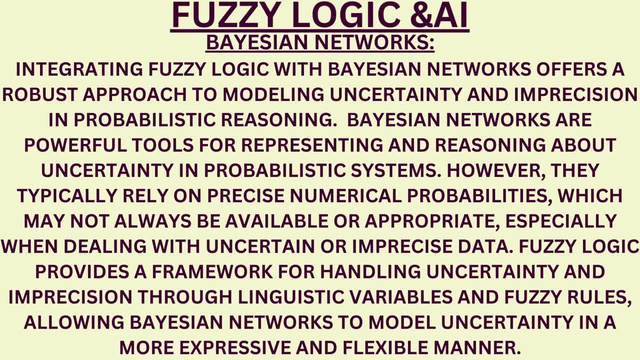 Fuzzy logic can be used to understand or measure uncertainty and imprecise numerical probabilities, which may not always be available or appropriate, especially when dealing with uncertain or implicit data. Fuzzy logic provides a framework for handling uncertainty and imprecision through linguistic variables and fuzzy rules, allowing Bayesian networks to model uncertainty in a more 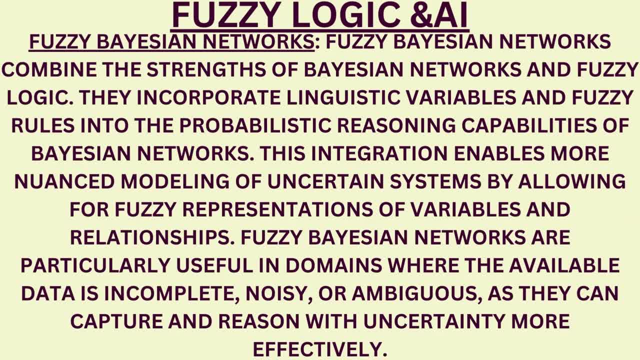 expressive and flexible manner. Fuzzy Bayesian networks. Fuzzy Bayesian networks: combine the Internet of Things to model uncertainty and implicit data. Combine the strengths of Bayesian networks and fuzzy logic. They incorporate linguistic variables and fuzzy rules into the probabilistic reasoning capabilities of Bayesian networks. 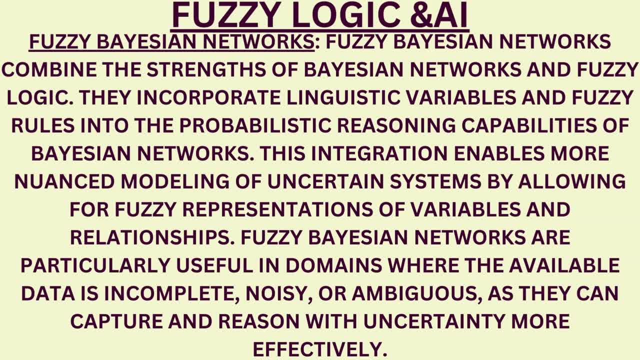 This integration enables more nuanced modeling of uncertain systems by allowing for fuzzy representations of variables and relationships. Fuzzy Bayesian networks are particularly useful in domains where the available data is incomplete, noisy or ambiguous, as they can capture and reason with uncertainty more effectively, Handling uncertain or imprecise evidence: Fuzzy. 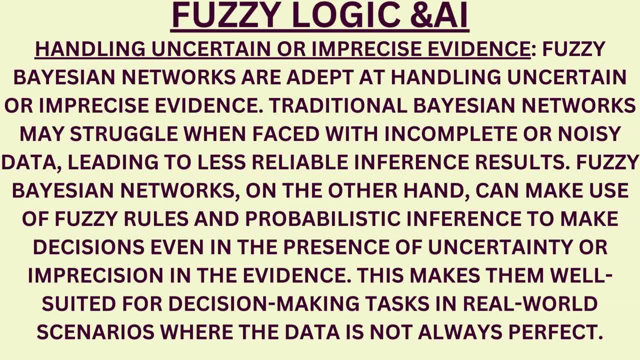 Bayesian networks are adept at handling uncertain or imprecise evidence. Traditional Bayesian networks may struggle when faced with incomplete or noisy data, leading to less reliable inference treatments results. fuzzy bayesian networks, on the other hand, can make use of fuzzy rules and probabilistic 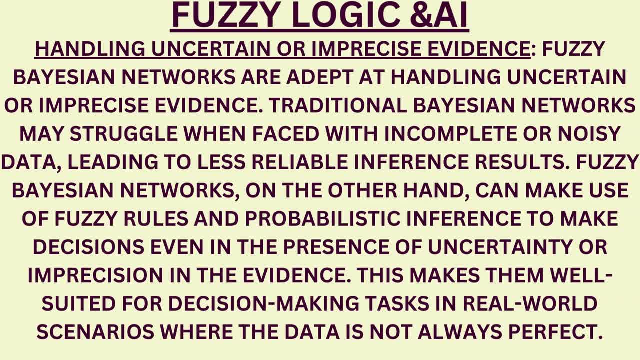 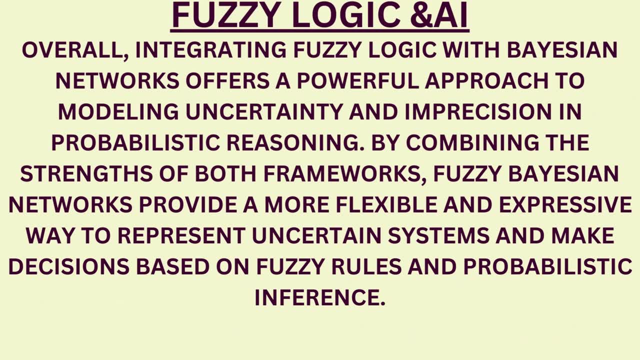 inference to make decisions even in the presence of uncertainty or impression in the evidence. this makes them well suited for decision making tasks in real world scenarios where the data is not always perfect. overall, integrating fuzzy logic with bayesian networks offers a powerful approach to modeling uncertainty and impression in probabilistic reasoning by combining the 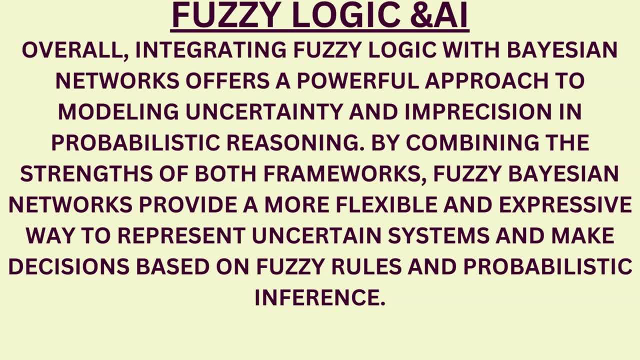 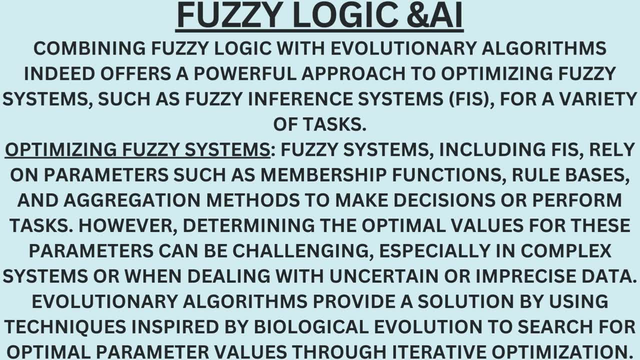 strengths of both frameworks. fuzzy bayesian networks provide a more flexible and expressive way to represent uncertain systems and make decisions based on fuzzy rules and probabilistic inference. combining fuzzy logic with evolutionary algorithms indeed offers a powerful approach to optimizing fuzzy systems, such as fuzzy inference systems, fis, for a variety of tasks optimizing fuzzy systems. fuzzy systems, including fis, rely on: 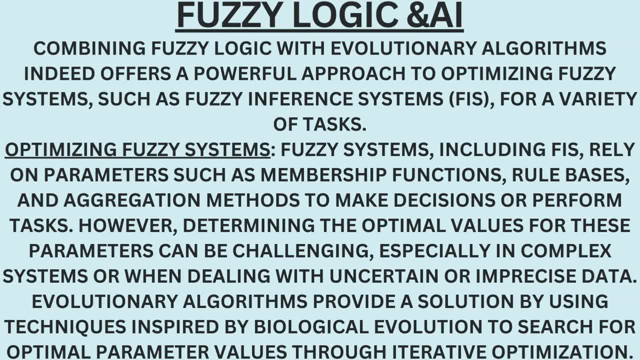 parameters such as membership, functions, rule bases and aggregation methods to make decisions or perform tasks. however, determining the optimal values for these parameters can be challenging, especially in complex systems or when dealing with uncertain or imprecise data. evolutionary algorithms provide a solution by using techniques inspired by biological evaluation. 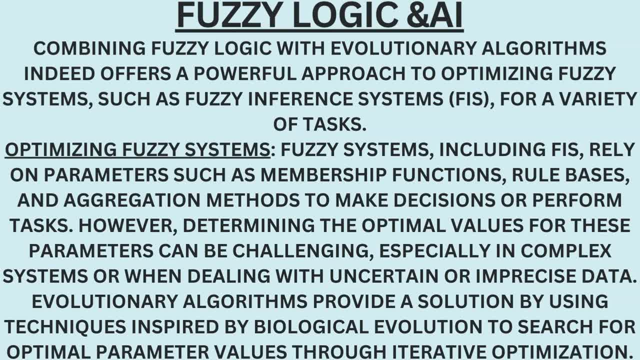 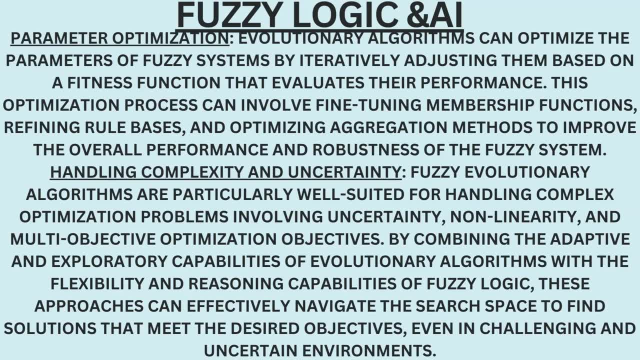 evolution to search for optimal parameter values through iterative optimization. parameter optimization: evolutionary algorithms can optimize the parameters of fuzzy systems by iteratively adjusting them based on a fitness function that evaluates their performance. this optimization process can involve fine-tuning membership functions, refining rule-based and optimizing aggregation methods to improve the overall performance and robustness of the fuzzy system, handling complexity and uncertainty. 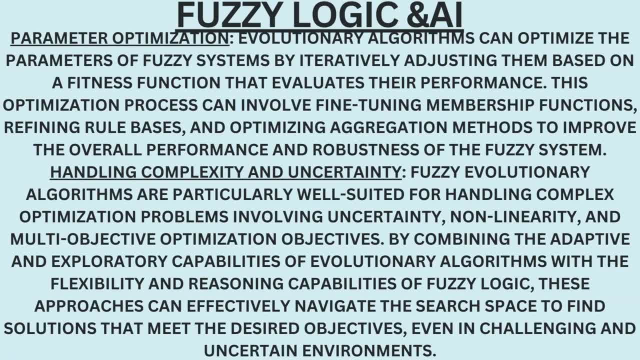 Fuzzy evolutionary algorithms are particularly well suited for handling complex optimization problems involving uncertainty, non-linearity and multi-objective optimization objectives. By combining the adaptive and exploratory capabilities of evolutionary algorithms with the flexibility and reasoning capabilities of fuzzy logic, these approaches can effectively navigate the search space to find solutions that meet the desired objectives, even in challenging and uncertain environments. 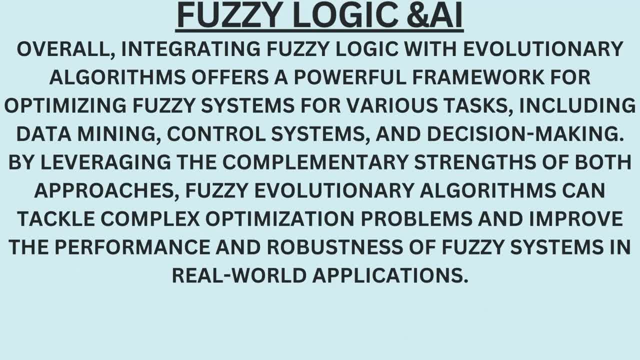 Overall, integrating fuzzy logic with evolutionary algorithms offers A powerful framework for optimizing fuzzy logic. Fuzzy logic provides fuzzy systems for various tasks, including data mining, control systems and decision-making. By leveraging the complementary strengths of both approaches, fuzzy evolutionary algorithms can tackle complex optimization problems and improve the performance and robustness of fuzzy systems in real-world applications. 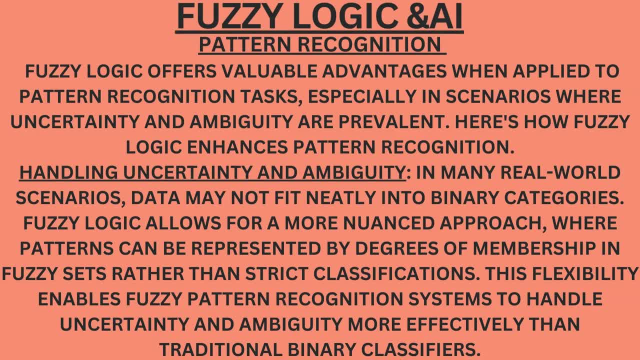 Fuzzy logic offers valuable advantages when applied to pattern recognition tasks. Fuzzy logic can be used in several scenarios where uncertainty and ambiguity are prevalent: Handling uncertainty and ambiguity. In many real-world scenarios, data may not fit neatly into binary categories. Fuzzy logic allows for a more nuanced approach where patterns can be represented by degrees of membership in fuzzy sets rather than strict classifications. 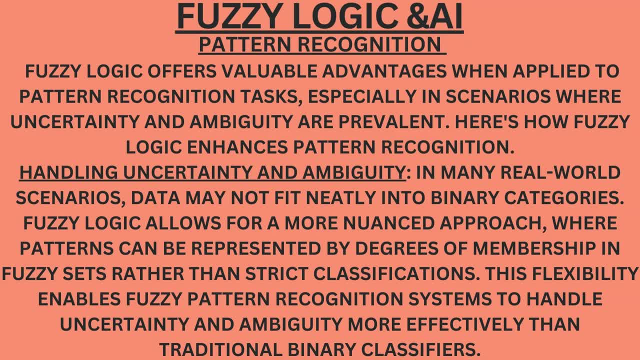 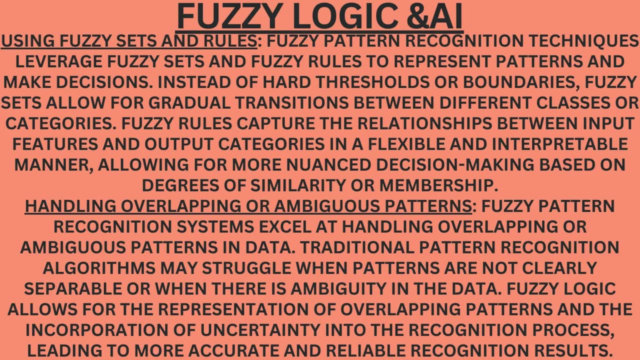 This flexibility enables fuzzy pattern recognition systems to handle uncertainty and ambiguity more effectively than traditional binary classifiers Using fuzzy sets and rules. fuzzy pattern recognition techniques leverage fuzzy sets and fuzzy rules to represent patterns and make decisions. Instead of hard thresholds or boundaries, fuzzy sets allow for gradual transitions between different classes or categories. 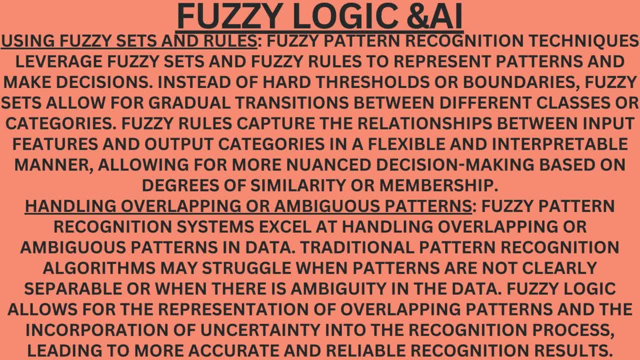 Fuzzy rules capture the relationships between input features and output categories in a flexible and interpretable manner, allowing for more nuanced decision-making based on degrees of similarity or membership. Handbook: Handling Overlapping or Ambiguous Patterns. Fuzzy pattern recognition systems excel at handling overlapping or ambiguous patterns in data. 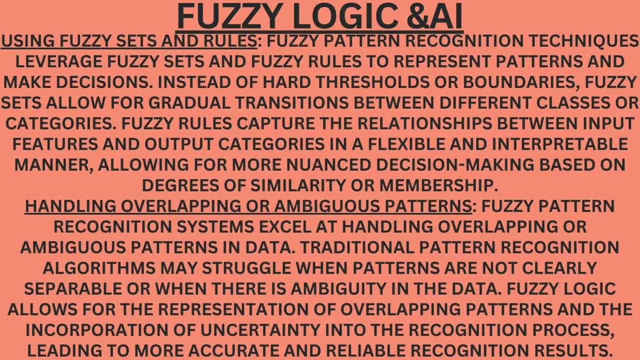 Traditional pattern recognition algorithms may struggle when patterns are not clearly separable or when there is ambiguity in the data. Fuzzy logic allows for the representation of overlapping patterns and the incorporation of patterns. Fuzzy logic allows for the representation of uncertainty into the recognition process, leading to more accurate and reliable recognition results. 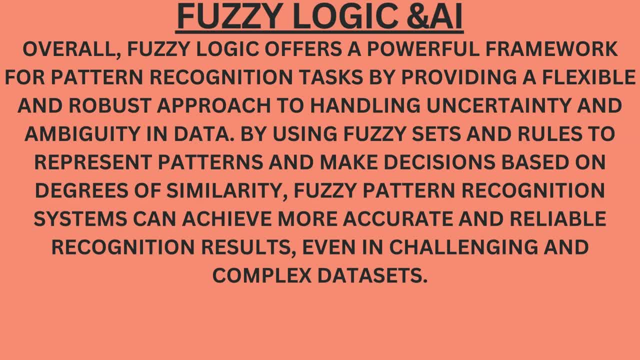 Overall, fuzzy logic offers a powerful framework for pattern recognition tasks by providing a flexible and robust approach to handling uncertainty and ambiguity in data. by using fuzzy sets and rules to represent patterns and make decisions based on degrees of similarity, Fuzzy pattern recognition systems can achieve more accurate and reliable recognition results, even in challenging and complex data sets. 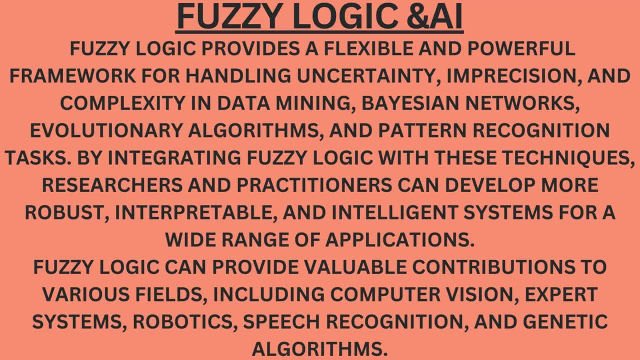 Fuzzy logic provides a flexible and powerful framework for handling uncertainty and complexity in data mining, Bayesian networks, evolutionary algorithms and pattern recognition tasks. By integrating fuzzy logic with these techniques. With these techniques, researchers and practitioners can develop more robust, interpretable and intelligent systems for a wide range of applications. 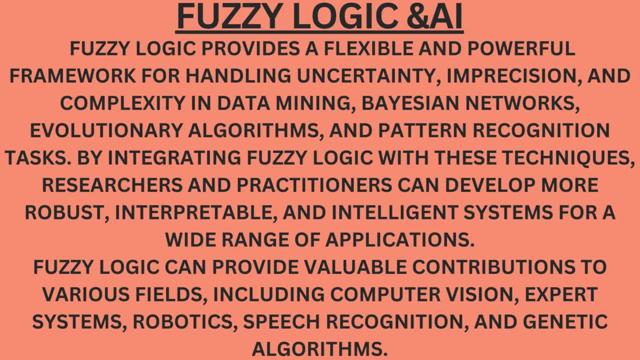 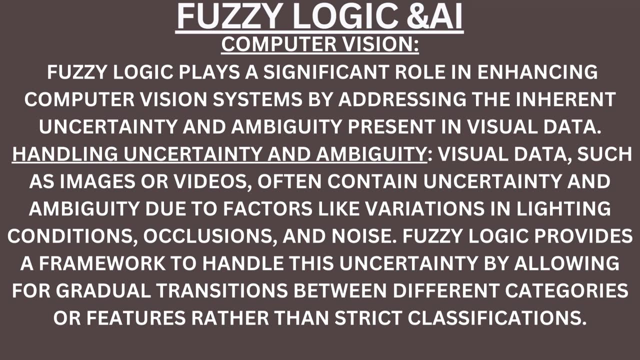 Fuzzy logic can provide valuable contributions to various fields, including computer VN expert systems, robotics, speech recognition and genetic algorithms. Computer VN Fuzzy logic plays a significant role in enhancing computer VN systems by addressing the inherent uncertainty and ambiguity present in visual data. 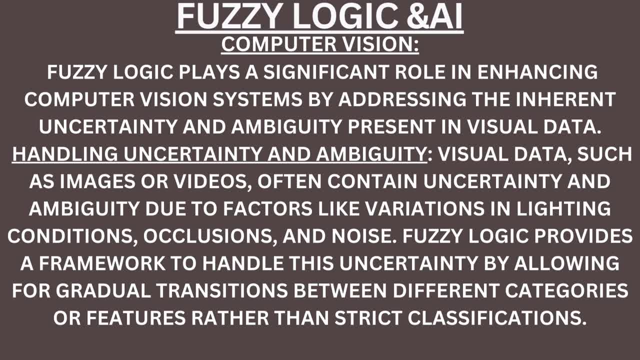 Handling uncertainty and ambiguity. Visual data, such as images or videos, often contain uncertainty and ambiguity due to factors like variations in lighting conditions, occlusions and noise. Fuzzy logic provides a framework to handle this uncertainty by allowing for gradual transitions between different categories or features, rather than strict classifications. 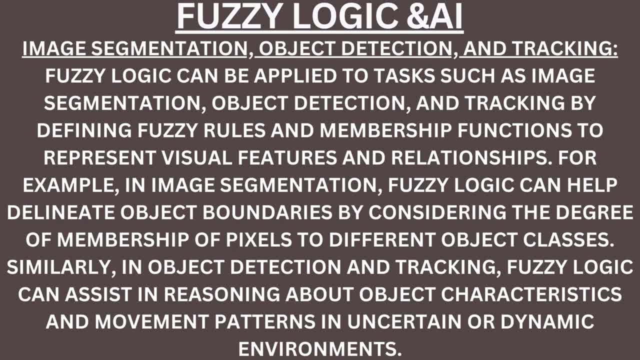 Image segmentation, object detection and tracking. Fuzzy logic can be applied to tasks such as image segmentation, object detection and tracking by defining fuzzy rules and membership functions to represent visual features and relationships. For example, in image segmentation, fuzzy logic can help delineate object boundaries by considering the degree of membership of pixels to different object classes. 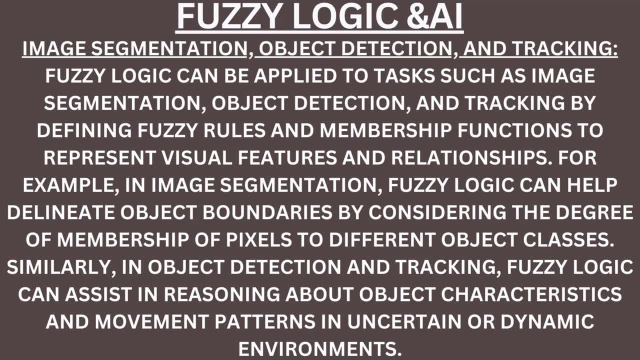 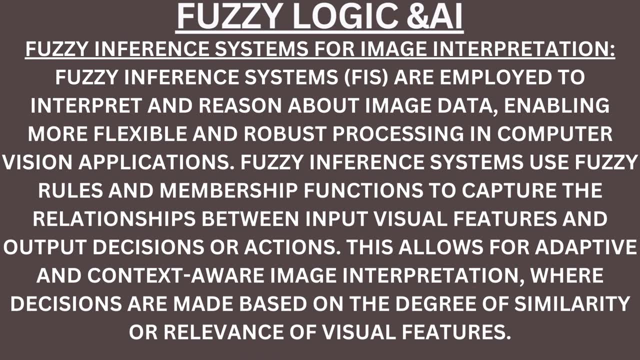 Similarly in object detection and tracking. fuzzy logic can assist in reasoning about object characteristics and movement patterns in uncertain or dynamic environments. Fuzzy inference systems for image interpretation. Fuzzy inference systems for image interpretation. Fuzzy inference systems, FIS, are employed to interpret and reason about image data, enabling more flexible and robust processing in computer. VN applications. 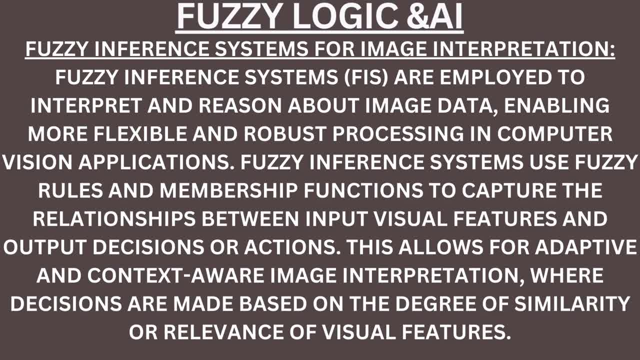 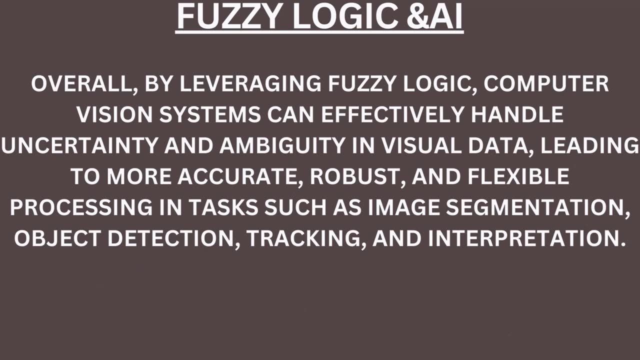 Fuzzy inference systems use fuzzy rules and membership functions to capture the relationships between input visual features and output decisions or actions. This allows for adaptive and context-aware image interpretation, where decisions are made based on the degree of similarity or relevance of visual features. Overall, by leveraging fuzzy logic, computer VN systems can effectively handle uncertainty and ambiguity in visual data. 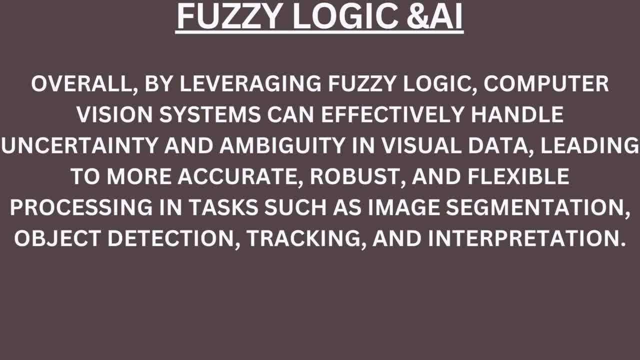 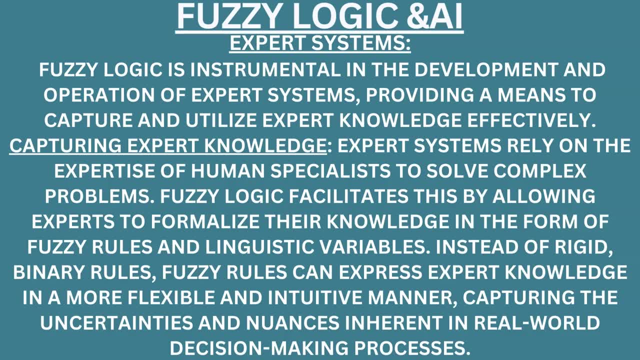 leading to more accurate, robust and flexible processing in tasks such as image segmentation, object detection, tracking and interpretation. Fuzzy logic is instrumental in the development and operation of expert systems, providing a means to capture and utilize expert knowledge effectively. Capturing expert knowledge: expert systems rely on the expertise of human specialists to solve complex problems. 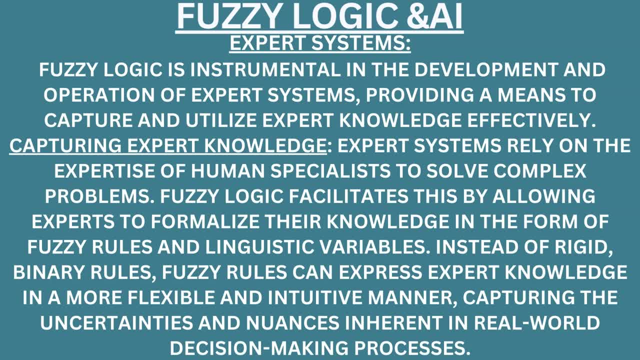 Fuzzy logic facilitates this by allowing experts to formalize their knowledge in the form of fuzzy rules and linguistics variables. Instead of rigid binary rules, fuzzy rules can express expert knowledge in a more flexible and intuitive manner, capturing the uncertainties and nuances inherent in real-world decision-making processes. 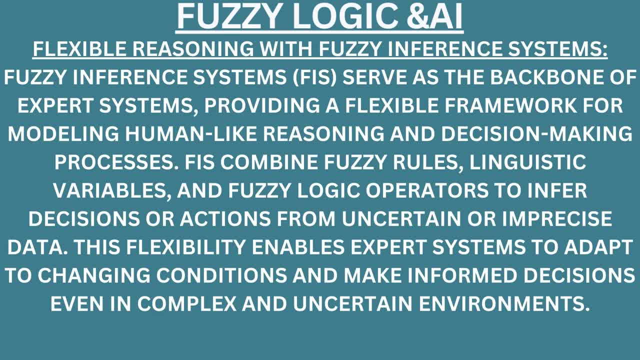 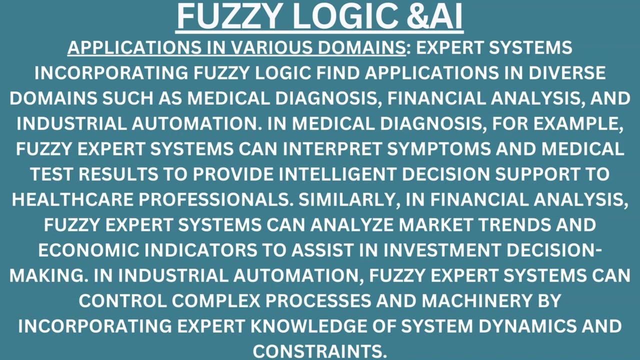 Flexible reasoning with fuzzy inference systems. Fuzzy inference systems serve as the backbone of expert systems, providing a flexible framework for monitoring and processing. Fuzzy inference systems use both remembered and complete research proof and data. Fuzzy inference systems create complex calculations and a flexible protocol for solving complex. 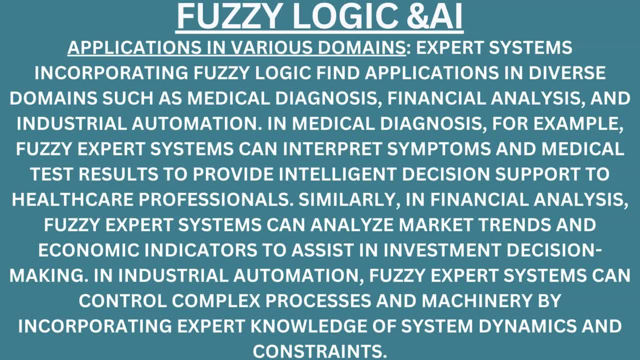 and hp-based problems Domains. Expert systems incorporating fuzzy logic find applications in diverse domains, such as medical diagnosis, financial analysis and industrial automation. In medical diagnosis, for example, fuzzy expert systems can interpret symptoms and medical test results to provide intelligent decision support to healthcare professionals. Similarly, in financial analysis, 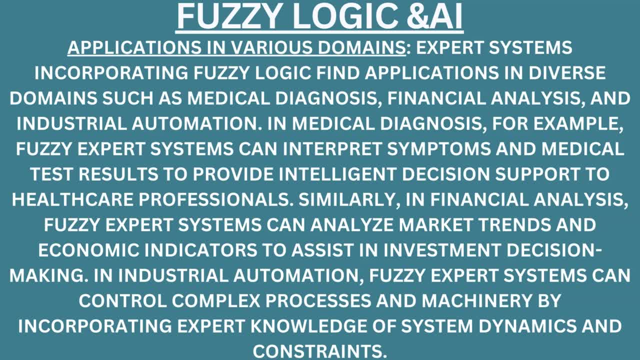 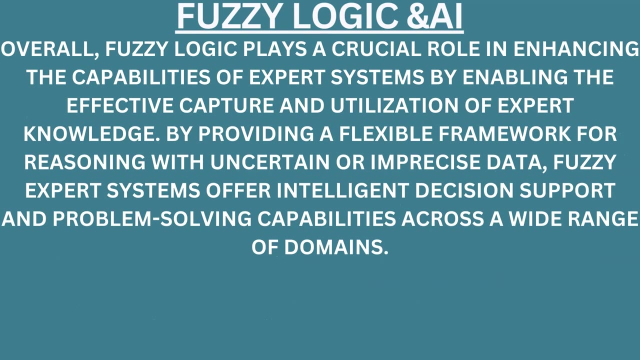 fuzzy expert systems can analyze market trends and economic indicators to assist in investment decision-making In industrial automation, fuzzy expert systems can control complex processes and machinery by incorporating expert knowledge of system dynamics and constraints. Overall, fuzzy logic plays a crucial role in enhancing the capabilities of expert systems. 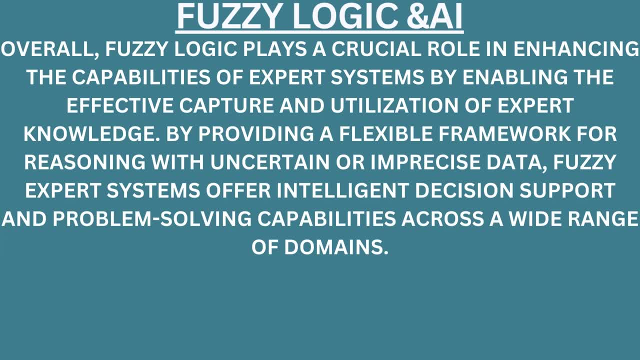 by enabling them to do the work that they need to do. Effective capture and utilization of expert knowledge by providing a flexible framework for reasoning with uncertain or emphasized data. fuzzy expert systems offer intelligent decision support and problem-solving capabilities across a wide range of domains. 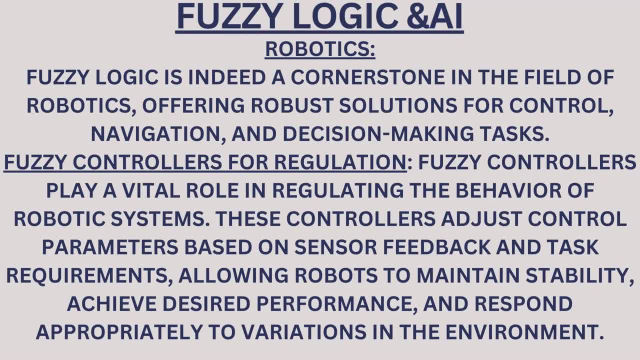 Robotics. Fuzzy logic is indeed a cornerstone in the field of robotics, offering robust solutions for control, navigation and decision-making tasks. Fuzzy controllers for regulation: Fuzzy controllers play a vital role in regulating the behavior of robotic systems. These controllers adjust control parameters based on sensor feedback. 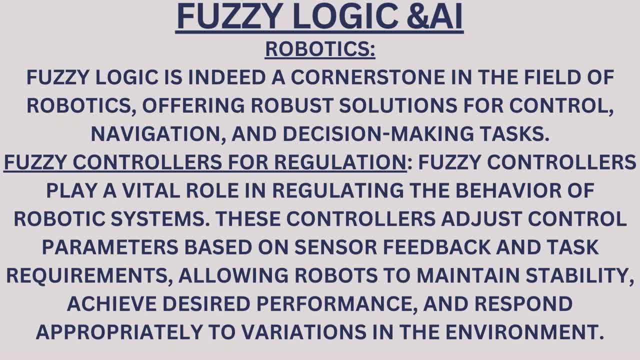 and task requirements allowing robots to maintain stability, achieve desired performance and respond appropriately to variations in the environment. Fuzzy control is particularly useful in situations of emergency. Fuzzy control is particularly useful in situations of emergency. Fuzzy control is particularly useful in situations of emergency. Fuzzy control is particularly useful. 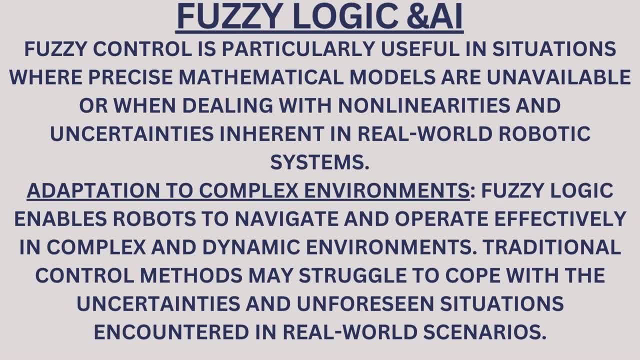 in situations where precise mathematical models are unavailable or when dealing with non-linearities and uncertainties inherent in real-world robotic systems. Adaptation to complex environments: Fuzzy logic enables robots to navigate and operate effectively in complex and dynamic environments. Traditional control methods may struggle to cope with the uncertainties and unforeseen아서им controls between robots and reactor making professionals and experts can Alors فصل لجمعoles تصمم اكرامل شركات welt کی تحقق بال د ballots stacked على م~. Fuzzy logic enables robots to specifically play an important role in Java application calculations. environment على conserve. لا تی eldestبths الع lider استثقائم وISHA و AM RUSSIA semaines لoopuvosociOOO Data owner 가atreحذój ماذ peaks designation alla pensa verrحمنHay. no HAMBY sucked by difficult to account a reward. 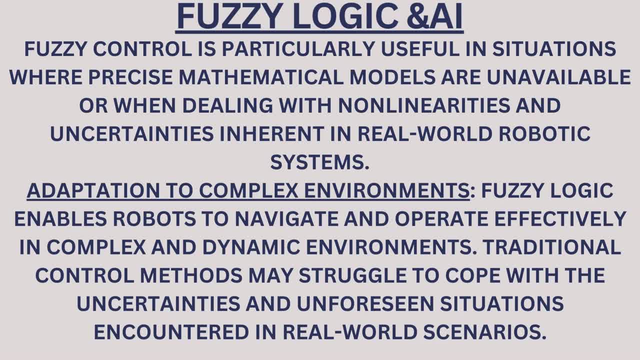 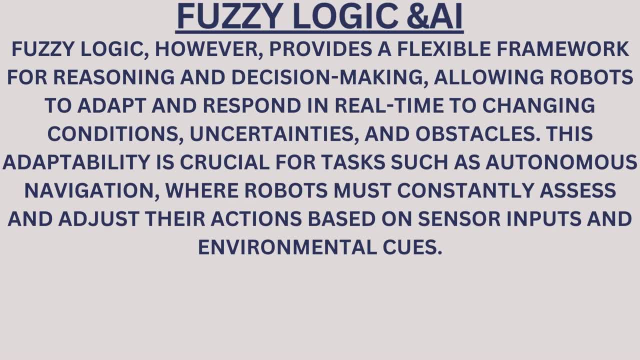 situations encountered in real world scenarios. fuzzy logic, however, provides a flexible framework for reasoning and decision making, allowing robots to adapt and respond in real time to changing conditions, uncertainties and obstacles. this adaptability is crucial for tasks such as autonomous navigation, where robots must constantly assess and adjust their actions based on sensor. 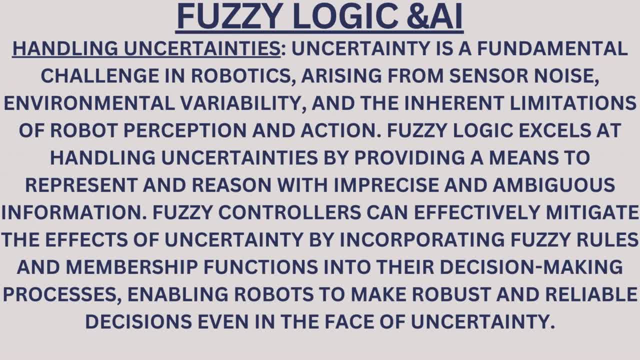 inputs and environmental cues. handling uncertainties. uncertain is a fundamental challenge in robotics arising from sensor noise, environmental variability and the inherent. effectively mitigate the effects of uncertainty by incorporating fuzzy rules and membership functions into their decision-making processes, enabling robots to make robust and reliable decisions even in the face of uncertainty. 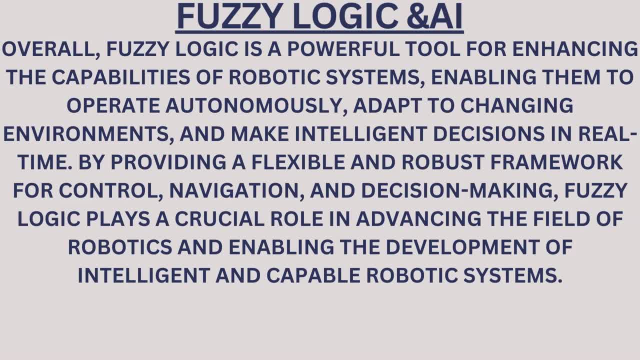 Overall, fuzzy logic is a powerful tool for enhancing the capabilities of robotic systems, enabling them to operate autonomously, adapt to changing environments and make intelligent decisions in real-time. By providing a flexible and robust framework for control, navigation and decision-making, fuzzy logic plays a crucial role in advancing the field of robotics and enabling the development. 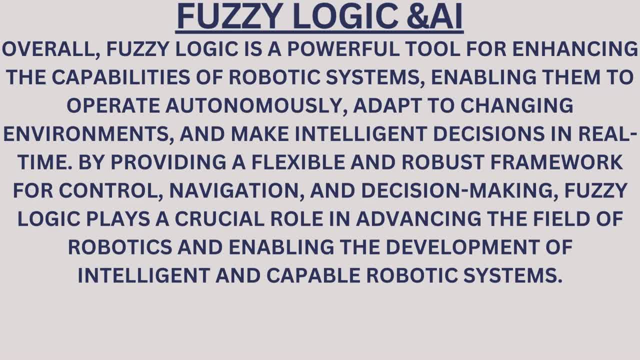 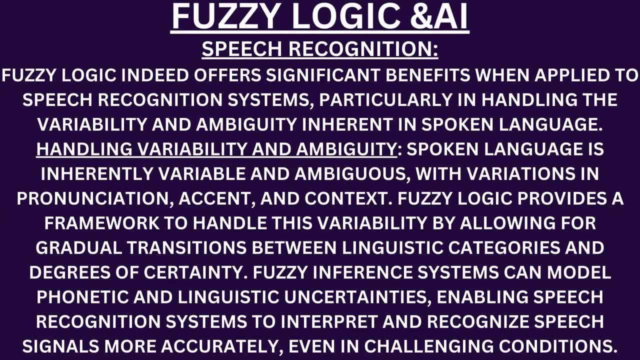 of intelligent and capable robotic systems. Speech Recognition- Fuzzy logic indeed offers significant benefits when applied to speech recognition systems, Particularly in handling the variability and ambiguity inherent in spoken language. Handling Variability and Ambiguity. Spoken language is inherently variable and ambiguous, with variations in pronunciation, accent and context. 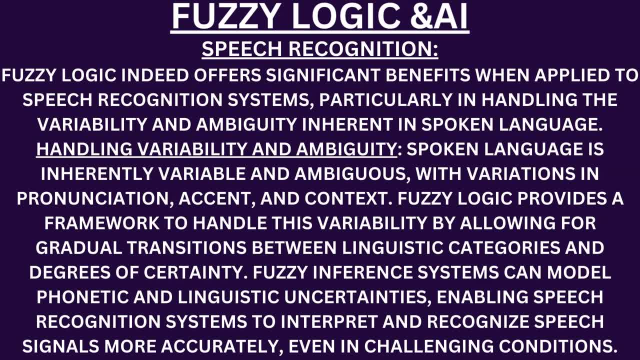 Fuzzy logic provides a framework to handle this variability by allowing for gradual transitions between linguistic categories and degrees of variability. Fuzzy inference systems can model phonetic and linguistic uncertainties, enabling speech recognition systems to interpret and recognize speech signals more accurately, even in challenging conditions. 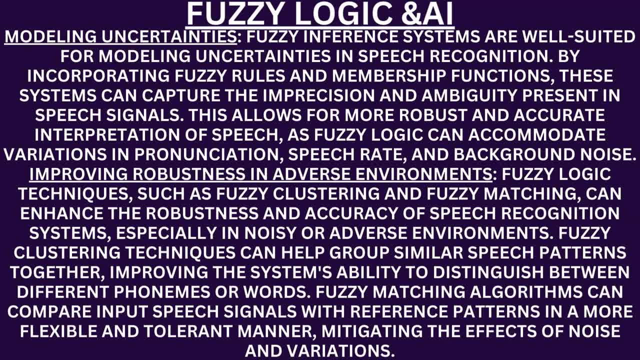 Modeling Uncertainties. Fuzzy inference systems are well-suited for modeling uncertainties in speech recognition. by incorporating fuzzy rules and membership functions, These systems can capture the imprecision and ambiguity present in speech signals. This allows for more robust and accurate interpretation of speech, as fuzzy logic can accommodate. 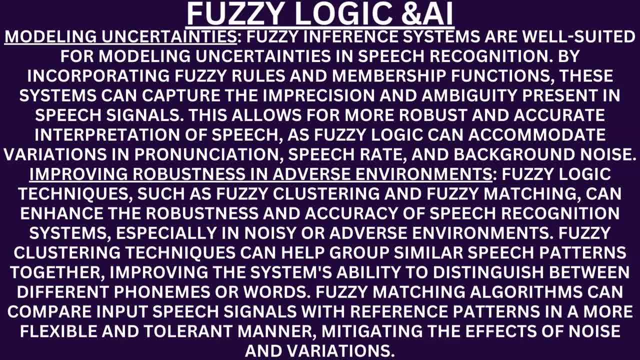 variations in pronunciation, speech rate and background noise. improving robustness in adverse environments. Fuzzy logic techniques such as fuzzy clustering and fuzzy matching can enhance the robustness and accuracy of speech recognition systems, especially in noisy or adverse environments. 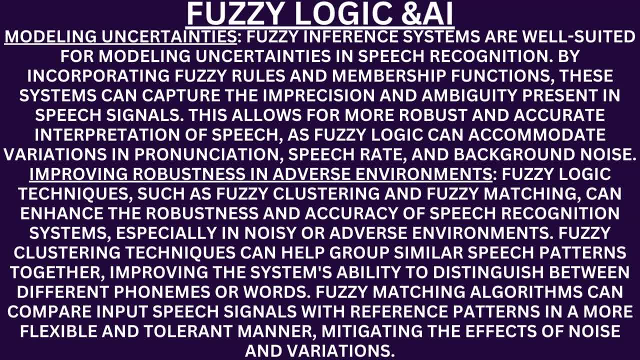 Fuzzy clustering techniques can help group similar speech patterns together, improving the system's ability to distinguish between different phenomena or words. Fuzzy matching algorithms can compare input speech signals or input signals to different phonetic patterns. Fuzzy matching algorithms can compare input speech signals or input speech patterns. 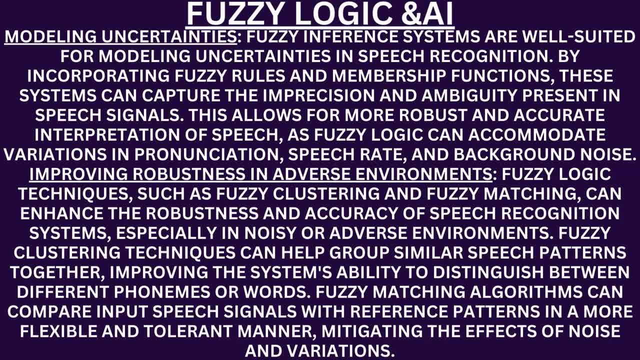 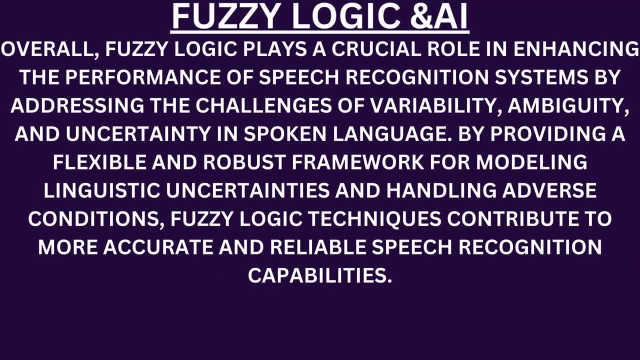 to different phonetic patterns with reference patterns in a more flexible and tolerant manner, mitigating the effects of noise and variations. Overall, fuzzy logic plays a crucial role in enhancing the performance of speech recognition systems by addressing the challenges of variabilities, ambiguity and uncertainty in spoken language. 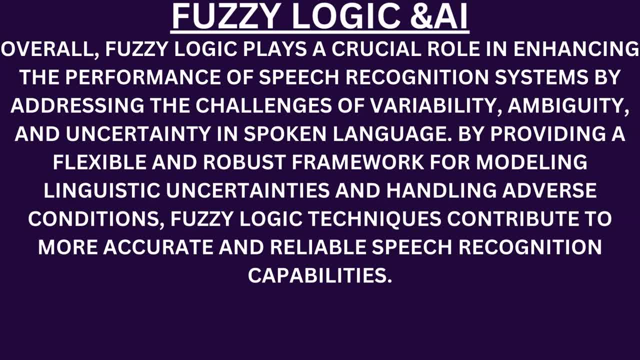 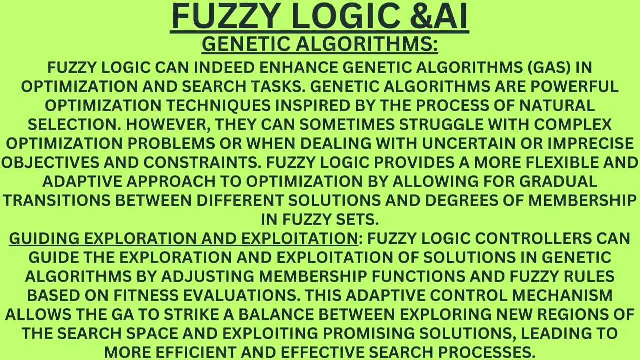 by providing a flexible and robust framework for modeling linguistic uncertainties and handling adverse conditions, Fuzzy logic techniques contribute to more accurate and reliable speech recognition capabilities. Genetic Algorithms- Fuzzy logic- can indeed enhance genetic algorithms in optimization and search tasks. Genetic algorithms are powerful optimization techniques inspired by the process of natural. 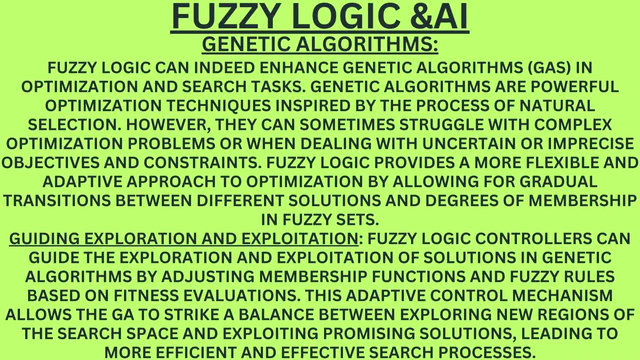 selection. However, they can sometimes struggle with complex options. Fuzzy logic provides a more flexible and adaptive approach to optimization by allowing for gradual transitions between different solutions and degrees of membership in fuzzy sets. Guiding Exploration and Exploitation: Fuzzy logic controllers can guide the exploration. 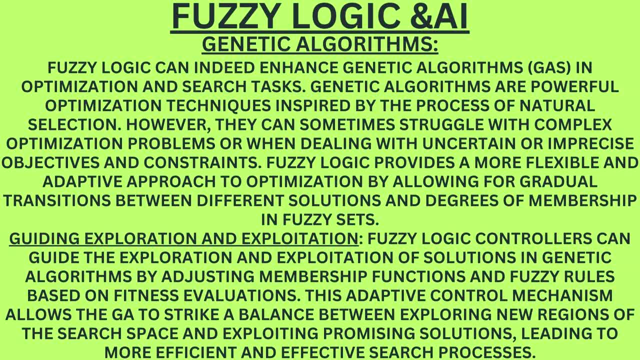 and exploitation of solutions in genetic algorithms. Genetic Algorithms, Fuzzy logic can be used by adjusting membership functions and fuzzy rules based on fitness evaluations. This adaptive control mechanism allows the genetic algorithm to strike a balance between exploring new regions of the search space and exploiting promising solutions leading 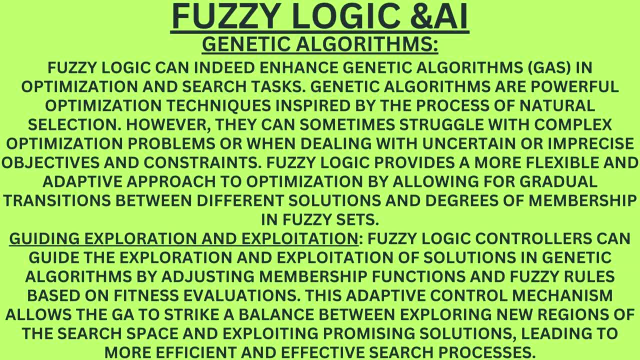 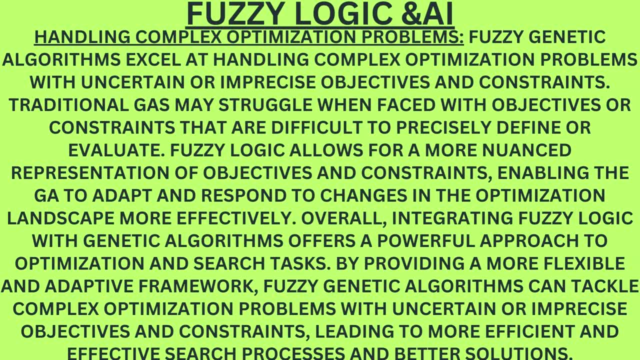 to more efficient and effective search processes. Handling Complex Optimization Problems. Handling Complex Optimization Problems: Fuzzy genetic algorithms excel at handling complex optimization problems with uncertain or imprecise objectives and constraints. Traditional GAS may struggle when faced with objectives or constraints that are difficult to precisely define or evaluate. 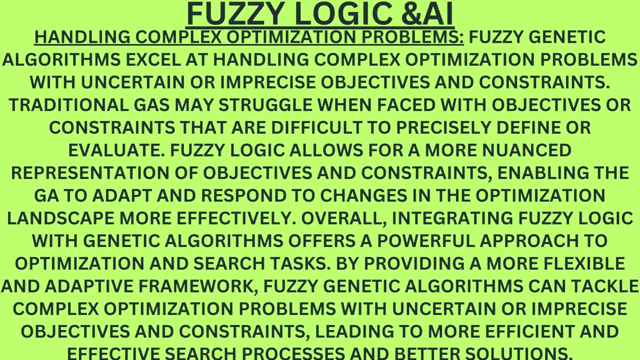 Fuzzy logic allows for a more nuanced representation of objectives and constraints, enabling the GAS to adapt. Fuzzy logic allows for a more nuanced representation of objectives and constraints, enabling the GAS to adapt and respond to changes in the optimization landscape more effectively. Overall, integrating fuzzy logic with genetic algorithms offers a powerful approach to optimization. 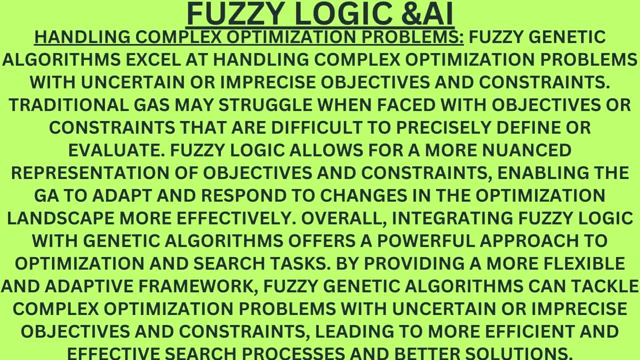 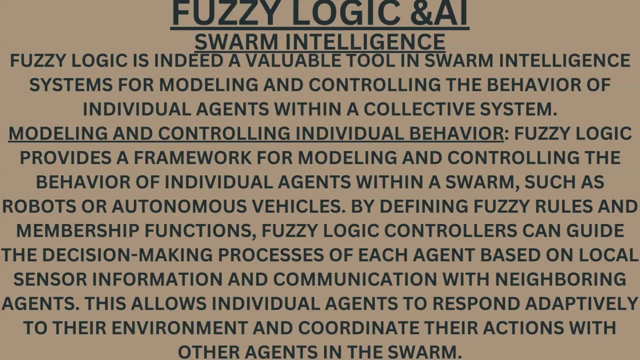 and search tasks. By providing a more flexible and adaptive framework. fuzzy genetic algorithms can tackle complex optimization problems with uncertain or imprecise objectives and constraints, leading to more efficient and effective search processes. Swarm Intelligence: Fuzzy logic is indeed a valuable tool in swarm. 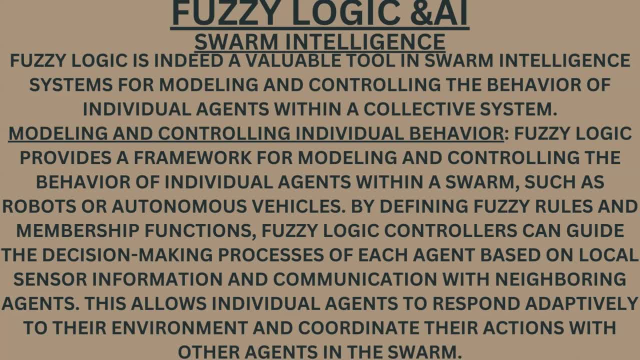 intelligence systems for modeling and controlling the behavior of individual agents within a collective system. Modeling and Controlling Individual Behavior: Fuzzy logic provides a framework for modeling and controlling the behavior of individual agents within a swarm, such as robots or autonomous vehicles. By defining fuzzy rules and membership functions, fuzzy logic controllers can guide the decision-making. 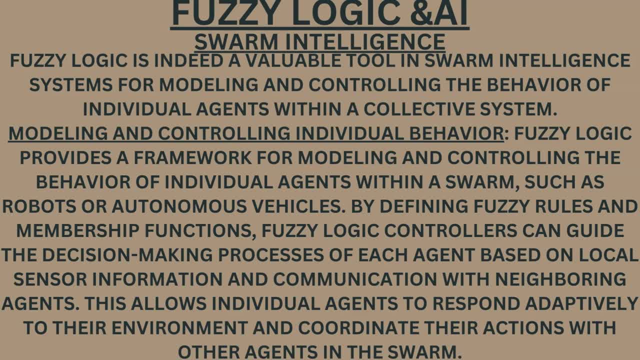 processes of each agent based on local sensor information and communication with neighboring agents. This allows individual agents to respond adaptively to their environment and coordinate their actions with other agents in the swarm. Guiding, Decision-Making and Coordination. Guiding, decision-making and coordination- fuzzy. 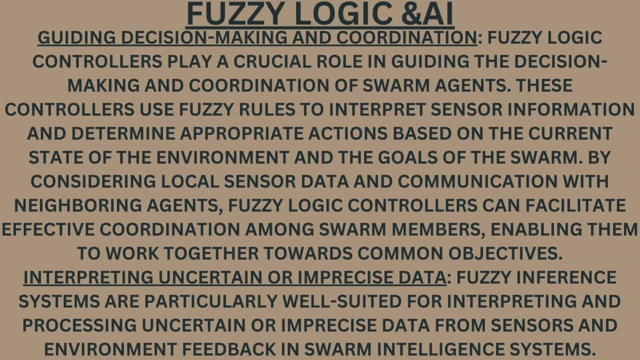 logic controllers play a crucial role in determining the behavior of individual agents within a swarm. By defining fuzzy rules and membership functions, fuzzy logic controllers can guide the decision-making processes of each agent based on local sensor information and communication with neighboring agents. These controllers use fuzzy rules to interpret sensor information and determine appropriate 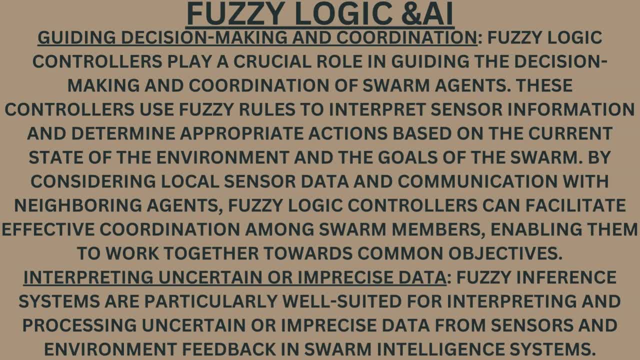 actions based on the current state of the environment and the goals of the swarm, By considering local sensor data and communication with neighboring agents. fuzzy logic controllers can facilitate effective coordination among swarm members, enabling them to work to control common objectives, Interpreting Uncertain or imprecise data. 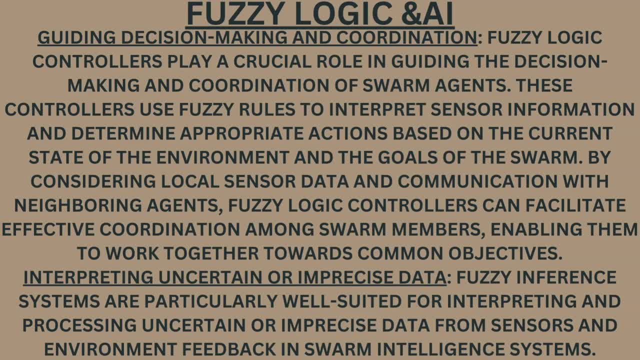 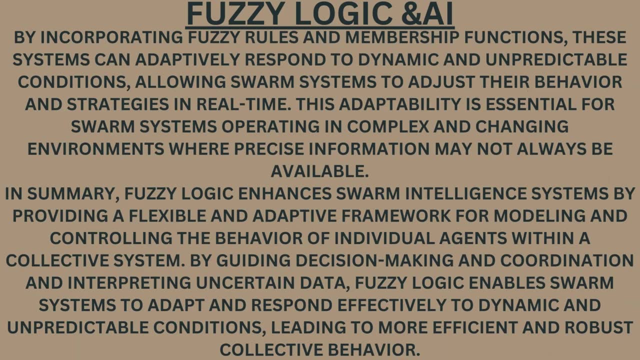 Fuzzy inference systems are particularly well-suited for interpreting and processing uncertain or imprecise data from sensors and environment feedback in swarm intelligence systems. By incorporating fuzzy rules and membership functions, these systems can adaptively respond to dynamic and unpredictable data. By incorporating fuzzy rules and membership functions, these systems can adaptively respond to dynamic and unpredictable data. 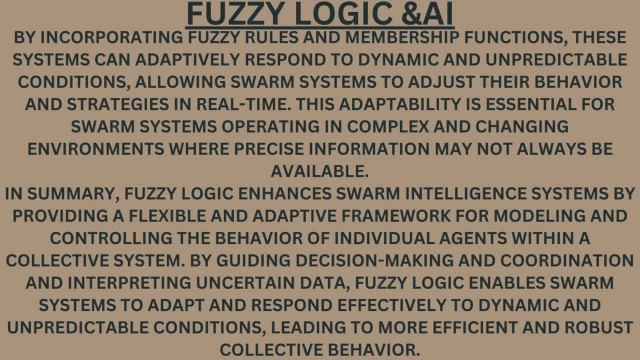 By turning its Cubist to the good side. search and control the exact sense of zurk�'s becue의. ff 2022 deadline: fuel hours, sauna weather time, content conditions, rate, volume, dostęp hours, supply time time time, location, position, content date, type date. 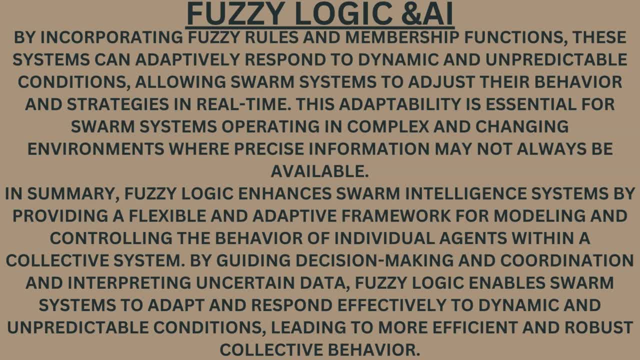 hand time time date down monthly of individual agents within a collective system. by guiding decision-making and coordination and interpreting uncertain data, fuzzy logic enables swarm systems to adapt and respond effectively to dynamic and unpredictable conditions, leading to more efficient and robust collective behavior. transfer learning- fuzzy logic indeed plays a crucial role in facilitating transfer learning by 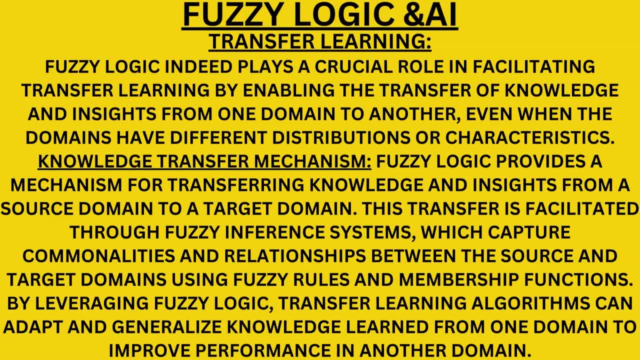 enabling the transfer of knowledge and insights from one domain to another, even when the domains have different distributions or characteristics. knowledge transfer mechanisms. fuzzy logic provides a mechanism for transferring knowledge and insights from a source domain to a target domain. this transfer is facilitated through fuzzy inference systems, which capture 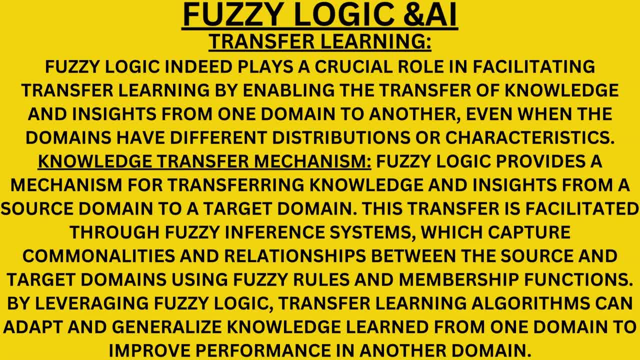 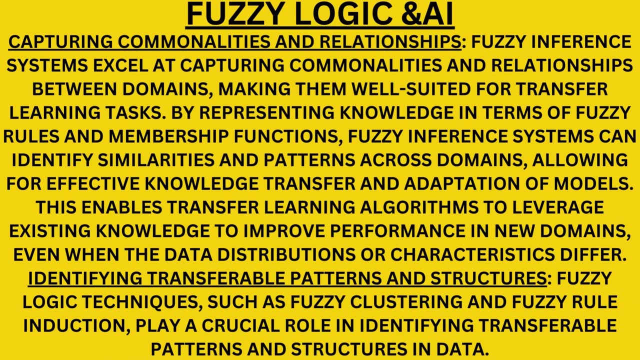 commonalities and relationships between the source and target domains using fuzzy rules and membership functions. By leveraging fuzzy logic, transfer learning algorithms can adapt and generalize knowledge learned from one domain to improve performance in another domain, Capturing Communalities and Relationships. Fuzzy inference systems excel at capturing commonalities and relationships between domains. 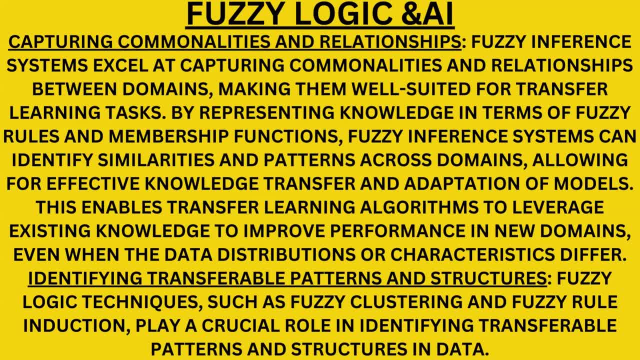 making them well-suited for transfer learning tasks By representing knowledge in terms of fuzzy rules and membership functions, fuzzy inference systems can identify similarities and patterns across domains, allowing for effective knowledge transfer and adaptation of models. This enables transfer learning algorithms to leverage existing knowledge to improve performance in new domains. 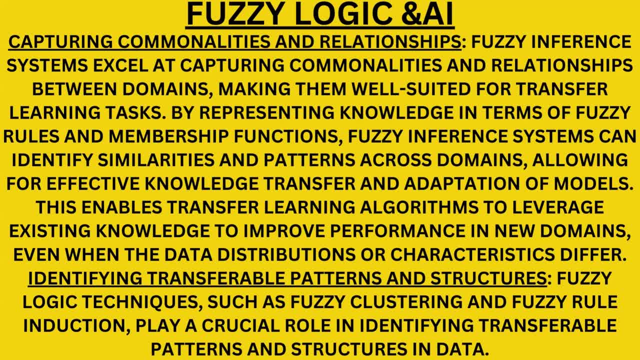 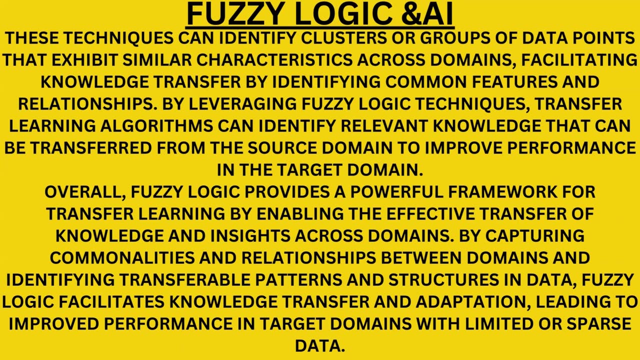 even when the data distributions of the domain are different. Fuzzy logic techniques such as fuzzy clustering and fuzzy rule induction play a crucial role in identifying transferable patterns and structures in data. These techniques can identify clusters or groups of data points that exhibit 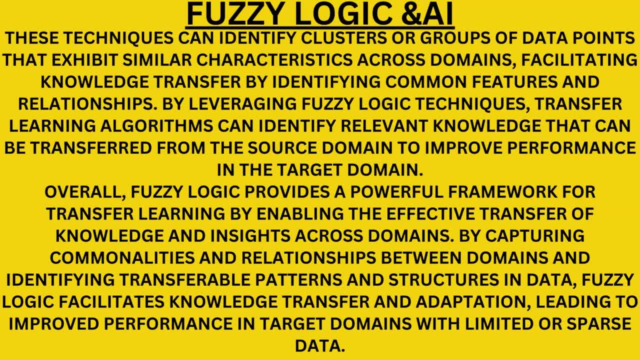 similar characteristics across domains, facilitating knowledge transfer by identifying common features and relationships. By leveraging fuzzy logic techniques, transfer learning algorithms can identify relevant knowledge that can be transferred from the source domain to improve performance in the target domain. Overall, fuzzy logic provides a powerful framework for transfer. 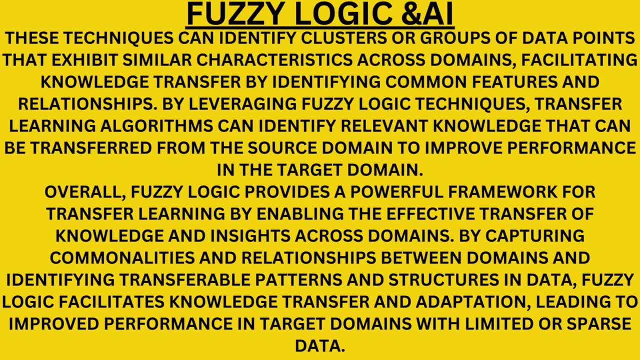 learning by enabling the effective transfer of knowledge and insights across domains. By capturing commonalities and relationships between domains and identifying transferable patterns and structures in data, fuzzy logic facilitates knowledge transfer and adaptation, leading to improved performance in target domains with limited or sparse data. 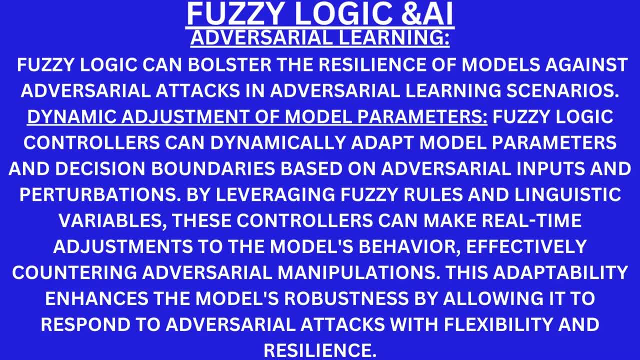 Adversarial Learning: Fuzzy logic can bolster the resilience of models against adversarial attacks in adversarial learning scenarios. Dynamic Adjustments of Model Parameters: Fuzzy logic controllers can dynamically adapt model parameters and decision boundaries based on adversarial inputs and perturbations. 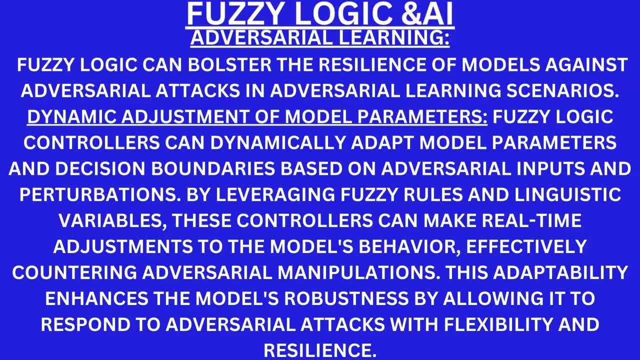 By leveraging fuzzy rules and linguistic variables, these controllers can make real-time adjustments to the model's behavior, effectively countering adversarial manipulations. This adaptability enhances the model's robustness by allowing it to respond to adversarial attacks with flexibility and resilience. 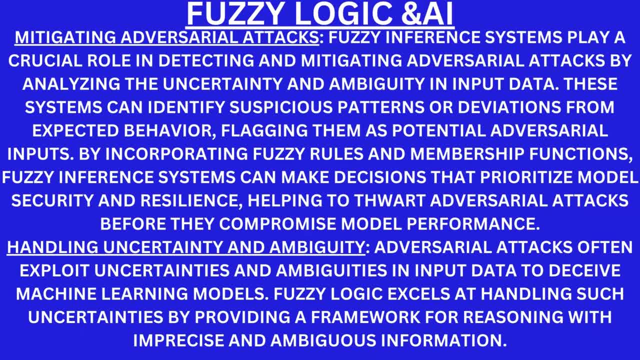 Mitigating Adversarial Attacks. Fuzzy inference systems play a crucial role in detecting and mitigating adversarial attacks. by analyzing the uncertainty and ambiguity in input data, These systems can identify suspicious patterns or deviations from expected behavior, flagging them as potential adversarial inputs. 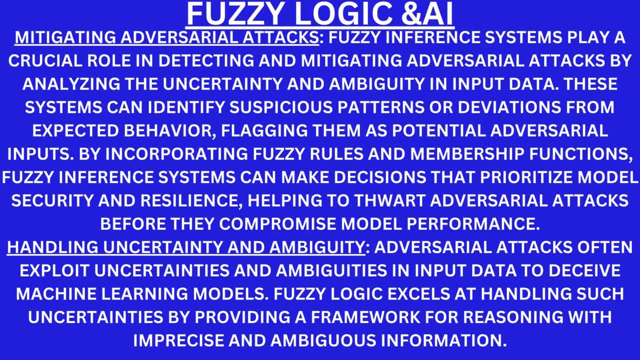 By incorporating fuzzy rules and membership functions, fuzzy inference systems can make decisions that prioritize model security and resilience, helping to ward adversarial attacks before they compromise model performance. Handling Uncertainty and Ambiguity: Adversarial attacks often exploit uncertainties and ambiguities in input data to deceive. 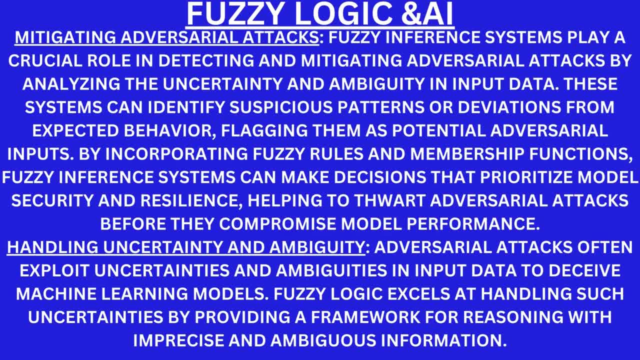 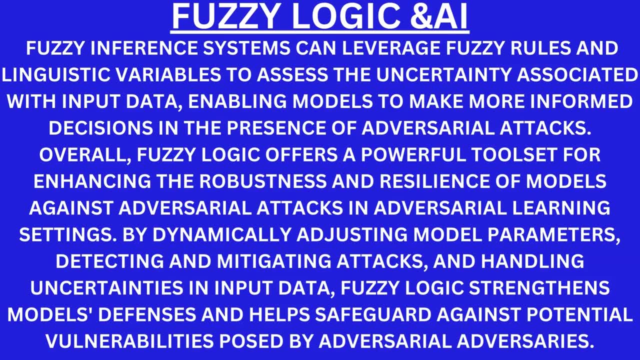 machine learning models. Fuzzy logic excels at handling such uncertainties by providing a framework for reasoning with imprecise and ambiguous information. Fuzzy inference systems can leverage fuzzy rules and linguistic variables to assess the uncertainty associated with input data, enabling models to make more informed decisions in the 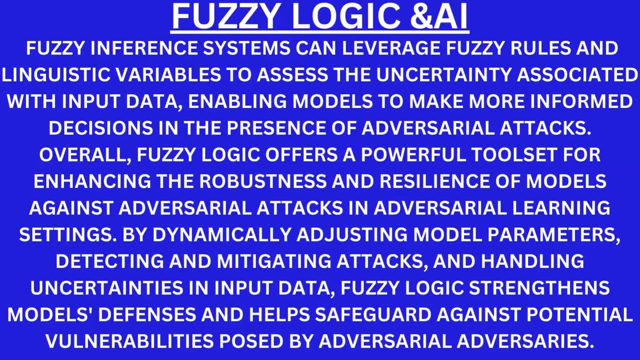 presence of adversarial attacks. Overall, Fuzzy logic offers a powerful toolset for enhancing the robustness and resilience of models against adversarial attacks in adversarial learning settings by dynamically adjusting model parameters, detecting and mitigating attacks and handling uncertainties in input data. 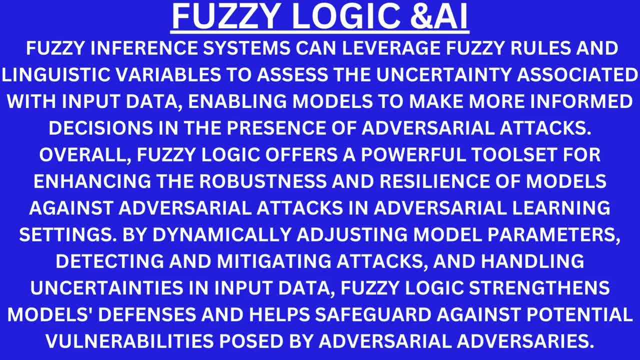 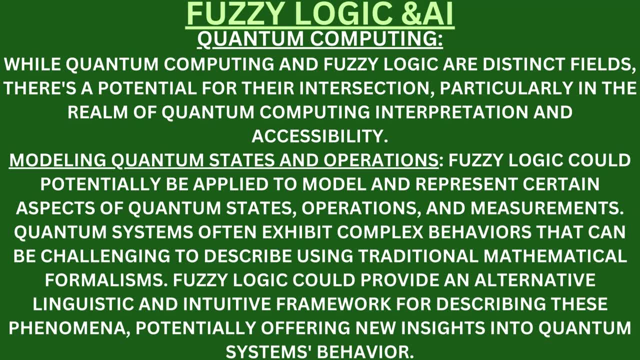 Fuzzy logic strengthens models' defenses and helps safeguard against potential vulnerabilities posed by adversarial attacks. Quantum Computing: While quantum computing and fuzzy logic are distinct fields, there is a potential for their intersection, particularly in the realm of quantum computing, interaction and accessibility. Modeling, Quantum States and Operations. 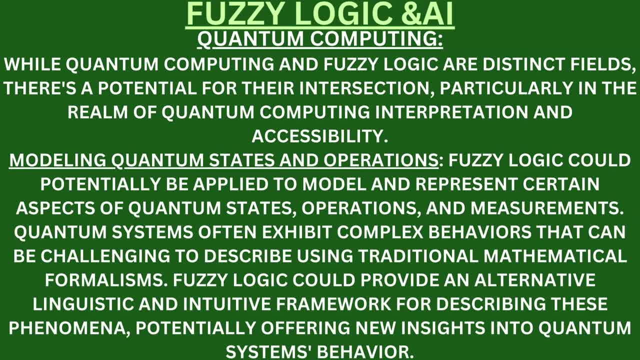 Fuzzy logic could potentially be applied to model and represent certain aspects of quantum states, operations and measurements. Quantum systems often have complex behaviors that can be challenging to describe using traditional mathematical formalisms. Fuzzy logic could provide an alternative linguistic and intuitive framework for describing these phenomena, potentially offering new insights into quantum. 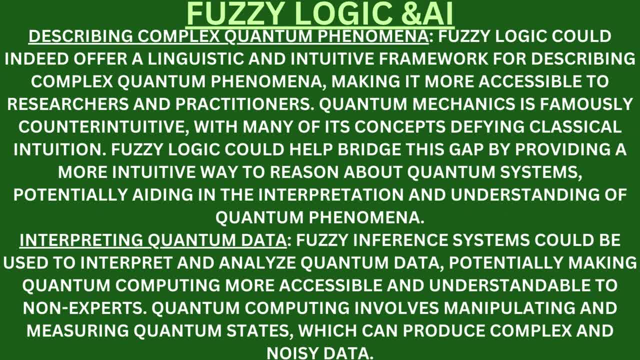 systems' behavior. Describing Complex Quantum Phenomena. Fuzzy logic could indeed offer a linguistic and intuitive framework for describing complex quantum phenomena, making it more accessible to researchers and practitioners. Quantum mechanics is famously counterintuitive, with many of its concepts defying classical. 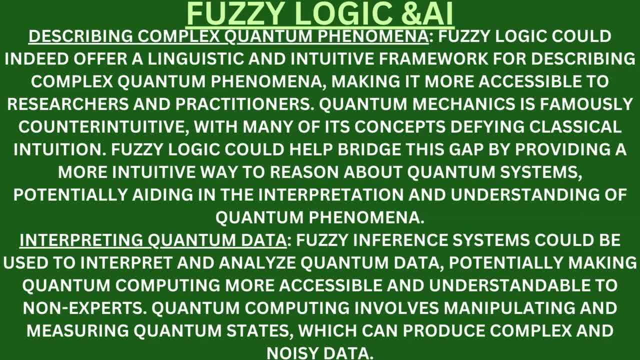 intuition. Fuzzy logic could help bridge this gap by providing a more intuitive way to reason about quantum systems, potentially aiding in the interpretation and understanding of quantum phenomena. Interpretation and Understanding of Quantum Phenomena. Interpreting quantum data: Fuzzy inference systems could be used to interpret and analyze quantum data. 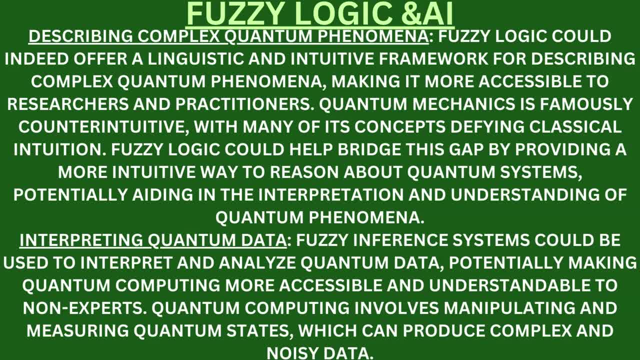 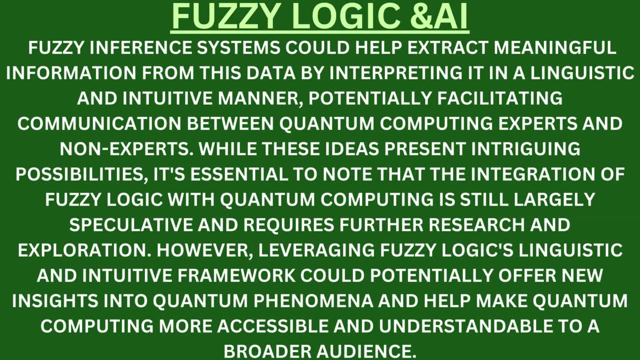 potentially making quantum computing more accessible and understandable to non-experts. Quantum computing involves manipulating and mirroring quantum states, which can produce complex and noisy data. Fuzzy inference systems could help extract meaningful information from this data by interpreting complex and noisy data. Fuzzy inference systems could help extract meaningful 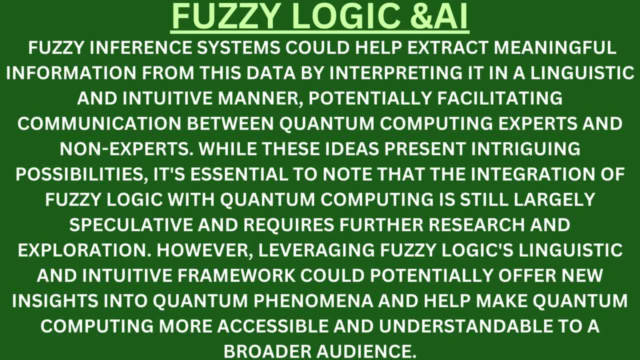 information by integrating complex and noisy data that might allow later, Elsa Fon, An overcoating sense of balance could help fuzzing fuzziness, and fuzzing fuzziness depending on the kind of plausible reason that problem arises, since quantum & quantum compute are closely linked towards match-and- análise in quantum information order learning random. 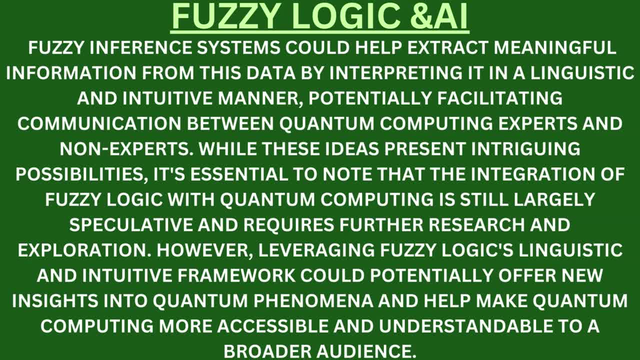 patterns of power and Piecework. Futurist power Tением theory is a Star Spirit, that is, a married engineer who needs answers to this ancient, competent Beta Mazisci for first-hand schizophrenia-based performanceuge of çi nagip at mantra qn q Ingredients. 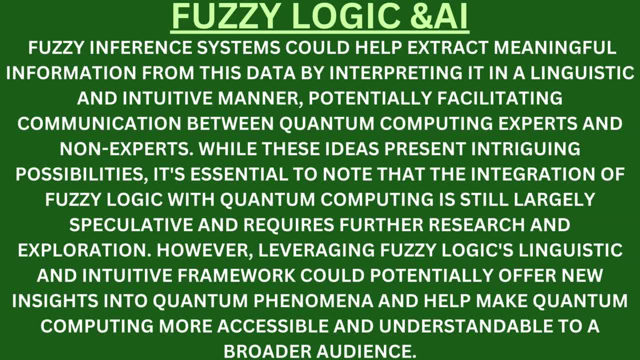 • Not all quantum technologies are qualified forquentI methodologies to handle quantum mechanics Change from application and application сх of pressed-to�� to naturalization process들. • Not all quantum countries are capable of진 function of抰 γν fitting theression farm. stata x 도 t° nə english equation. 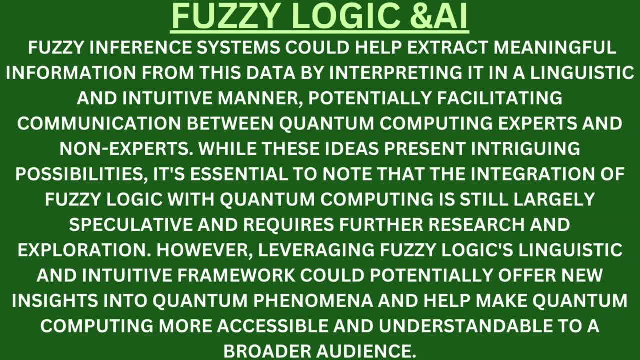 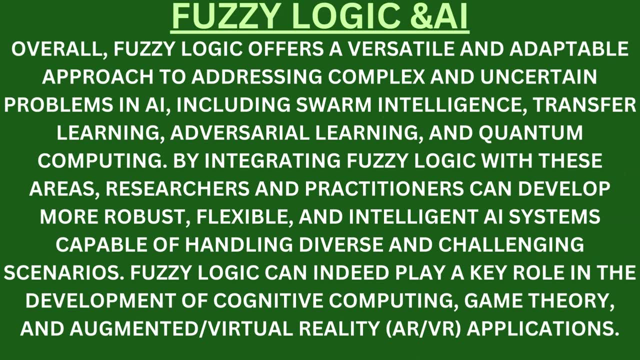 intuitive framework could potentially offer new insights into quantum phenomena and help make quantum computing more accessible and understandable to a broader audience. Overall, Fuzzy Logic offers a versatile and adaptable approach to addressing complex and uncertain problems in artificial intelligence, including swarm intelligence transfer learning. 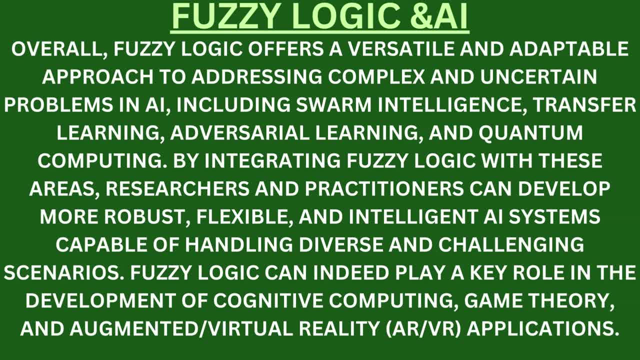 adversarial learning and quantum computing. By integrating Fuzzy Logic with these areas, researchers and practitioners can develop more robust, flexible and intelligent artificial intelligence systems capable of handling diverse and challenging scenarios. Fuzzy Logic can indeed play a key role in the development of cognitive computing, game theory and augmented 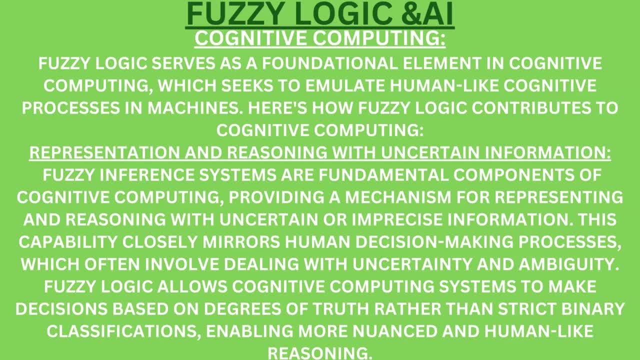 virtual reality applications. Cognitive Computing is a new technology that is being developed in the field of artificial intelligence. Fuzzy Logic serves as a foundational element in cognitive computing, which seeks to emulate human-like cognitive processes in machines: Representation and Reasoning with Uncertain Information. 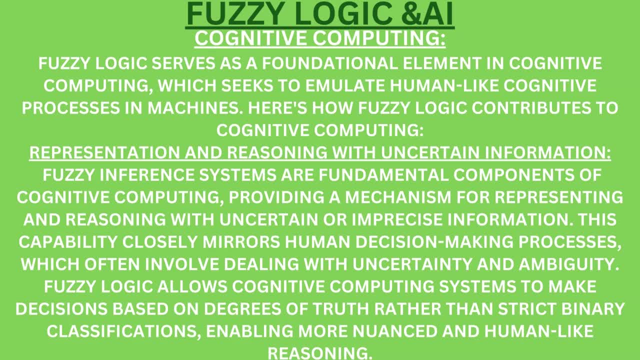 Fuzzy inference systems are fundamental components of cognitive computing, providing a mechanism for representing and reasoning with uncertain or imprecise information. This capability closely mirrors human decision-making processes, which often involve dealing with uncertainty and ambiguity. Fuzzy Logic allows cognitive computing systems to make decisions. 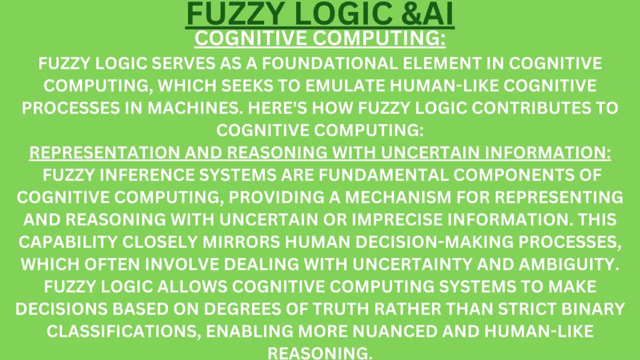 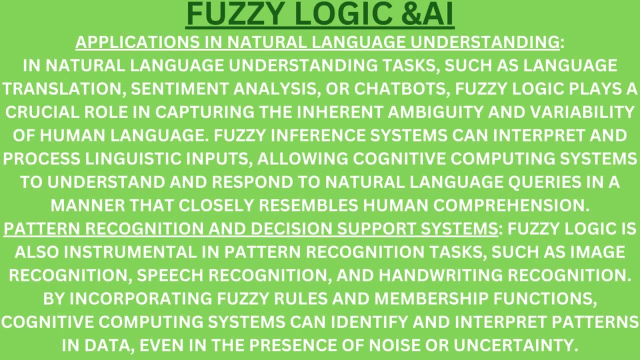 based on degrees of truth rather than strict binary classifications, enabling more nuanced and human-like reasoning. Applications in Natural Language, Understanding In natural language, understanding tasks such as language translation, language processing, language processing and language processing, language translation, sentiment analysis or chatbots. fuzzy logic plays a crucial role in capturing. 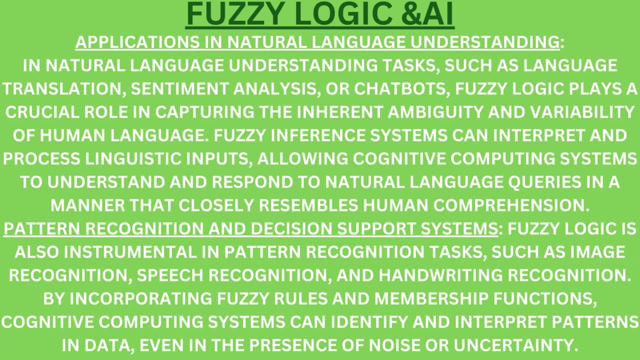 the inherent ambiguity and variability of human language. Fuzzy inference systems can interpret and process linguistic inputs, allowing cognitive computing systems to understand and respond to natural language queries in a manner that closely resembles human comprehension. Fuzzy logic is also instrumental in pattern recognition tasks such as image recognition. 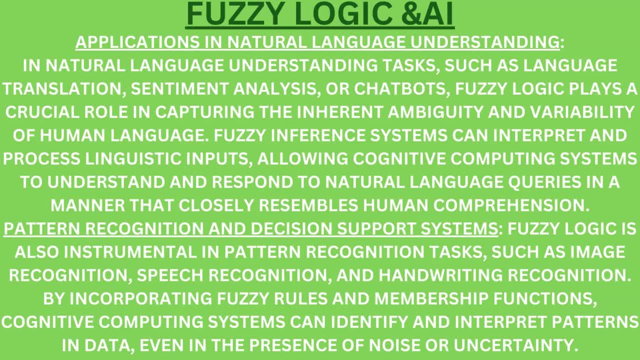 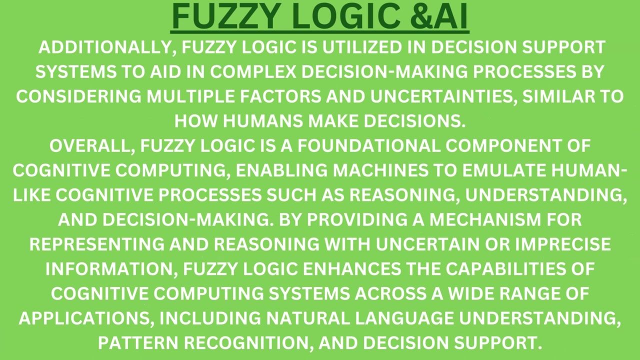 speech recognition and handwriting recognition. By incorporating fuzzy rules and membership functions, cognitive computing systems can identify and interpret patterns in data even in the presence of noise or uncertainty. Fuzzy logic is utilized in decision support systems to aid in complex decision-making processes by considering multiple factors and uncertainties, similar to how humans make 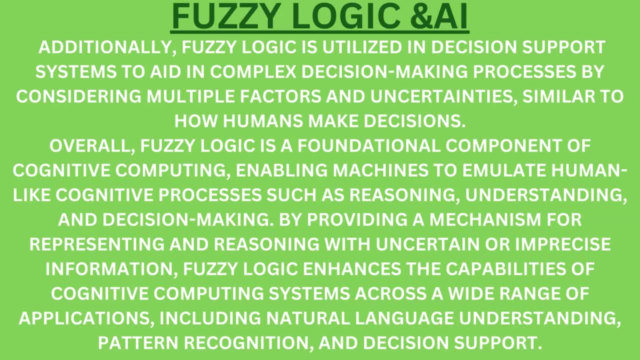 decisions Overall. fuzzy logic is a foundational component of cognitive computing, enabling machines to emulate human-like cognitive processes such as reasoning, understanding and decision-making. by providing a mechanism for decision-making, For representing and reasoning with uncertain or imprecise information, fuzzy logic enhances 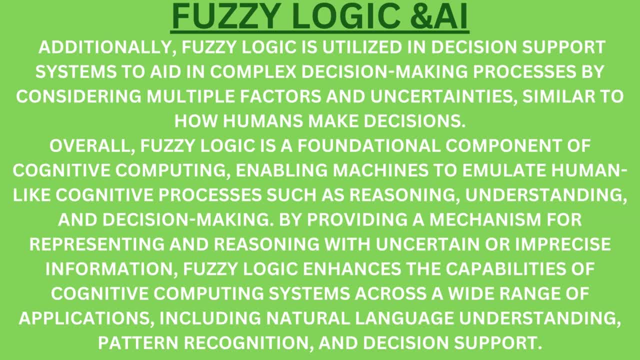 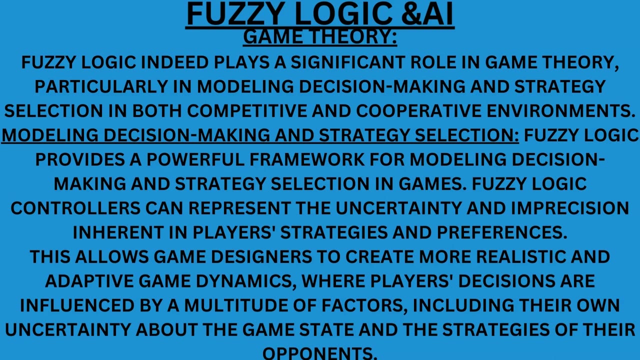 the capabilities of cognitive computing systems across a wide range of applications, including natural language understanding, pattern recognition and decision support. Game Theory: Fuzzy logic indeed plays a significant role in game theory, particularly in modeling, decision-making and strategy selection in both competitive and 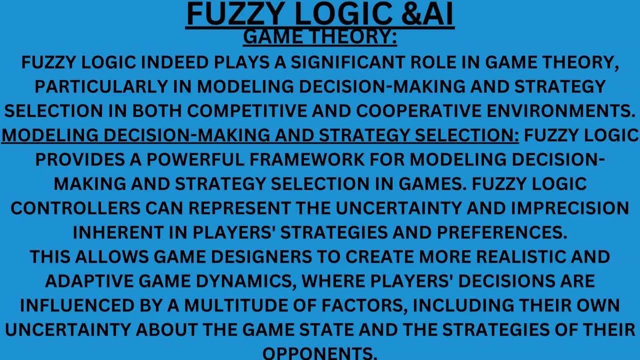 cooperative issues. The game theory plays an essential role in the development of games, residential and business-based systems, and Google's game theory is an important component of financial environments modeling, decision making and strategy selection. fuzzy logic provides a powerful framework for modeling, decision making and strategy selection in games. fuzzy logic controllers. 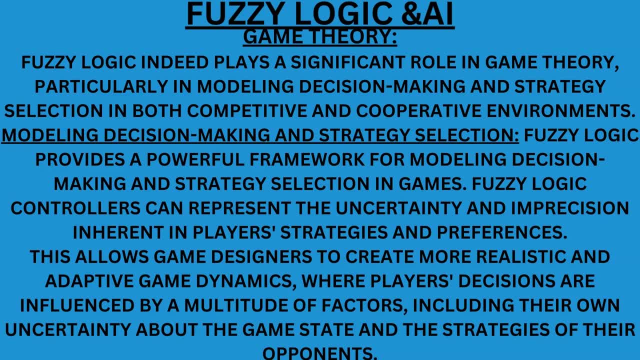 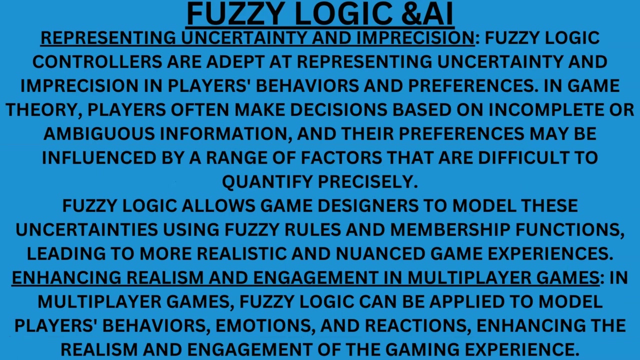 can represent the uncertainty and impression inherent in players strategies and preferences. this allows game designers to create more realistic and adaptive game dynamics where players decisions are influenced by a multitude of factors, including their own certainty about the game state and the strategies of their opponents. representing uncertainty and impression. 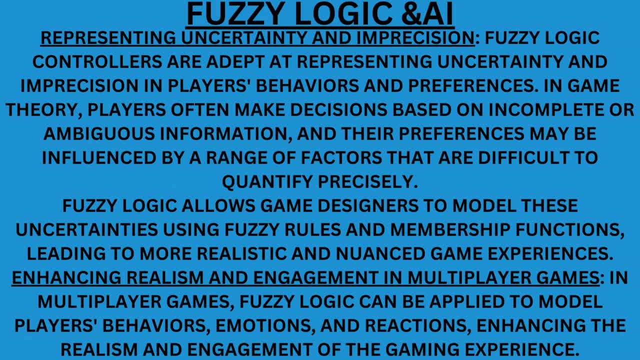 fuzzy logic controllers are adept at representing uncertainty and impression in players behaviors and preferences. in game theory, players often make decisions based on incomplete or ambiguous conditions in game, recklessly matching attitude, situations orーpreferences. fuzzie logic allows game designers model these uncertainties using fuzzy rules and membership. 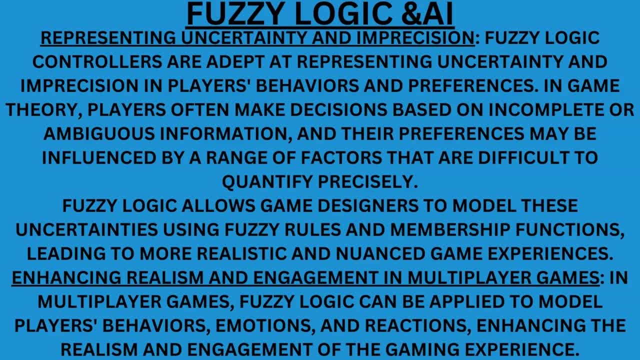 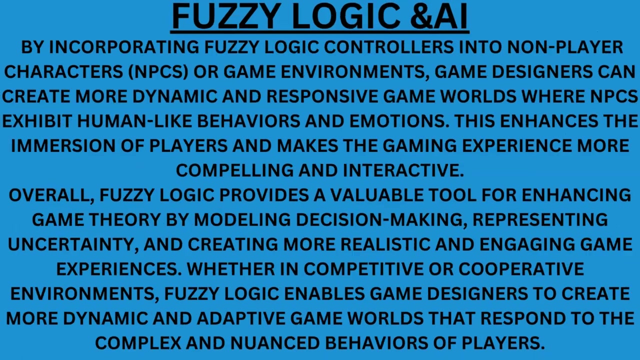 functions leading to philosophy. realistic and nuanced game experiences. enhancing realism and engagement in multiplayer games. scales in multiplayer games: fozzie logic can be applied to model players behaviors, emotions and reactions. enhancing the realism and engagement of the gaming experience by incorporating fuzzy logic controllers into non-player characters. 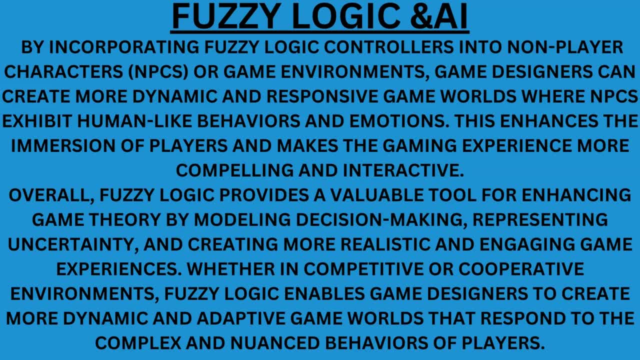 npcs or game environments. game designers can create more dynamic and responsive game world where npcs exhibit human-like behaviors and emotions. this enhances the immense immersion of players and make the gaming experience more compelling and interactive. overall, fuzzy logic provides a valuable tool for enhancing game theory by modeling decision making representing 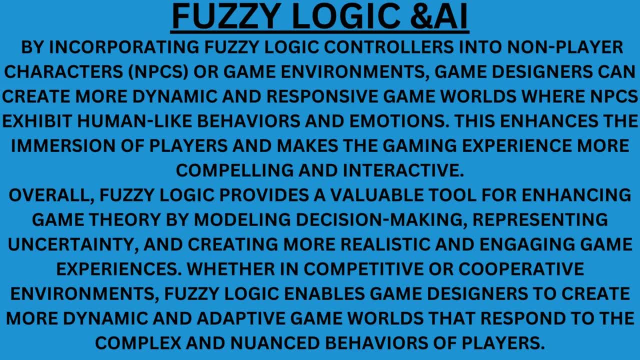 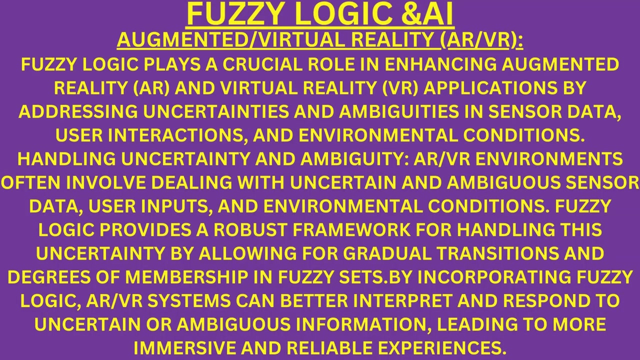 uncertainty and creating more realistic and engaging game experiences, whether in competitive or cooperative environments. fuzzy logic enables game designers to create more dynamic and adaptive game worlds that respond to the complex and nuanced behaviors of players. augmented virtual reality- ar, vr. fuzzy logic plays a crucial role in enhancing augmented reality, ar and virtual 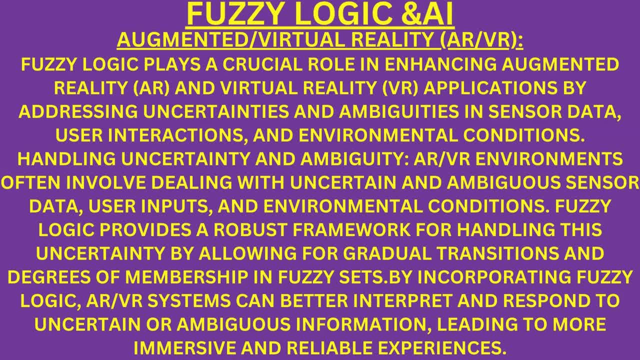 reality vr applications by addressing uncertainties and ambiguities in sensor data, user interactions and environmental conditions. handling uncertainty and ambiguity- ar vr environments often involve dealing with uncertain and ambiguous sensor data, user inputs and environmental conditions. fuzzy logic provides a robust framework for handling the uncertainty by allowing for. 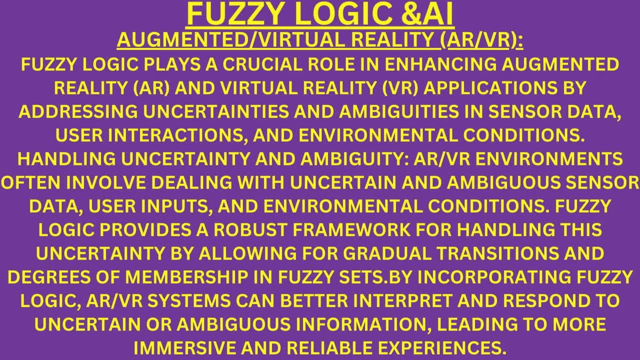 gradual transitions and degrees of membership in fuzzy sets by incorporating fuzzy logic, ar, vr and virtual reality vr applications. by incorporating fuzzy logic, ar and virtual reality vr applications, by enhancing augmented reality and environmental conditions, ar vr systems can better interpret and respond to uncertain or ambiguous information, leading to more. 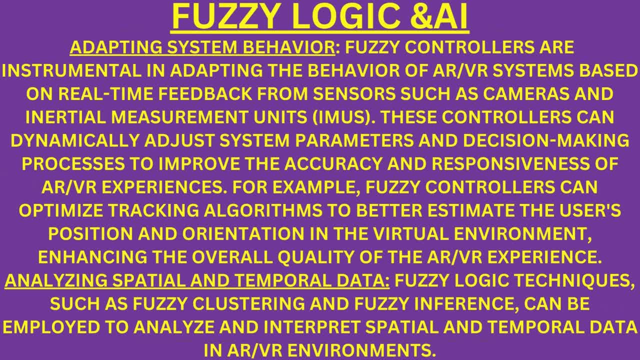 immersive and reliable experiences. adapting system behavior: fuzzy controllers are instrumental in adapting the behavior of ar vr system based on real-time feedback from sensors such as cameras and inertial measurement units imus. these controllers can dynamically adjust system parameters and decision making processes to improve the accuracy and 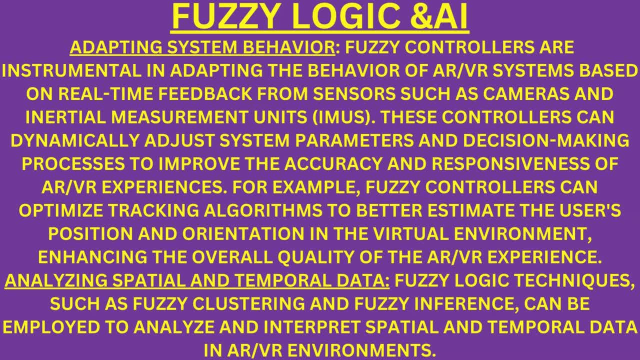 responsiveness of ar vr experiences. for example, fuzzy controllers can optimize tracking algorithms to better estimate the user's positions and orientation in the virtual environment, enhancing the overall quality of the ar vr experience. analyzing special and temporal data, fuzzy logic techniques such as fuzzy clustering and fuzzy inference can be employed to analyze and 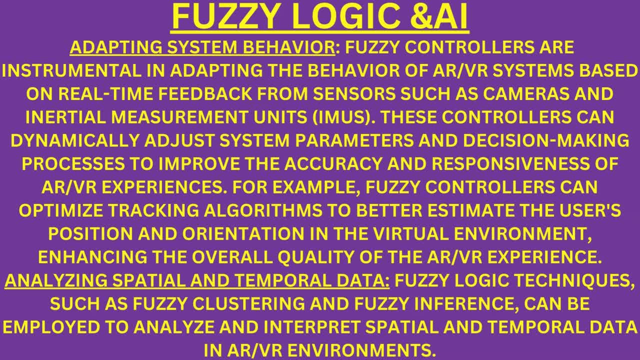 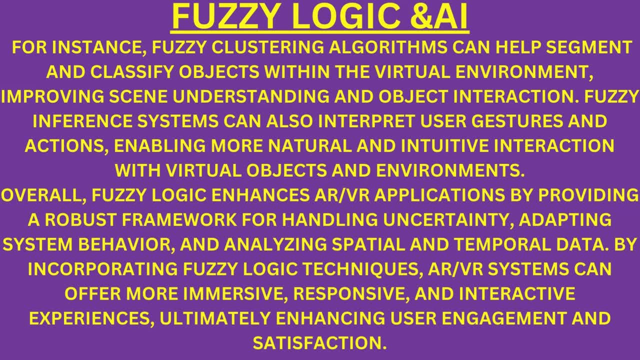 interpret special and temporal data in ar vr environments. for instance, fuzzy clustering algorithms can help segment and classify objects within the virtual environment, improving scene understanding and object interaction. fuzzy inference systems can also interpret user gestures and actions, enabling more natural and intuitive interaction with virtual objects and environments. 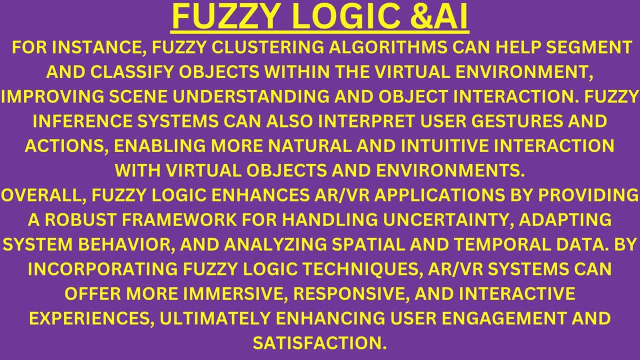 overall. fuzzy logic enhances ar vr applications by providing a robust framework for handling uncertainty, adapting system behavior and analyzing special and temporal data. by incorporating fuzzy logic techniques, ar vr systems can offer more immersive, responsive and interactive experiences, ultimately enhancing virtual and virtual reality vr applications, user engagement and satisfaction. fuzzy logic plays a crucial role in cognitive computing. 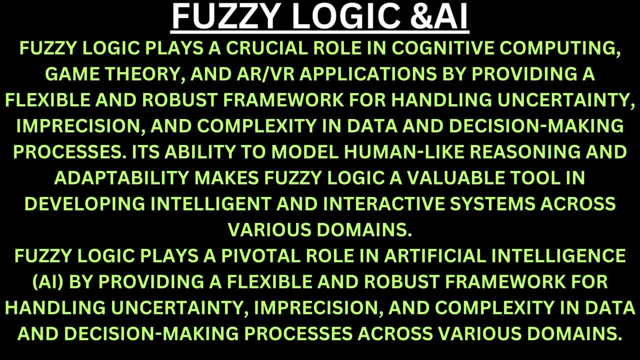 game theory and ar? vr applications, by providing a flexible and robust framework for handling uncertainty, impresion and complexity in data and decision making processes. its ability to model human-like reasoning and adaptability makes fuzzy logic a valuable tool in developing intelligent and interactive systems across a wide range of technologies and technologies and technologies. 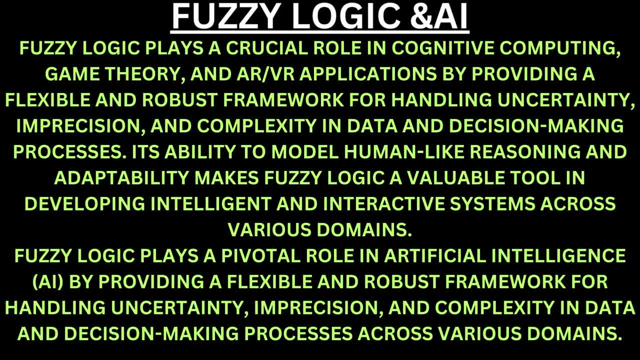 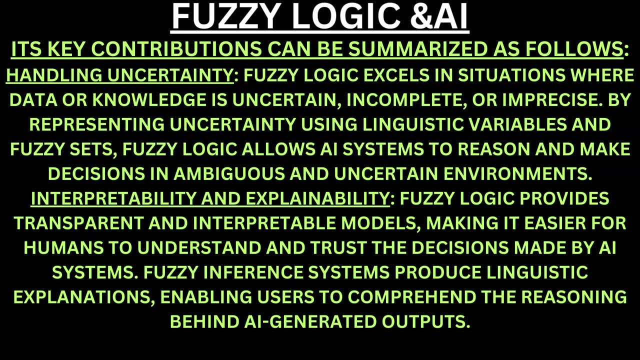 across various domains. fuzzy logic plays a pivotal role in artificial intelligence by providing a flexible and robust framework for handling uncertainty, impression and complexity in data and decision making processes across various domains. its key contributions can be summarized as follows: handling uncertainty: fuzzy logic excels in situations where data or knowledge is uncertain. 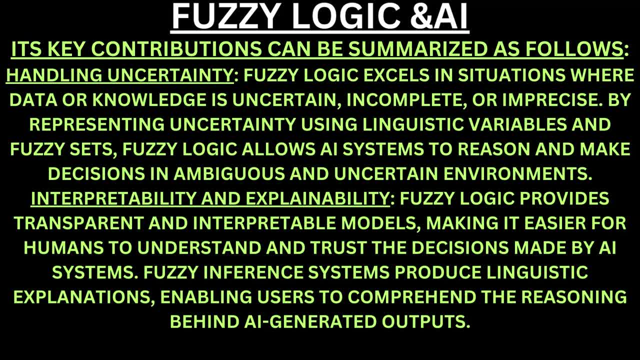 or imprecis by representing uncertainty using linguistic variables and fuzzy sets. fuzzy logic allows artificial intelligence systems to reason and make disseigns in ambiguous and uncertain environments. interpretability and explainability: fuzzy logic provides transparent and interpretable models, making it easier for humans to understand and trust the decisions made by. 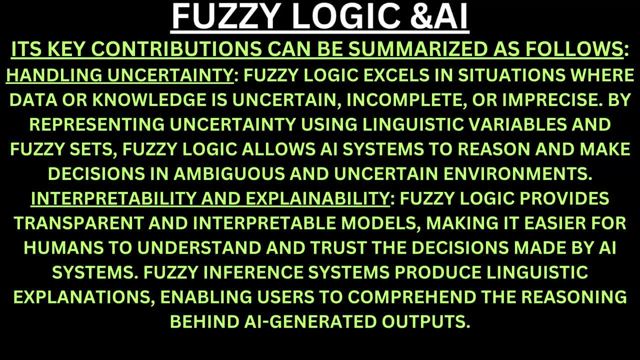 artificial intelligence systems. fuzzy slices are designed to mogąize the disclosure subuna and into questa. the policymakers may wonder: why is there a lack of understanding between Fashion Logistics and Tha grease perdu by artificial intelligence systems? fuzzy in systems produce linguistic explanations enabling users to comprehend the reasoning behind AI. 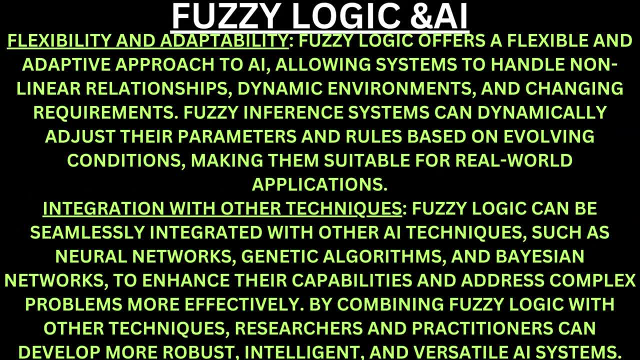 generated outputs. Flexibility and adaptability: Fuzzy logic offers a flexible and adaptive approach to artificial intelligence, allowing systems to handle non-linear relationships, dynamic environments and changing requirements. Fuzzy inference systems can dynamically adjust their parameters and rules based on evolving conditions, making them suitable for real-world.